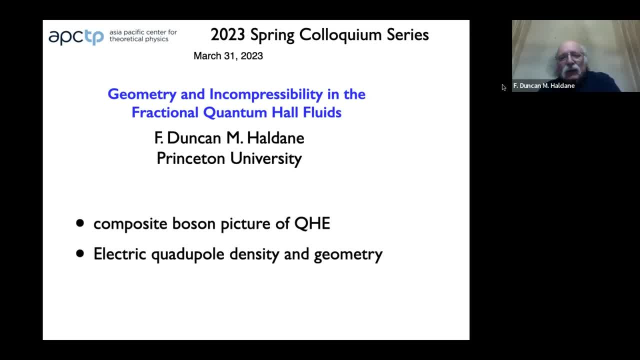 Okay, thank you. so, thank you for the invitation. give you my my, my, my viewpoint on the problems of the fractional quantum Hall effect and which, of course, is the the first, the most strongest of the topologically ordered states to have been discovered. 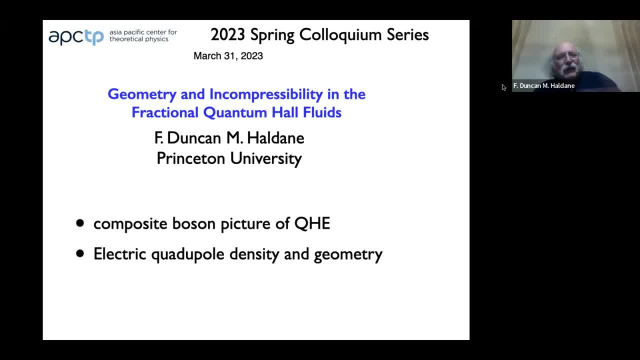 And now people are hoping to find generalized quantum Hall effect, find fractional churn insulators, do things in twisted bilayer graphene. so there's lots of new possibilities. But I'm going to basically give you my philosophy on the fractional Hall effect and tell you something about what I think is a new development that I have just made in this. 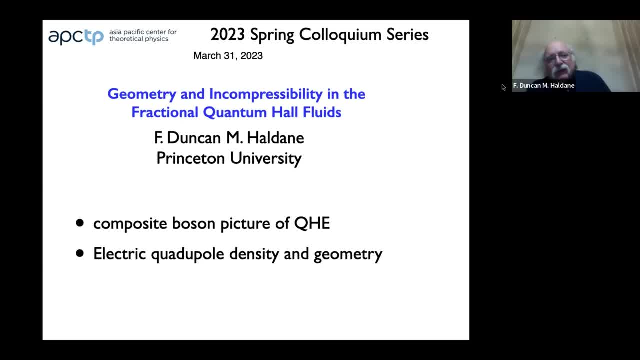 And the basic issue I think in all these topological states is Most of the work takes for granted. you've got a gap And then you have a state with some kind of no low lying expectations and you have topological states that you can- topological defects- you can move around and hopefully use for quantum computing and the most interesting states. 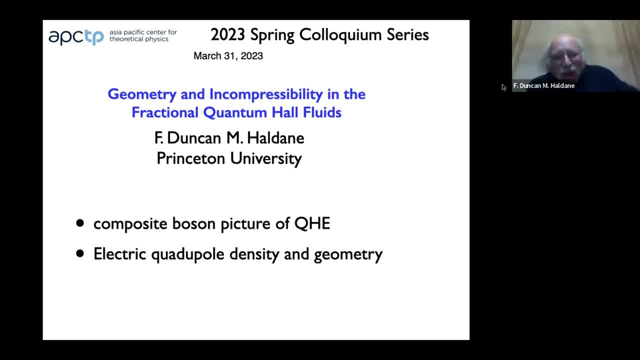 But to have these topological states you need to get the gap. And what's been, what hasn't been really properly addressed, I think, is what exactly is the mechanism, the energetic mechanism that gives rise, why? why a topological phases sometimes favored? 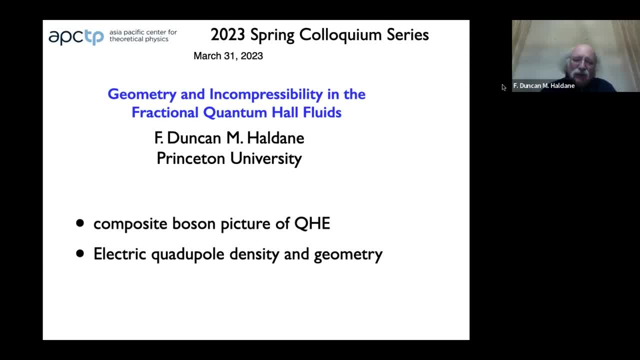 What is it? the favors and And if we can understand that better we can, that we maybe can work out how to build some of these more exotic states that that, on paper at least to show- we promise for things like Quantum computing and and topologically protected quantum computing. 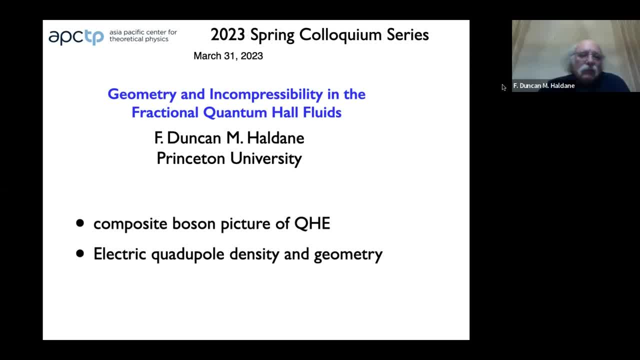 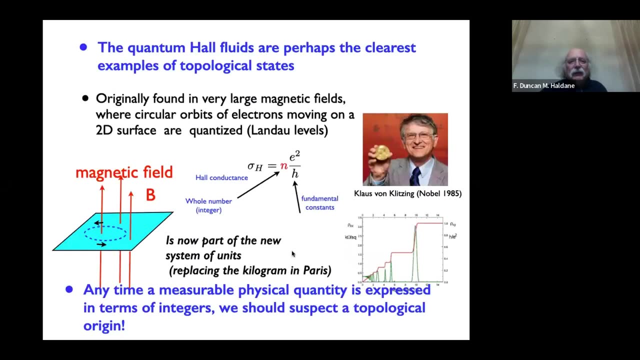 Okay, so I'm going to start off rather simply for a large amount of time. I hope it's not too simple, but people asked for- I was asked- to give some kind of overview for starting. So, okay, I'm gonna focus on the composite boson picture. 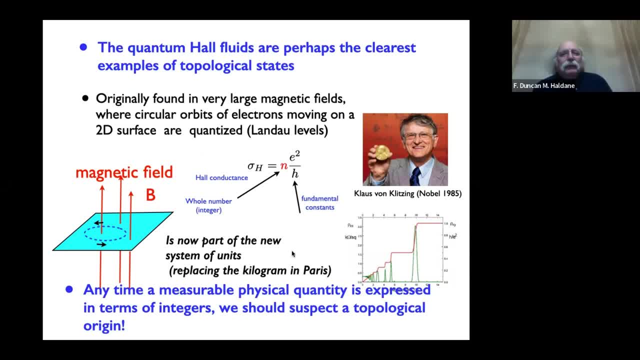 and I'll explain. it'll emerge widely as I go along. But again, let's start simply that quantum Hall states, quantum Hall fluids are perhaps the clearest examples of topological states And of course there's been a number of Nobel prizes. 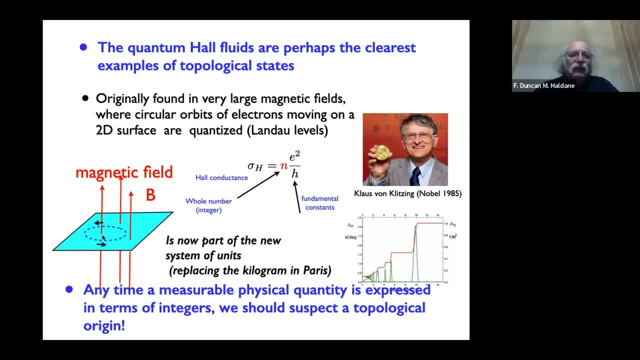 in this and the basic feature is that we have two-dimensional system. It's a very two-dimensional thing: Electrons confined to a lattice plane, basically either a lattice plane on a crystal or possibly a graphene sheet, And if you have a magnetic field, of course, 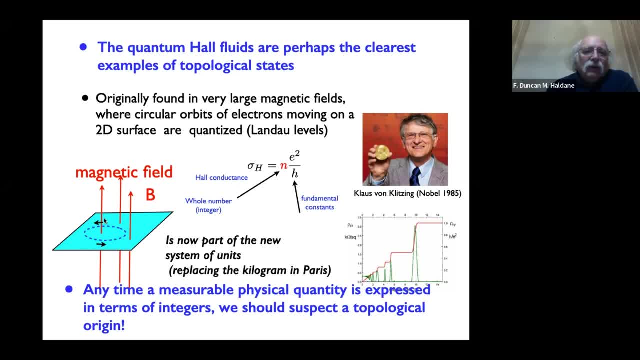 then the electrons in the magnetic field, through the plane. the electrons want to go in closed orbits, in around the field lines. And the crucial reason why do they wanna go in closed orbits? because they're moving along lines of. because they're moving along lines of. 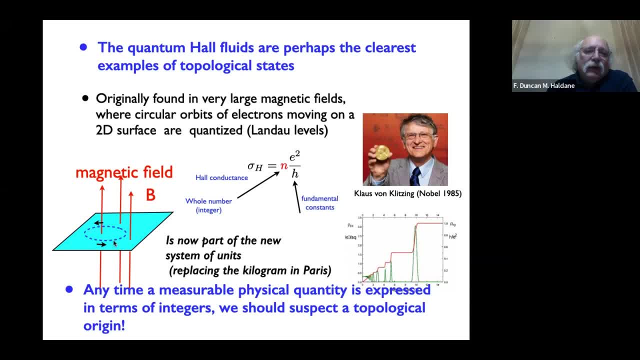 because they're moving along lines of constant energy in a block band structure that's living on this two-dimensional plane. So it's important there's actually a crystalline background, something which has block states. Most of the usual treatments, the simple treatments, will just assume. 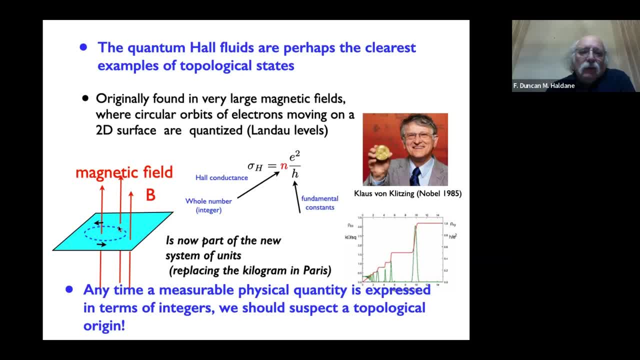 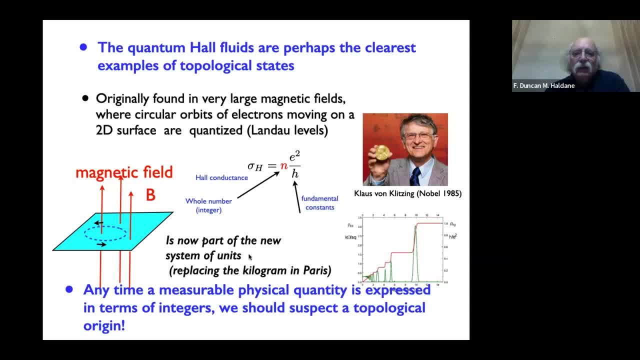 through which a magnetic field is passing. okay. So I mean, the crucial feature, of course, was that when the whole conductance is measured, it's integer, times, fundamental constants, And of course the famous measurements started off with Von Klitzing, and we see here: 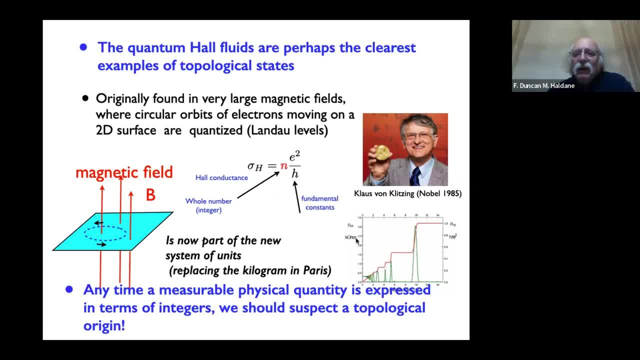 the experimental as a situation. If I measure the, the inverse of the conductivity, the resistivity as a function, the whole resistivity as a function of a magnetic fields, you get these nice plateaus at very highly quantized. And now this is part of the new system of units. 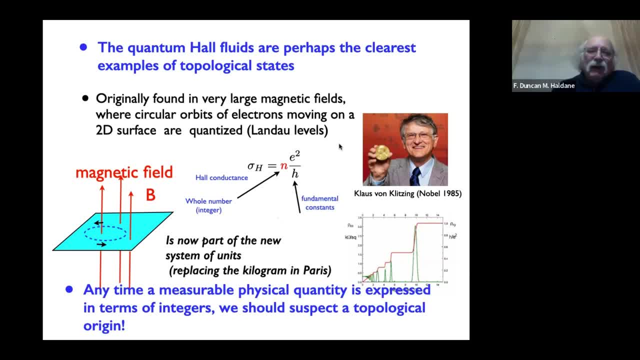 because it's allowed us to get rid of the kilogram. by combining this with the Josephson effect in superconductors, everyone can now build their own kibble balance, which allows you to check the market traders scales to make sure they're not cheating the customers. 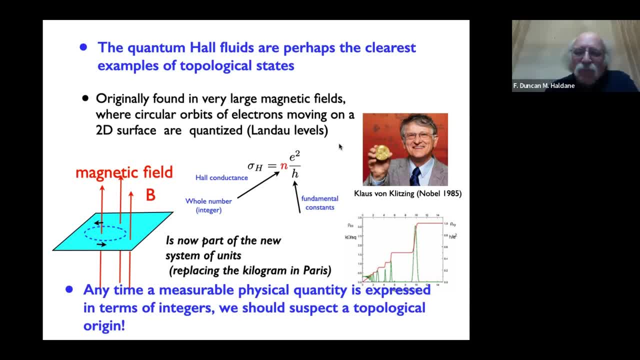 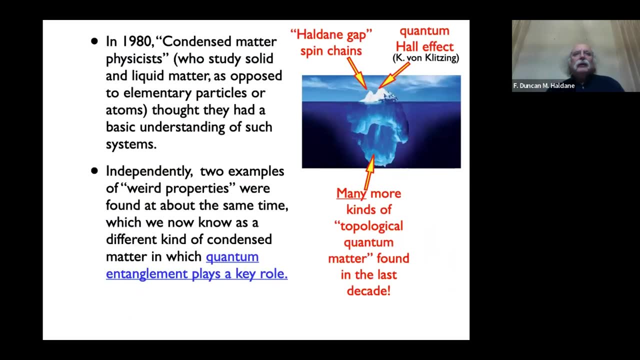 without having to go back to Paris to check your device. Okay, so what's happening here? Okay, sorry. So around 1980, condensed matter- physicists who were studying things found- studying liquid and solid matter- were finding a couple of weird properties. 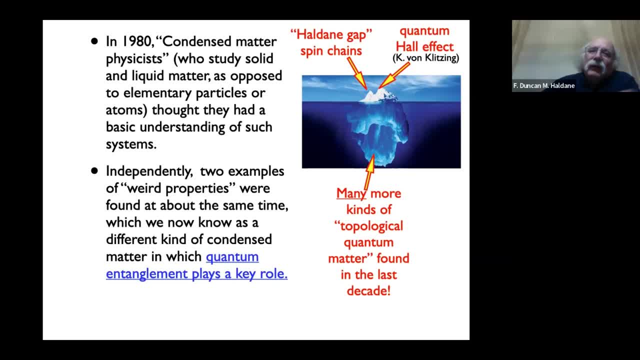 Two things that happened at the same time. almost One was Von Klitzing's discovery of the of the integer quantum Hall effect, And I was actually working on spin chains that turned out to be have a topological state in them too. 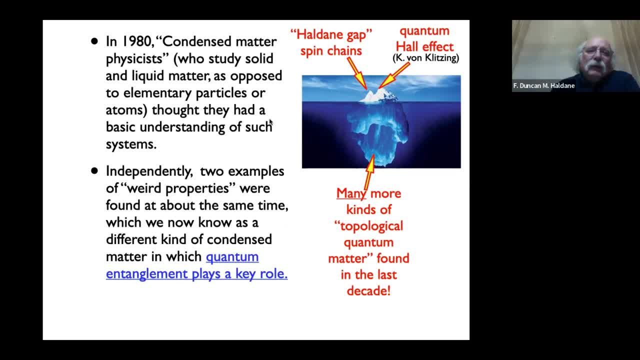 And these are kind of. these were kind of very weird examples which didn't seem to fit at the time, And now we know they're the new kind of condensed matter, which is which we call topological quantum matter, in which in some sense, 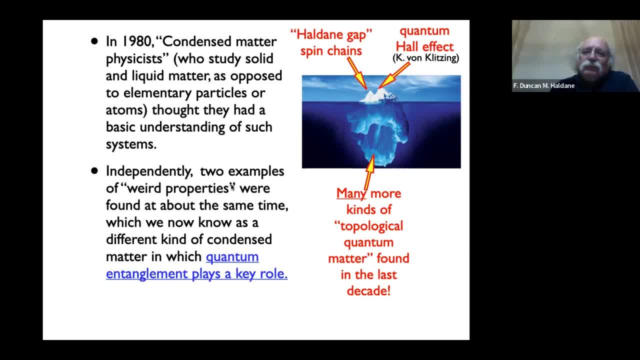 quantum entanglement is playing an important role And of course, many more different kinds of topological quantum matter being found in the last 20, 40 years, especially in the last decade or so, And so now we have a big kind of general picture of topological quantum matter. 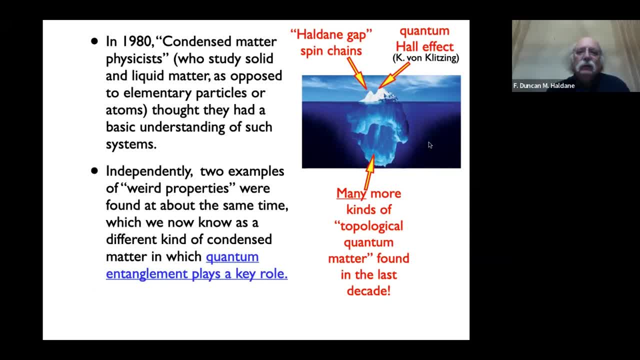 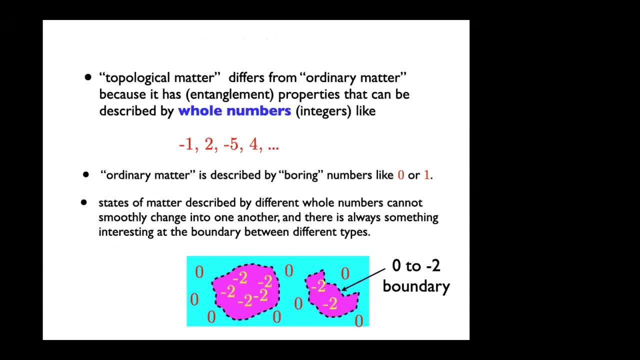 Let's see if my Elemental question. Okay, Here you are A question. Can I? Yeah, Question, Yeah. So in the previous page you mentioned about two terminology: topology in quantum entanglement. So can I have? I'm all. 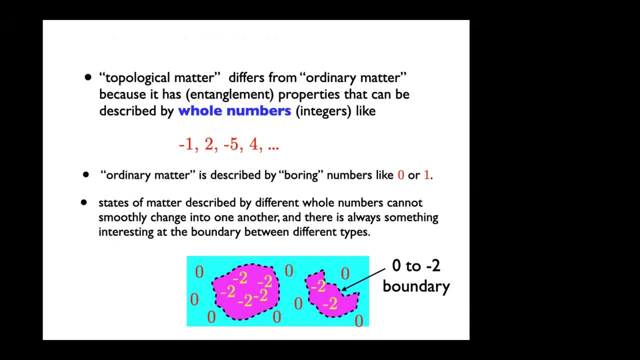 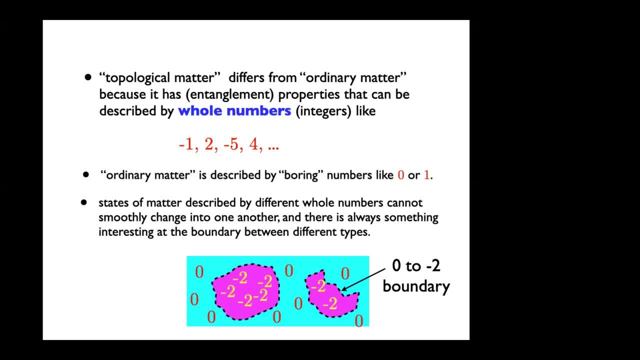 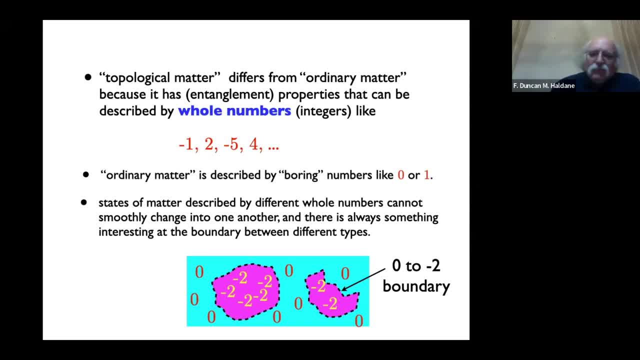 Can I have, although I think somewhat earlier stage to ask, but can you give me more on some Manalese direct, Some intuitive relation between entanglement and topology? Can I Okay When a topological structure in a system, there's a kind of connectedness across it? 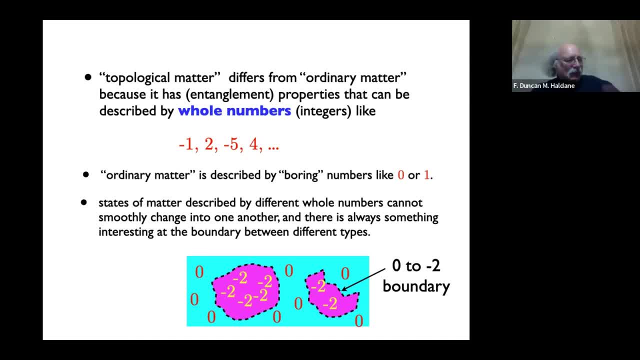 Basically, the edge states really come from the fact there's some kind of entanglement in the bulk. that is different. You can't just chop the thing into. let me see if the slides have it, Let me just move on and we'll see what happens here. okay. 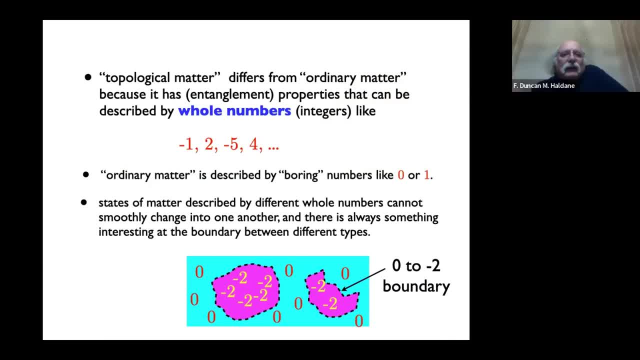 So I would say that, yeah, the basic feature is that topological structures have something that passes through the system. So, for example, in the spin chains, in the AKLT spin chain, you split The spin ones into two spin halves which join in each direction and form a chain that passes through the thing. 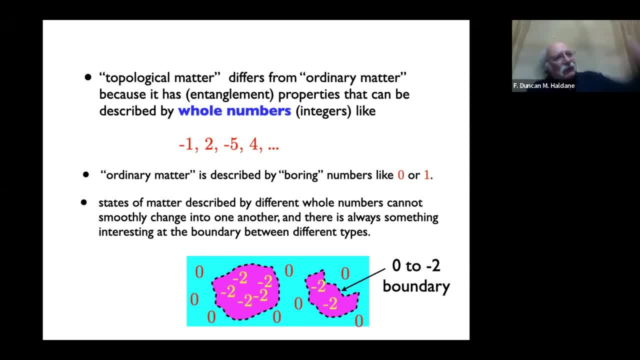 So by cutting the system in half you get non-trivial entanglement spectra at the bound when you break it. Let me move on. okay, Okay, thank you, Okay, yeah, So I guess basically a topological matter has got something where the properties 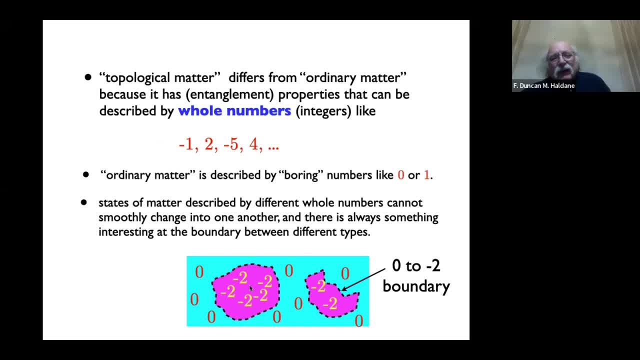 These depend on whole numbers, right, And basically whole numbers can't change continuously. So if you can classify something's topology by an integer of some kind, then where a different kind of matter occurs on the other side of a boundary, 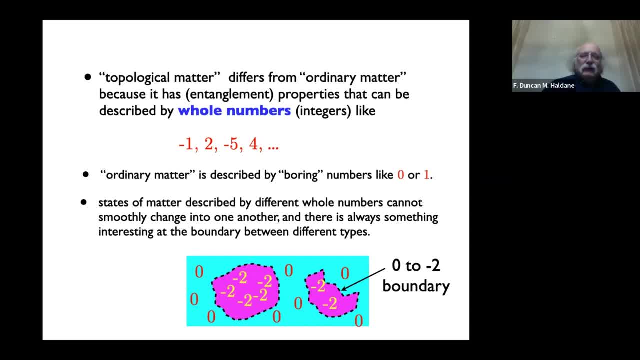 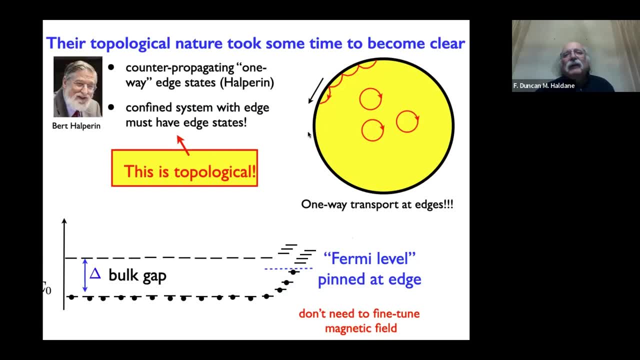 there has to be something happening at the boundary And indeed in the quantum Hall effect. it took some time for the for the topology to become clear, but one of the clearer things in it is that, if I have this, these electrons going around in little circles inside this quantum Hall regime region. 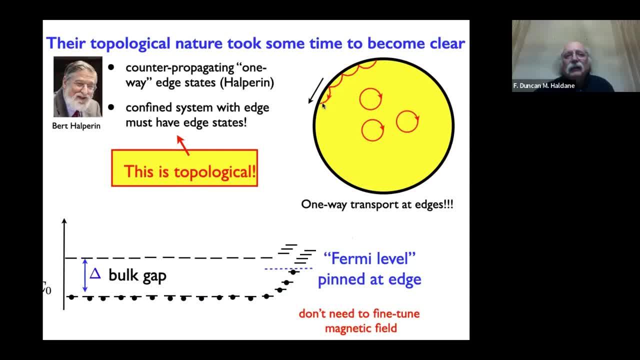 if the circles or the orbits don't close but bounce off the boundary, then you get states which go around, in this case, in one direction only, which is a very strange property. They go around If the picture shows, If the picture shows the internal orbits being clockwise, in which case if they collide with the edge, 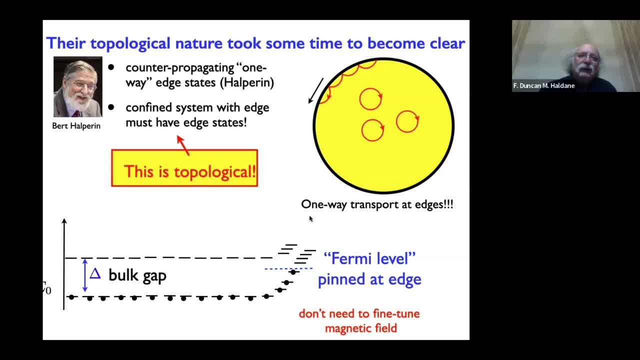 the modes at the edge go in the anticlockwise direction, And this is very typical of topological matter, where something funny is happening at the edge. And of course, in the experiment that von Klitzing did, other people had done essentially the same experiment before, but they did it in the wrong way. 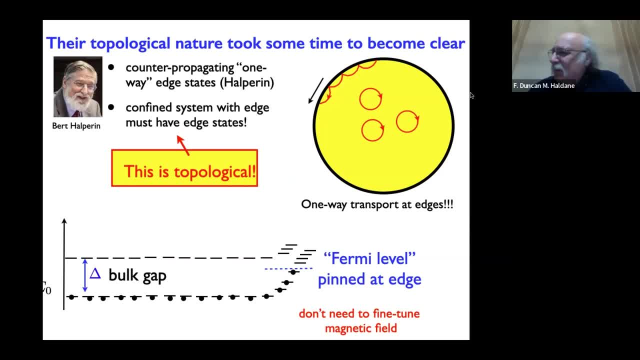 von Klitzing von Klitzing von Klitzing took his sample and he cranked up the magnetic field with a constant current generator flow, with a constant current flowing through the system von Klitzing von Klitzing. 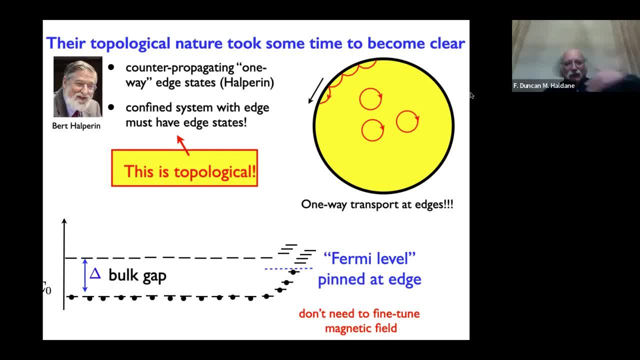 von Klitzing. And then he found that the whole voltage measured transverse to the current was the same number to That's. because you've got to keep up the magnetic field, you throw all of those Einstein moves and to run theanton. 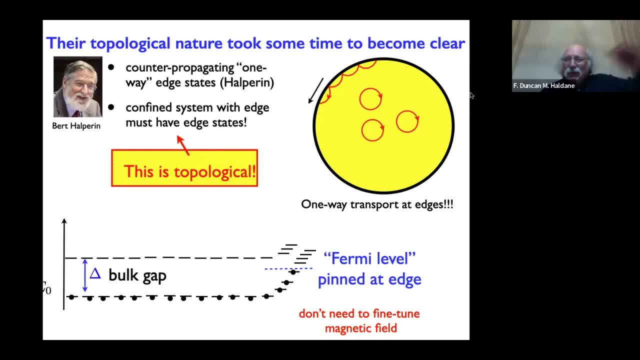 that time I think 304 significant figures. And of course you shouldn't get that, because each time you start the magnetic field up you've got a slightly different magnetic field at the end to exactly the same current, so you'll never see the same voltage. so the coo thing was that the 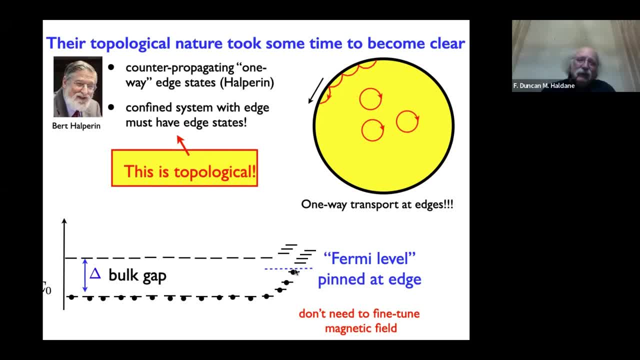 the edge states pin the fermi energy and as you change the magnetic field a little bit, the it doesn't affect the call constants. right states flow in and out of the of the landau levels from the edge states, but the so long as your fermi level stays in the gap. 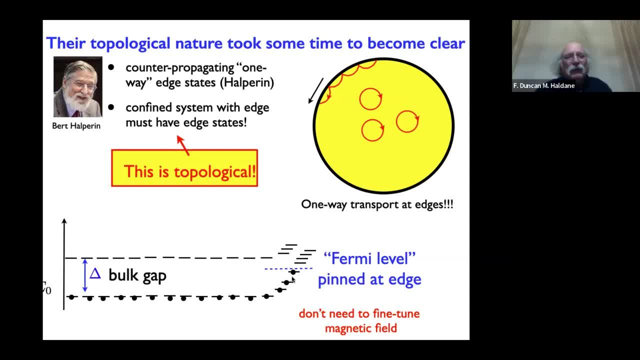 you get exactly the same, the same uh measurement for a fixed current. so the edge states were the crucial thing that actually allowed one klitzing to to discover the effect. i i believe that he initially thought there was something wrong with the voltmeter because, uh, you shouldn't get you. 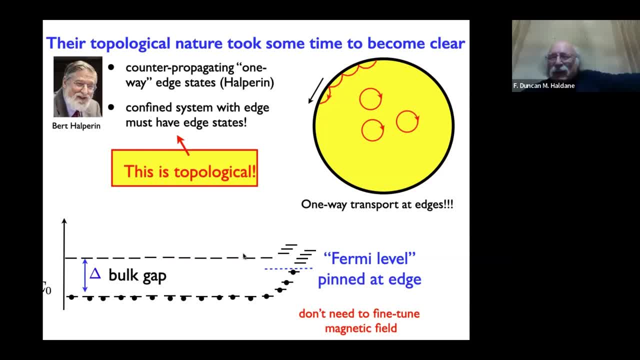 know digital voltmeter, you get this. if you get the same number occurring to to four or five significant figures, you think there's something, not something not working with your vault, with your digital voltmeter. but in fact that was the crucial thing. so topology is the is the crucial. 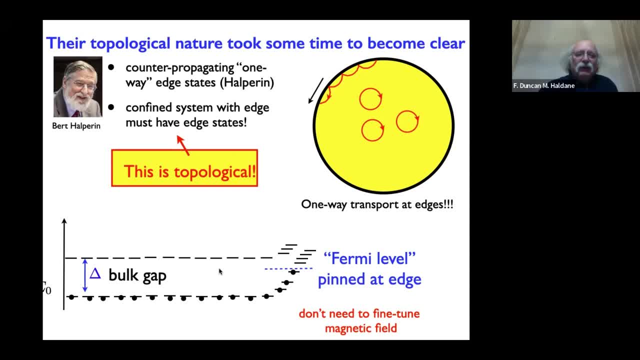 thing that actually gives rise to this perfect quantization of the, of the whole constant, and, of course, the issue about how well it's quantized. basically it's because the edge states die off exponentially into the bulk so long as no other edge is closed. in units of the decay length to the first edge, then you get this perfect number. okay. 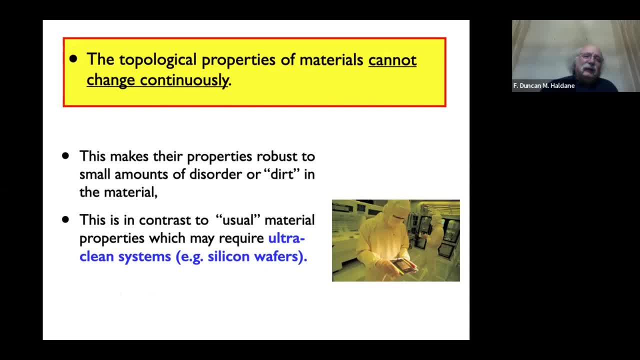 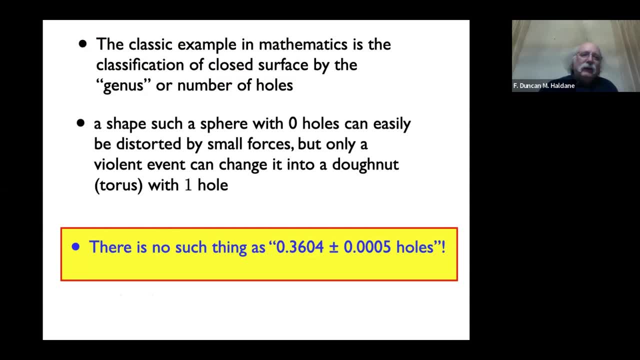 so topological properties of materials can't change continuously and that makes them kind of robust, okay. and of course the whole thing that we see all the time in experimental talks about, um, topological insulators is that people show the famous uh, gauss-bonnet thing. so 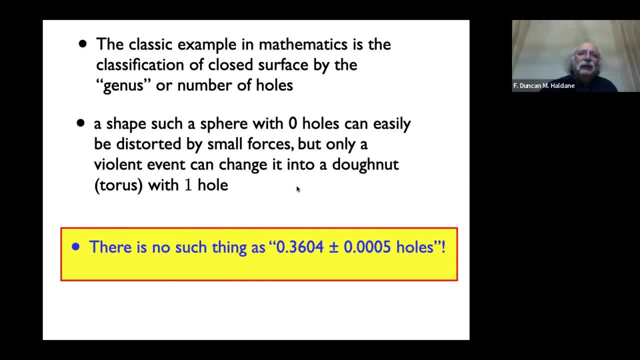 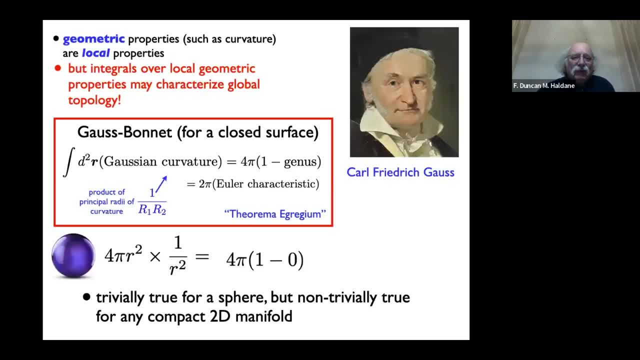 classical examples of topology is classifying surfaces by their genus, the number of holes, and holes are quantized, they come in integer amounts and we get the famous uh gauss-bonnet formula. and of course, the surprising thing is that um gauss-bonnet has a uh generalization by churn uh to a much more. 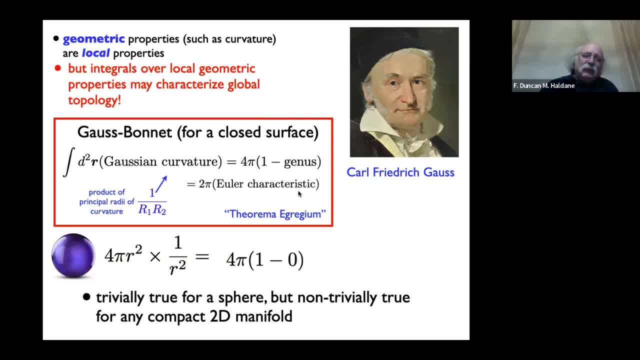 abstract form of gauss-bonnet, and it's the abstract form of gauss-bonnet that uh ended up providing a key. the key element of why the whole constant, the whole uh conductivity was, was quantized by linking it to the churn number. okay, let's move on a bit. 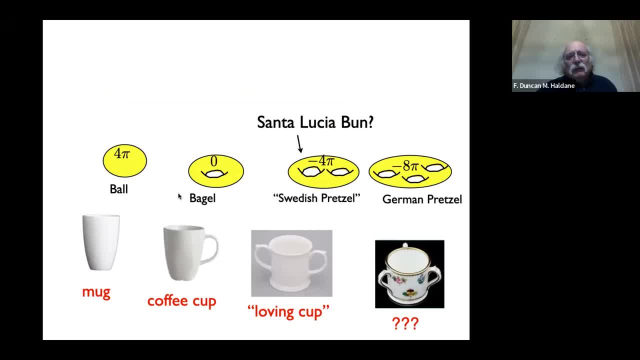 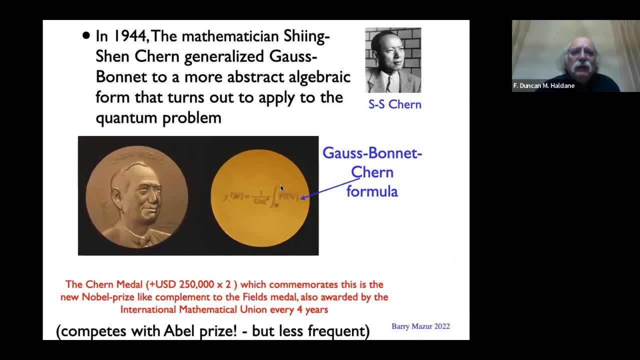 so, anyway, here's the old story about, um, about coffee cups turning into donuts and etc. so let's, i guess, and there's the, the churn formula, and the churn formula, uh, gauss-bonnet churn formula, is on the back of the, the churn medal, which is, uh, one of the 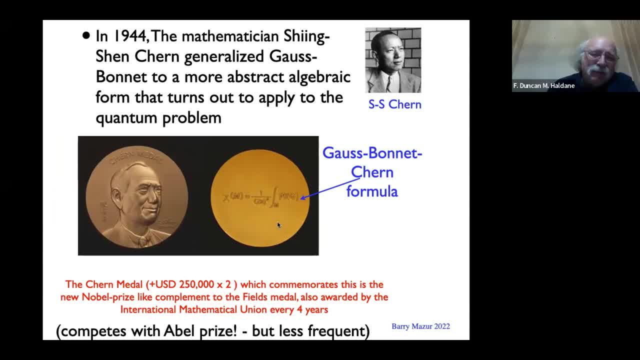 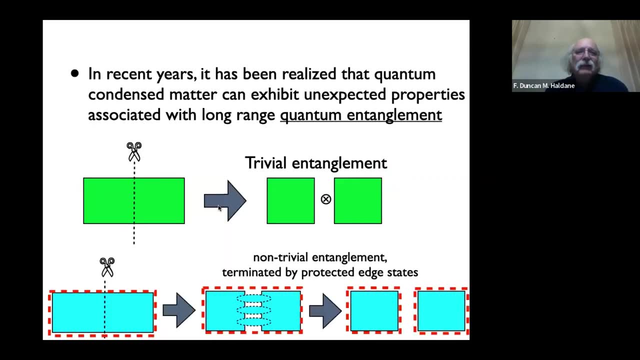 one of the kind of non-feel, the, since the fields metal in math is restricted to people below 40, it's a kind of noble one of the one of these kind of lifetime achievement things, which is a which is open to mathematicians of any age. okay, okay, so. so the basic issue of uh. 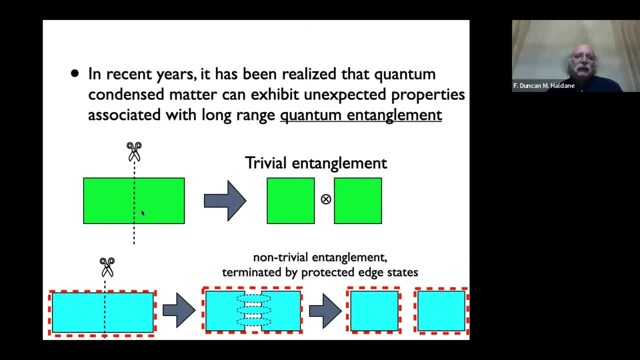 entanglement is here. if i have a if, if i have two pieces of the sample which are trivially entangled- i not entangled, basically, or very weakly entangled- i can chop the thing in half and i will just get a direct, essentially a direct product state of of the two pieces. 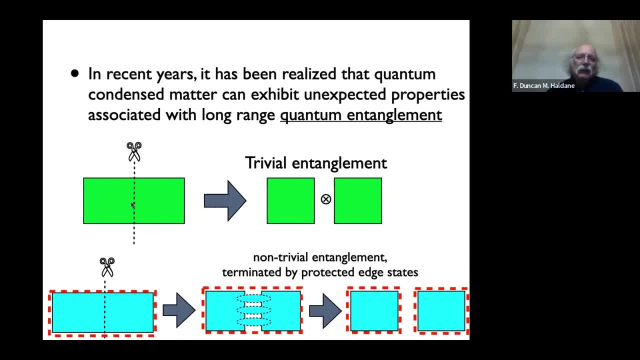 uh, so top of non-topological matter will have a small amount of entanglement across the boundary, but it will no, no fundamental entanglement between the part of the sample over here and the part of the sample over here. oops, but if i have the um uh, the topological, 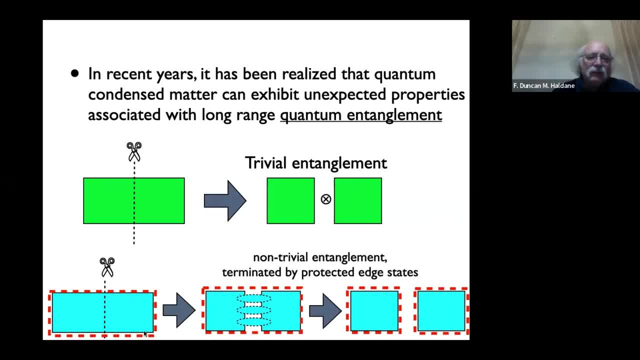 matter, the topological matter has an edge state around it, on its boundary, and if i try to chop it into two halves, to do a um, it will resist at first. but uh, if i managed to, if i managed to divide it into two, once it's separated, the topological edge states will have have now covered the, the open, the boundary that 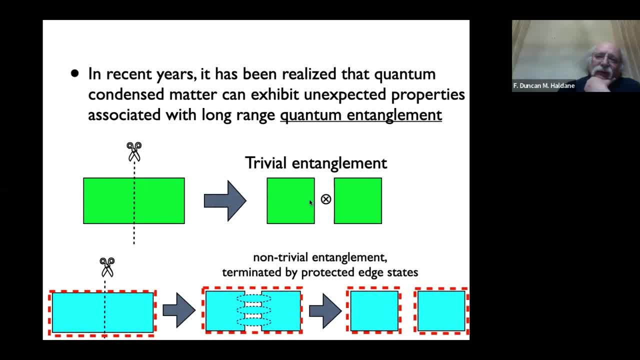 got exposed and that's clearly that the question that was was: where was the entanglement taking place? there's this feature that there's a just a non-trivial entanglement. uh, and in fact if you calculate the schmidt um spectrum, the entanglement spectrum between the 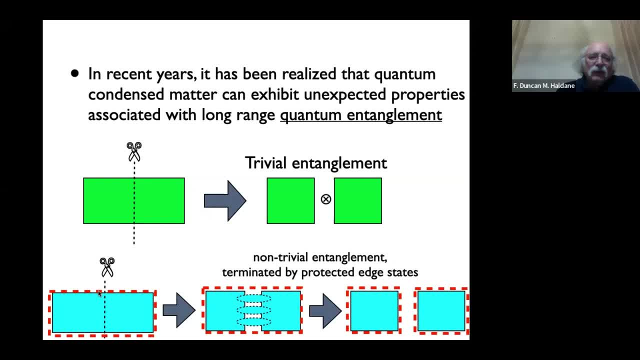 between the two halves of the thing before i cut it. you will, of course you will. you will find out that the entanglement spectrum contains an image of the edge state, the physical edge state, which will appear if i do actually divide it in half. so the entanglement is invisible, as is shown up by 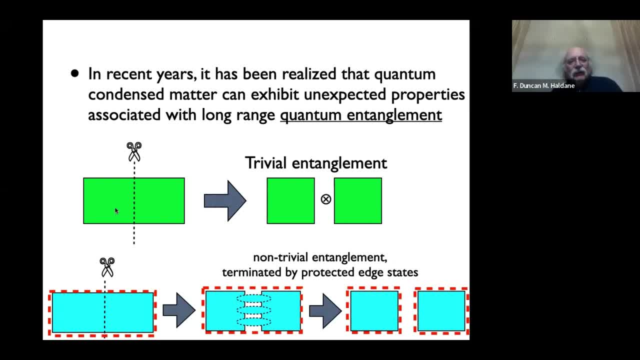 the entanglement spectrum. the entanglement spectrum is actually divided in half. so the fixed edge, the edge, is actually the edge, um, the edge of the edge, uh, so the edge of the edge. basically, if you do the hebd or the edge of the edge, you can calculate it as the surface of the 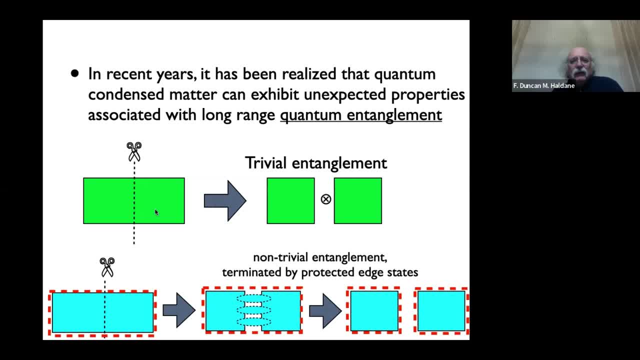 edge at once. as you do it by uh, by basically doing a partial trace over one one side, uh will reveals, reveals the edge states. so the h states are there because they have to be there, because there's actually entanglement in the, by just doing this mathematical procedure of the Schmidt decomposition of the right and left sides. 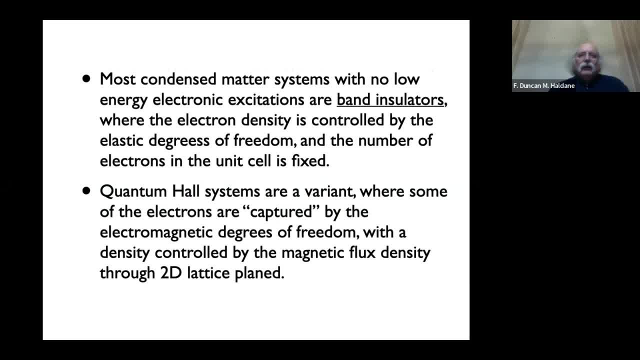 of the sample. Okay, So most condensed matter systems with no low energy electronic excitations are band insulators. Okay, And so you can say they're incompressible. The electron states are incompressible If there's no low energy electronic excitations. the density of the 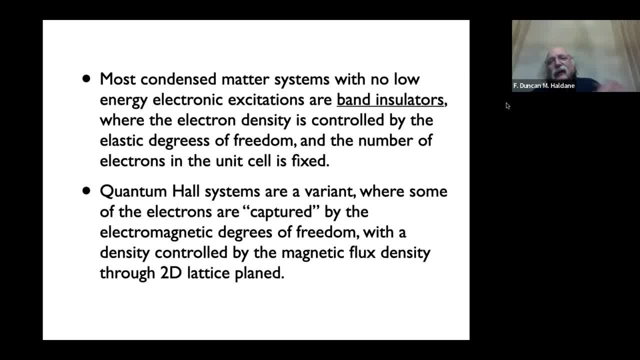 electrons is controlled by something else, And in the usual case it's a band insulator. It's the elastic degrees of freedom that That control the electron density. It's completely fixed by the volume of the Brillouin zone, which is determined by the Bragg vectors of crystalline order, So the quantum Hall systems. 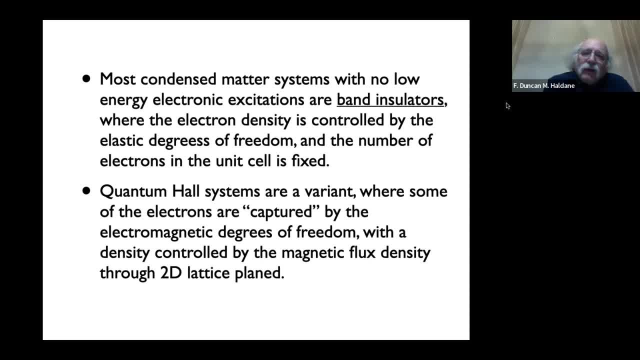 actually Conceptually they're a variant. There's The electrons have actually been captured, not Has been. There's still a system with no low energy degrees of freedoms, so the electrons are captive to something else. but some of the electrons have been. 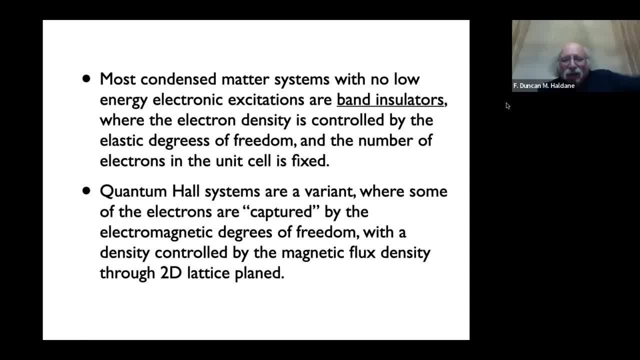 stolen away by the electromagnetic degrees and now controlled by the electromagnetic degrees of freedom. And the density is now controlled by a magnetic flux density through a 2D lattice plane. So basically, in the quantum Hall, In the quantum whole effect, some electrons that live on a On a lattice plane have Are slowing down Or there's. 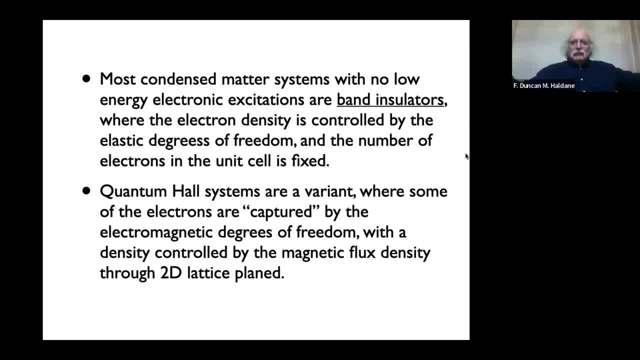 no Thanks. a two. now, when lambda levels form now belong to the electromagnetic fields and they no longer. most of the electrons are still controlled by the, by the elastic degrees of freedom. they live in bands which are don't have, which are not churned bands, but um, the quantum hall effect basically means some of the electrons are still. 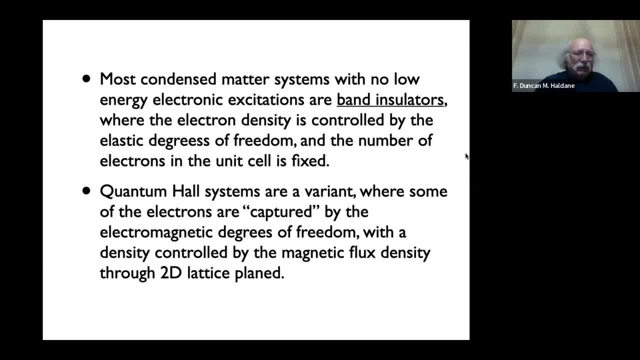 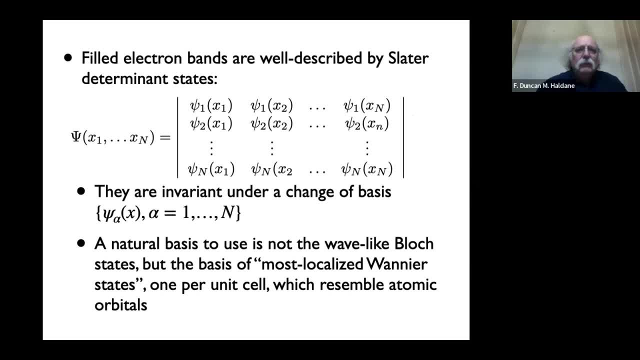 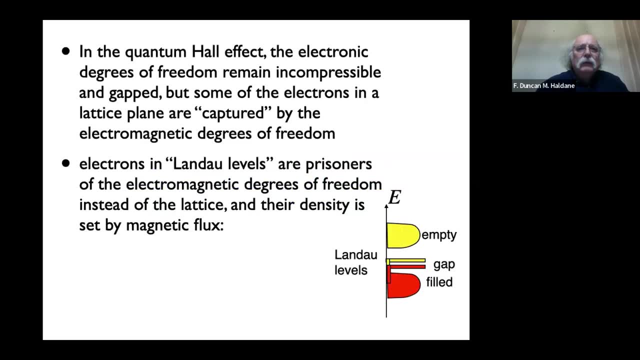 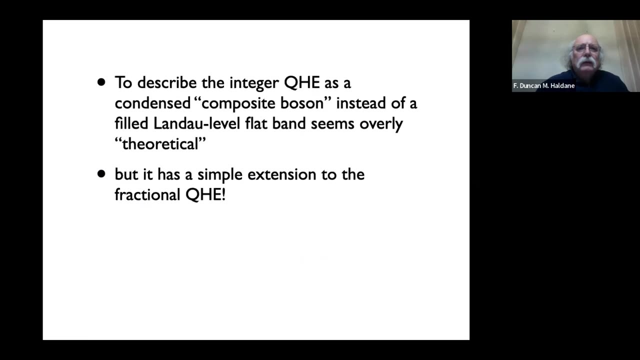 captive, but now they belong to the electromagnetic fields. okay, okay, let's see if i can get this to. so okay, let's see my. let's see if i'm right question. sorry, i'm trying to get to my. i've got some problem in getting to. let's go there's. 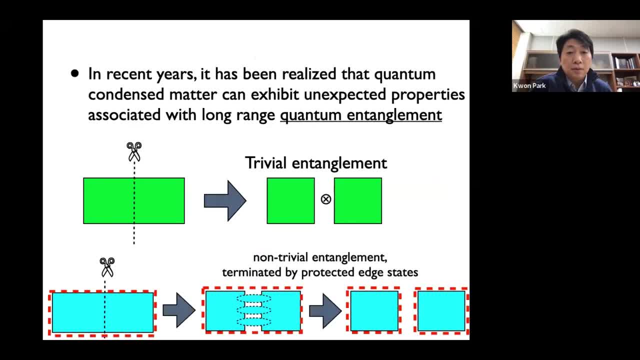 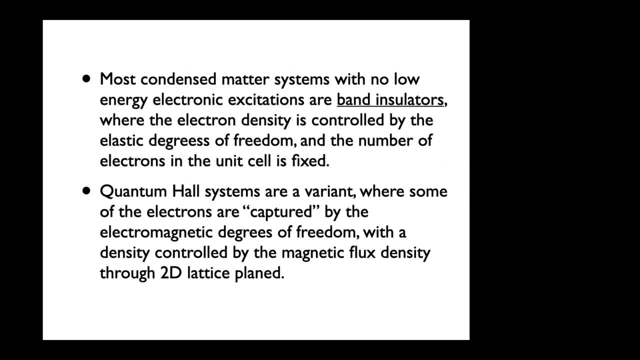 a question. you can get back to the beginning, don't go. there's a question. yeah, oh yeah, question, uh. so let me try to understand the meaning of elastic degree of freedom. if i recall, the tinder theorem is- so you mentioned that- the area of brilliance. i mean it's the electronic number. but so is there any elasticity of freedom in the? 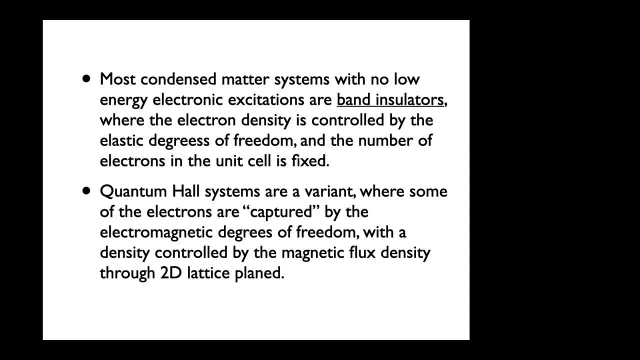 latin, the theorem or so. so what would apply when you have a fermi surface? yes, so if it's a band insulator, there's no fermi surface and there's no low energy, electronic degrees of freedom. so the electrons themselves, they're, they're, they can't do much right. 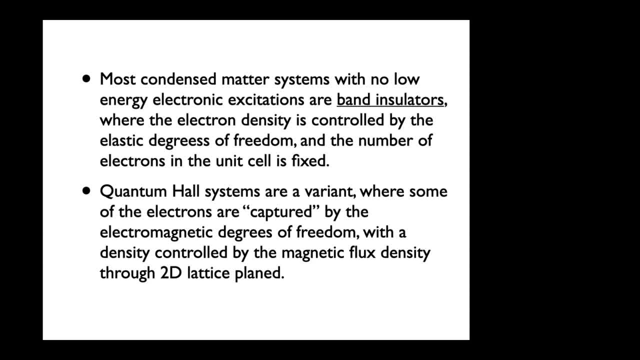 they're directed by something else. so if it's, if it's a band insulator, there's going to be a a whole, not an integer number of electrons per unit, per unit cell, and so the electron density can only be controlled by varying the unit cell volume, and the only thing that does that would be. 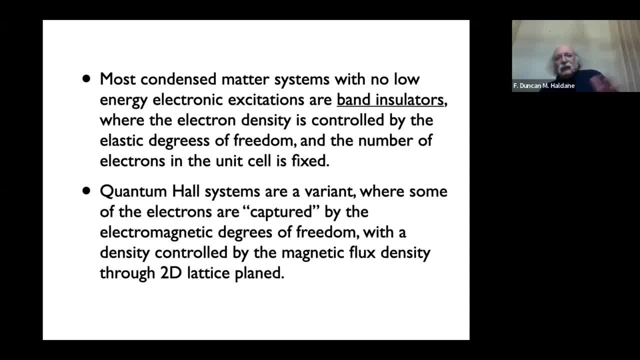 longitudinal phonons. so the electron density is completely fixed by the elastic degrees of freedom of the crystal uh. but when you have a quantum hall effect, some of the some part of the electron density is now becomes controlled by a magnetic flux through a lattice plane, and so that those electrons- the one that participate- 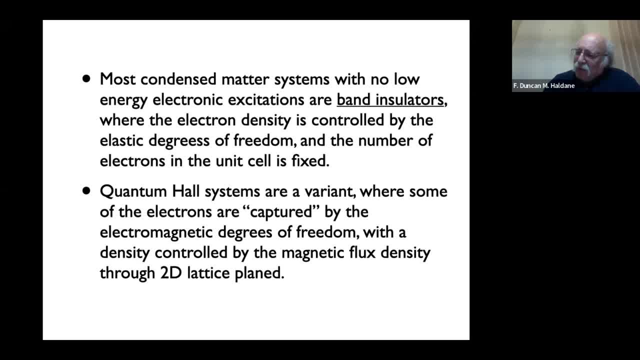 in the um fracture in the quantum hall effect. those electrons are uh, have lost contact, have lost connection with the underlying lattice and are completely controlled by the um electromagnetic degrees of freedom. so the difference between a band insulator and the landau level, incompressible landau level state is that the landau level state is a fluid that can. 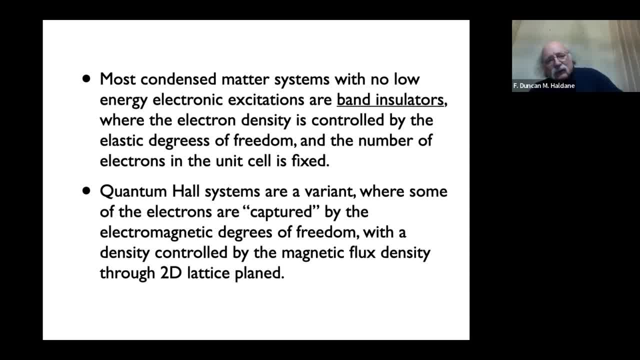 flow, the, the, the flow velocity is also completely controlled by the electromagnetic degrees of freedom, and it's just the electromagnetic drift velocity e over b. so not only is the density of electrons, uh, fixed by the magnetic flux, but the current of electrons is completely controlled by the, the electric field, and in fact the, the gradient of the flow velocity, which maybe 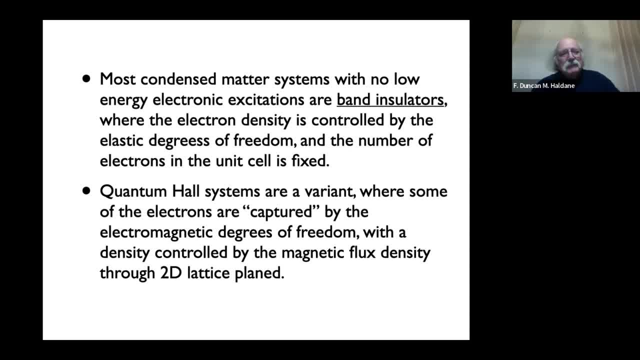 i'll come to, which defines the viscosity of the electron system, which is a dissipation of viscosity in landau levels. the gradient of the electric field drives uh differential flow velocities uh have. so if it's a uniform electric field, the flow, everything flows at the same rate. 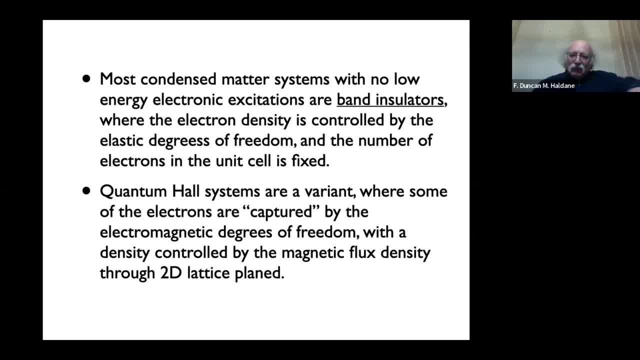 uh, with a gradients of electric field you have, you have differential flow. so the the quantum system is is is incompressible, but it is belong the electrons that participate in it belong, belong to the lat, belong to the electromagnetic field and and they do what they're told to do by the electromagnetic field, they, they. 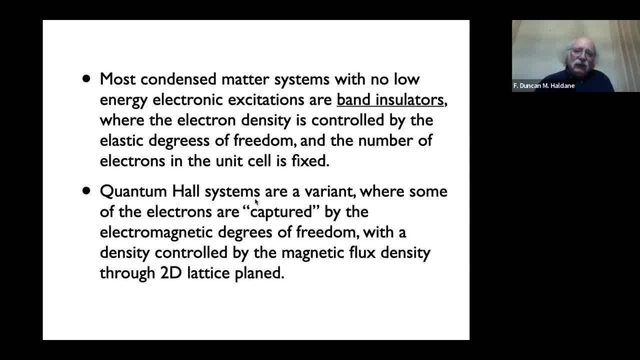 have a density fixed by the, by the b fields, and they have a current which is fixed by the electric field, and that's, of course, the um, the quantum hall effect, that the current, uh, and the current, of course, is a dissipationless current, so it's at right angles to the electric field. okay, so, 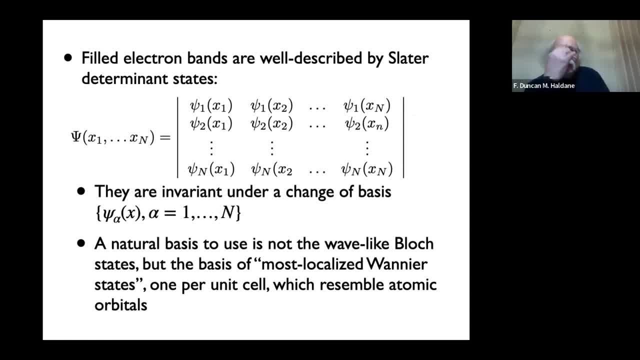 so, uh, filled electron bands, of course, are well described by slated determinant states, and the most important feature of a slater determinant state is probably that it's invariant under a change of basis, right? so, of course, what i've got here is: uh, i'll come back. 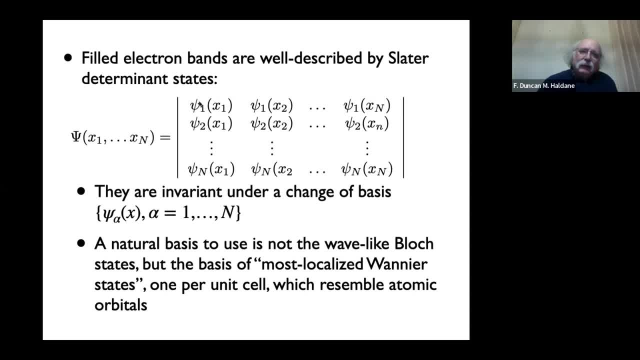 to this later. i've got here, uh, the slater determined i've got some basis of single particle states which actually don't have to be orthogonal to each other because they just have to be linearly independent. and uh, then i have the coordinates of the electrons along along the columns. 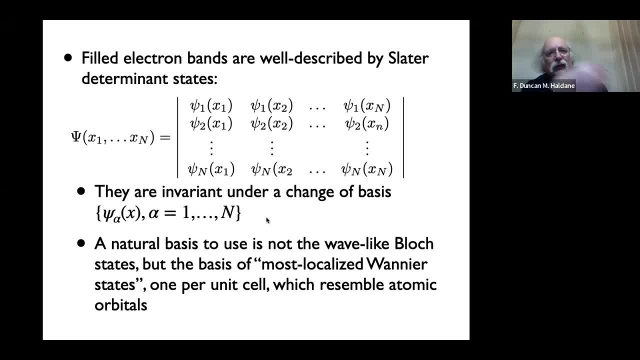 and all the other way around. um, so i'm going to go back to the, the third one, of course. what is so? you have a a large freedom of choice in describing a field band, and you might think the thing to do is describe it in terms of, of block states. but the natural basis in all things 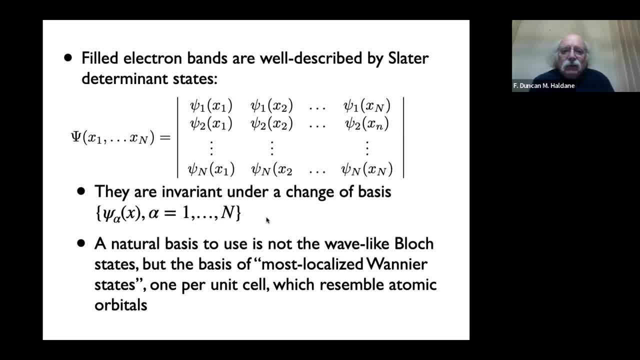 is really the local basis, and the local basis of a band is actually the, the basis which is so-called- And these basically resemble atomic orbitals and they're basically pinned down to the atomic positions. So once you adopt the, once you've found the most localized shape of these things, you can't adiabatically move those orbitals without changing their shape. 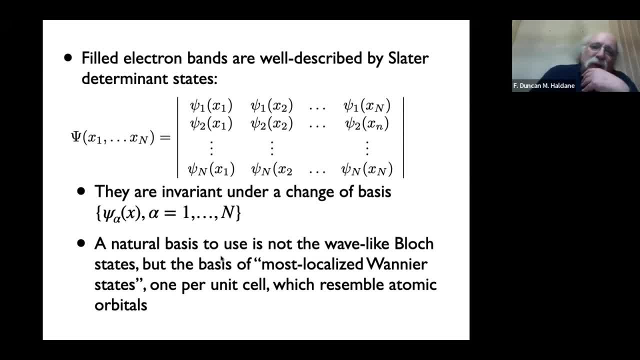 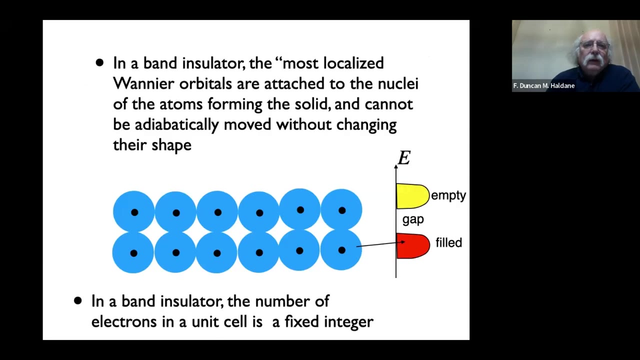 So the most the local basis that you get for describing a band is nailed down and attached to the lattice. but that's not going to be the case for Landau levels. Something doesn't work, okay, Yeah, Okay. so in a band insulator, the most the most localized Guani orbitals are attached to the band. 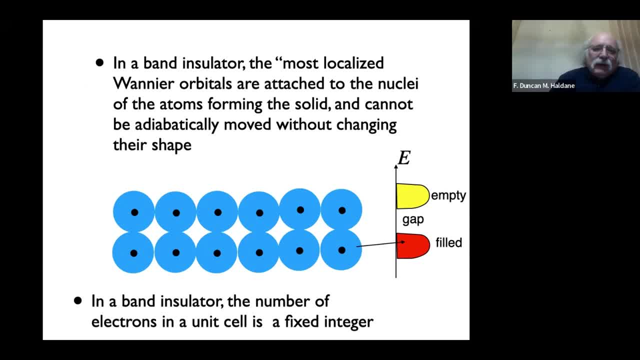 The nuclei of the atom, and so you can't move them adiabatically and, of course, in a band insulator. If I could move this In a band insulator. the number of electrons in the unit cells are fixed integer. 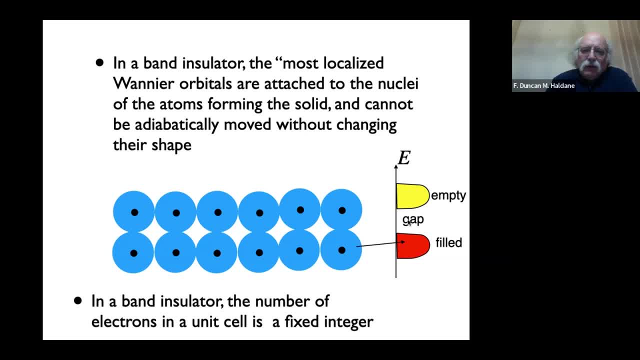 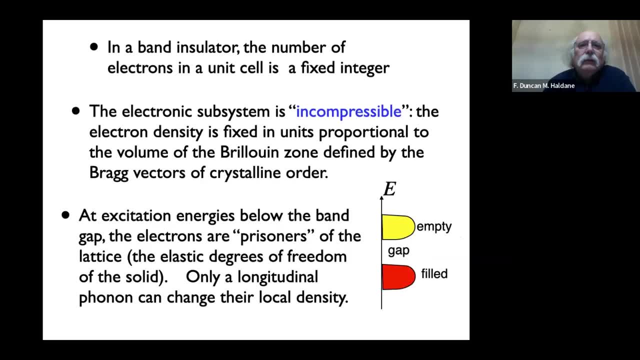 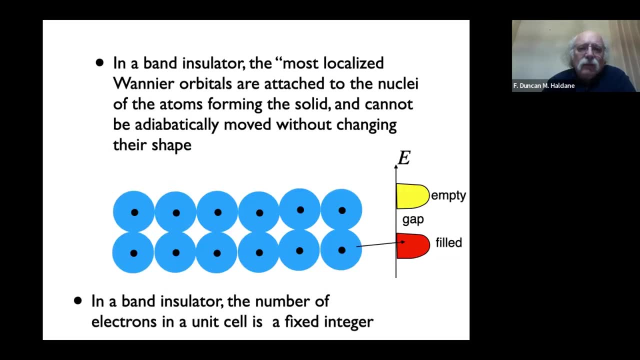 And we have a gap, Right. So let's now think about the Why my thing stopped working. Okay, So you can't move a band insulator because the electron density is proportional to the volume of the bullion zone. Yeah, there we are, Okay. 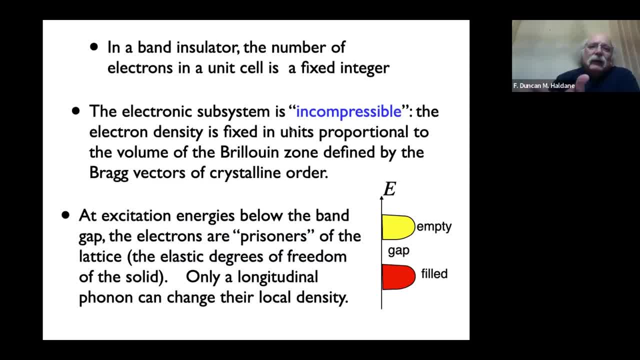 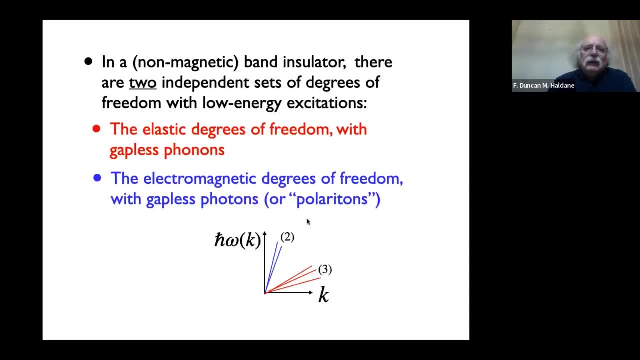 Okay, so The electric, basically electron, subsystem is incompressible because the electron density is proportional to the volume of the bullion zone, And So that's what I've already said. So in a non-magnetic band insulator we have like two independent steps of degrees of freedom with low-energy excitations. 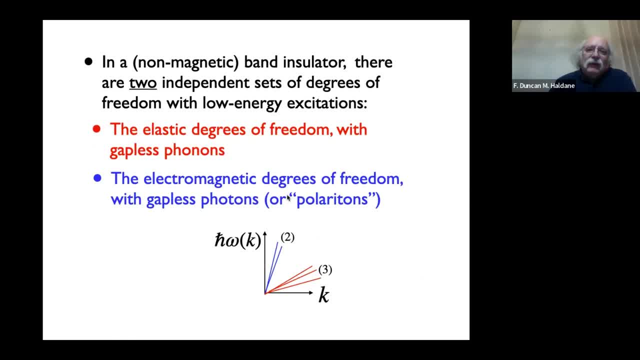 The elastic ones, which are the phonons, and the electromagnetic ones with the photons or polaritons. And so if you have a conductor, of course you've got lots and lots of low-energy electronic degrees of freedom. But we were dealing with the case where the electrons are incompressible. 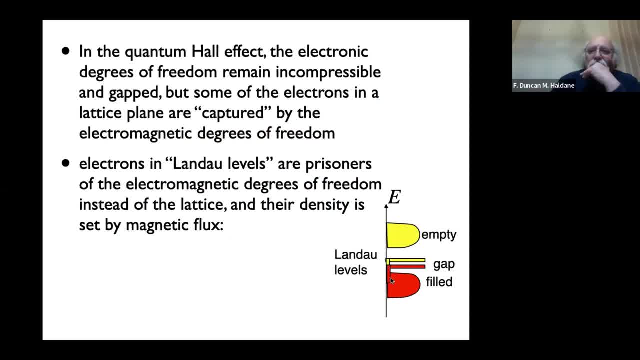 So in the quantum Hall effect now we out of the tops and bottoms of the bands, when we apply a magnetic flux to the system, we start to get lambda levels, And the density of electrons in a filled lambda level is of course set by the magnetic flux. as I said, 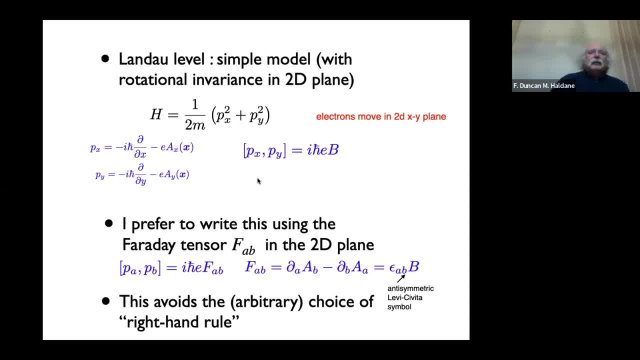 So let's look at the lambda levels in a bit more detail, And what I'm going to give you is a kind of composite boson picture of the integer Hall effect, which will immediately generalize to a much, much more interesting composite boson picture of the fractional Hall effect. 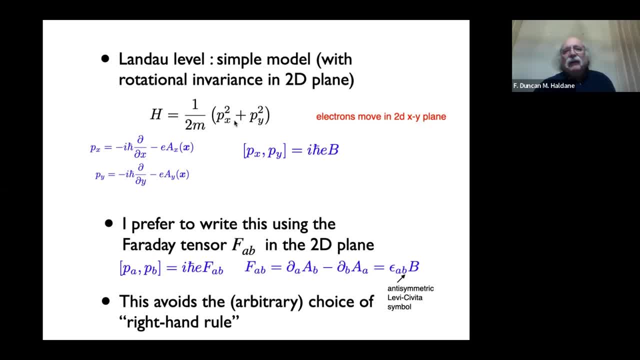 So we can start off with the simplest model of lambda levels, which is a rotationally invariant lambda Level, And one point I'm going to make is that actually, in real life, lambda levels are not rotationally invariant, because they're derived not from Newtonian mechanics but from a band structure. 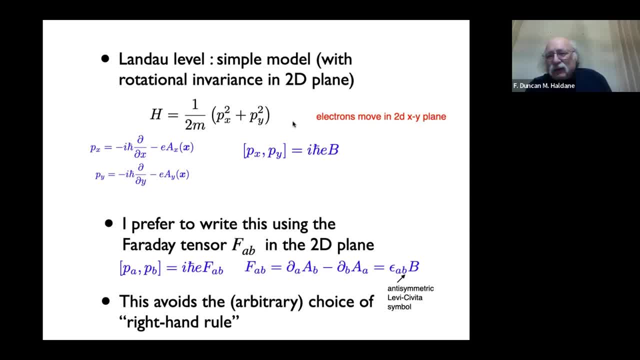 And, in condensed matter, there is no such thing as continuous rotational invariance. So the simple models which have it for quantum Hall they have. the rotational invariance of these models is the toy model feature. So one has to be suspicious about the generality of the results one derive using the using these very simple models where there's a conserved angular momentum. 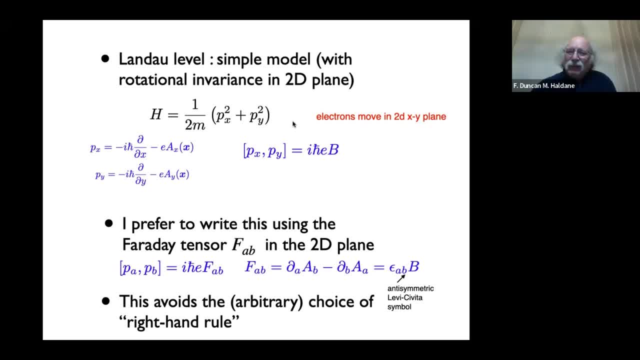 Condensed matter does not have anything like conserved angular momentum in it, Just field theories do, and the vacuum has it, but not inside crystalline matter. So of course the key thing in the lambda levels is that the presence of the magnetic field means that the 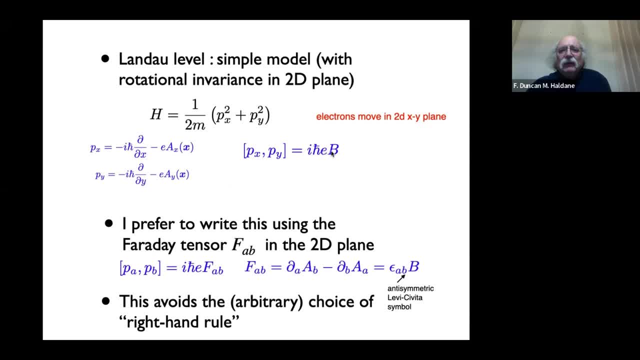 momentum, the dynamical momentum components no longer commute and have a nonzero, have a Heisenberg algebra where their commutator is a nonzero C number on the right hand side. OK, So actually, for many purposes it's, it's actually preferable not to use this notation of B, because B here means the magnetic flux normal to the plane. 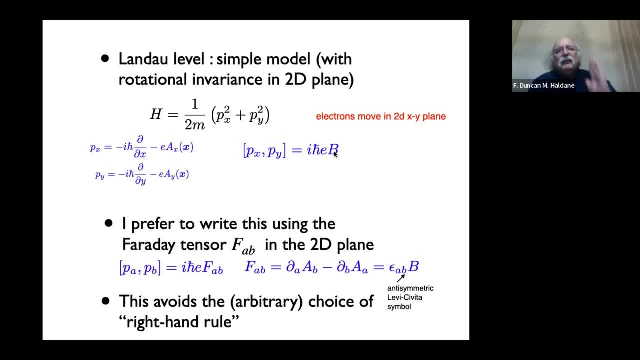 But then are we talking about The flux going from bottom to top, from lower to higher or higher to lower, And, in fact, one of the things you have learned in electromagnetism: you spend your time teaching the students the, the right hand rule for working out what the electromagnetic forces are. 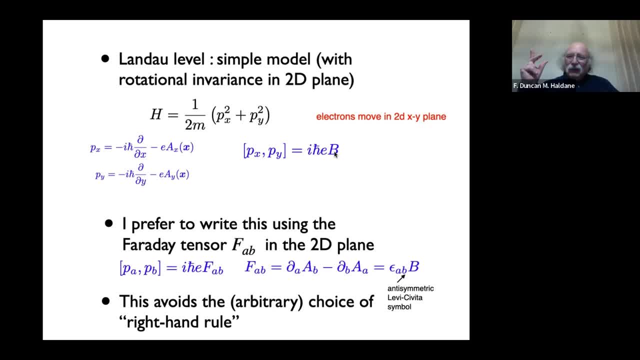 But of course the right hand rule is a complete, is a gauge choice, because someone in Alpha Centauri could have, aliens in Alpha Centauri could have, if they had hands, could have chosen the left hand rule. So you actually want to avoid this orientational choice. 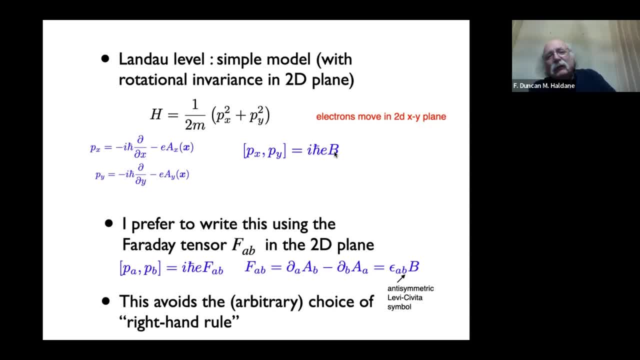 So it's actually many of the formulas, especially in two dimensions, turn out to look a lot better if you express them not in terms of B but in terms of the Faraday tensor. And the Faraday tensor has got is an anti-symmetric tensor in the plane. 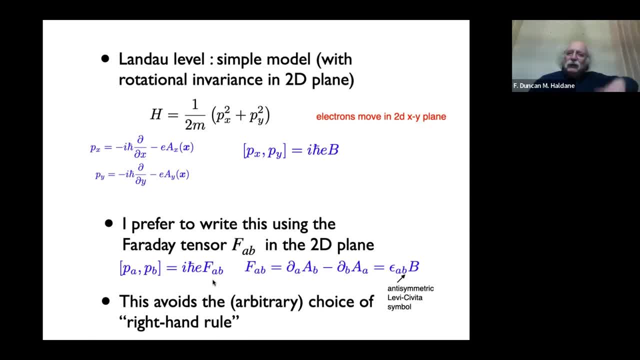 So it's got no, no reference to normal, to the normal, to the plane or anything in it. OK, And so then the commutation Relations of the momenta are just the Faraday tensor, And if we need to use a B field notation, we have to introduce an anti-symmetric symbol, which has a handedness ambiguity, and a B field which has a handedness and ambiguity. 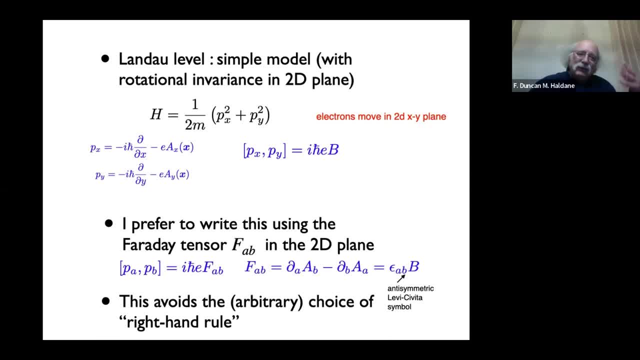 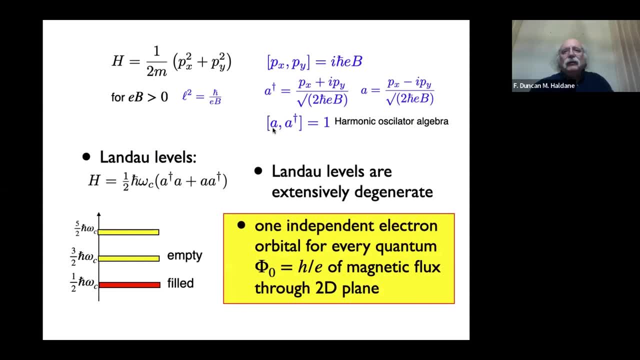 But the product of the two, which is the Faraday tensor, is completely generic. OK, So of course we work This out And of course, the crucial, of course, with this simple model we have, we can solve it as a harmonic oscillator problem. 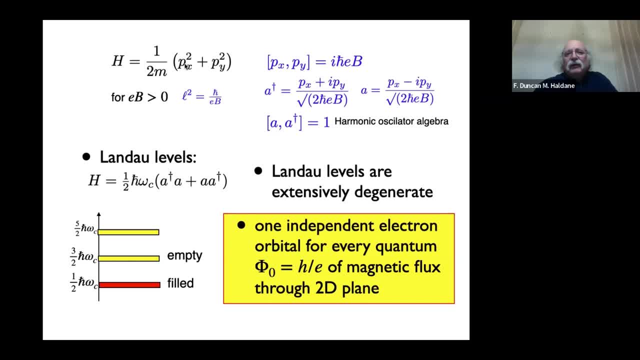 The more general lambda level problem doesn't have to have a quadratic dispersion. here It has. it has some dispersion which, if it's lambda quantization, it just means that the constant, the contours of constant energy are closed, are closed paths in the Brillouin zone. 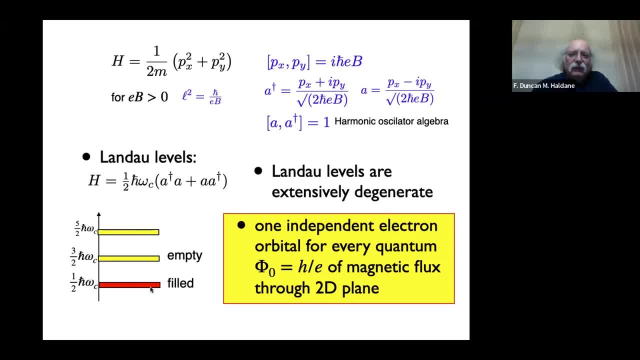 So, but again, it's very simple to use the harmonic Oscillator form And the key point, of course, is that the lambda level is extensively degenerate And there's one independent electron orbital for every quantum of magnetic flux passing through the two dimensional plane. every London quantum of magnetic flux. 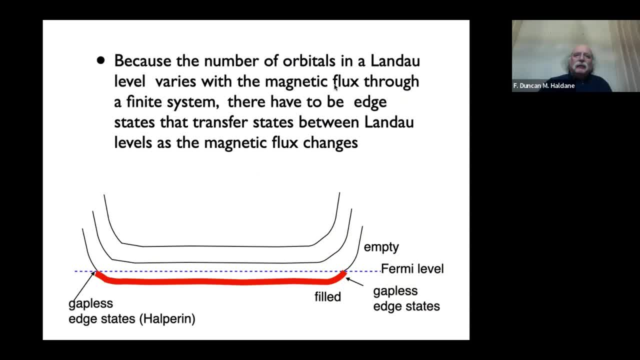 And, of course, because the number of orbitals in the lambda level is varying with the magnetic flux through a finite system, they automatically have to be edge states that allow States to be transferred from above the Fermi level, from the, from higher energies, down into the, into the lambda levels that are occupied. 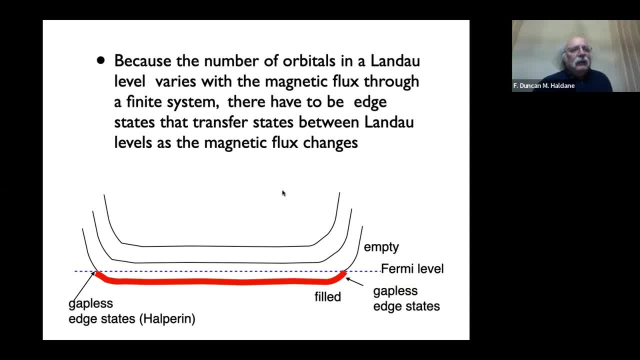 So the fact that the there's not the, the magnetic flux density can be varied continuously and the number of states changes in a in a in a lambda, in a in a narrow band. lambda level changes as you change. The flux means you automatically have to. 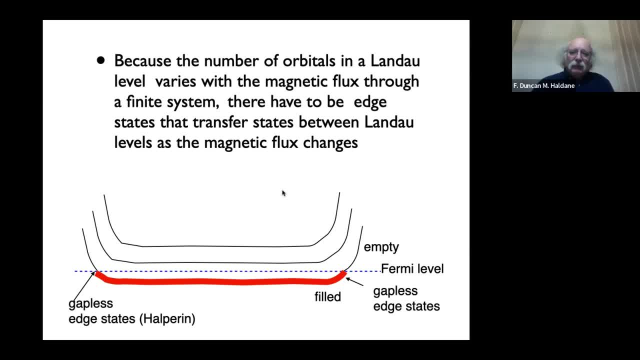 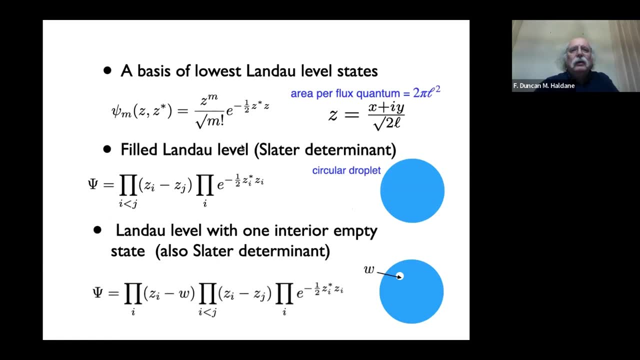 Have these topological, the required edge states at the edge of the system, which is of course, one of the features one finds quite generally in topological systems. OK, OK, so Let's look at the lambda level and of course, the simplest basis of lowest lambda level states that: 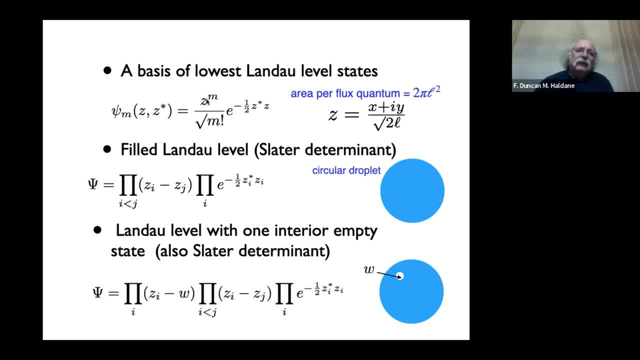 Everyone learns. They sometimes call it the, the symmetric gauge basis, but really The choice of a basis is nothing to do with gauge. it may look a basis may look better, it may look more appealing in some gauge, but the, the basis here, is a nice, it's a basis of circular, circular state. 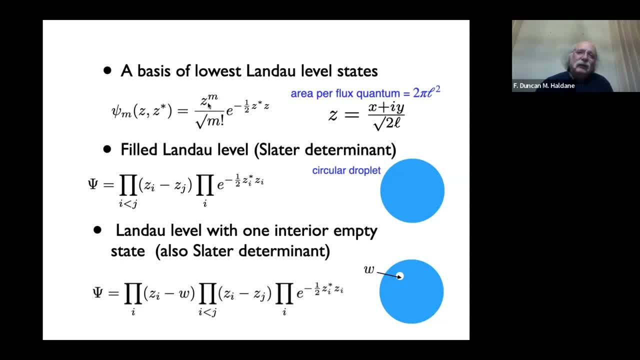 And so we have the, the feature that everyone is impressed by- that The lowest lambda level of these rotationally invariant levels. And so we have the, the feature that everyone is impressed by- that The lowest lambda level of these rotationally invariant levels Is- 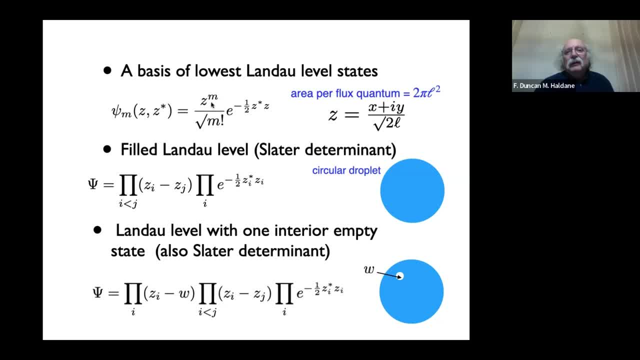 The states are polynomials in in Z, which I, which I've now made dimensionalist, it's explicitly way of a square root of The magnetic length else which is defined. so the area Flux quantum is is tupal squared, And of course we can immediately then write down the 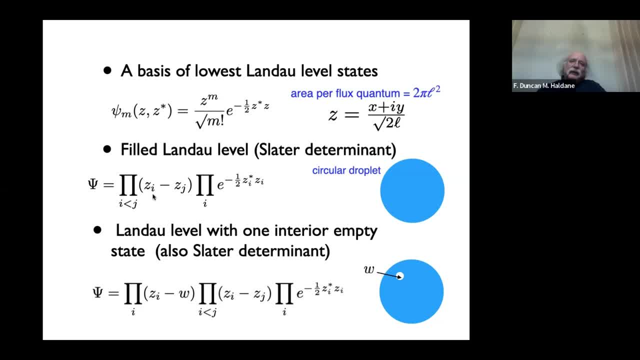 The slated determinant Of Examines That, that the state, which is, of course, the van der Maan determinant. It's the most the simplest anti-symmetric function. that's a polynomial in the Zs, and this describes the circular droplets. 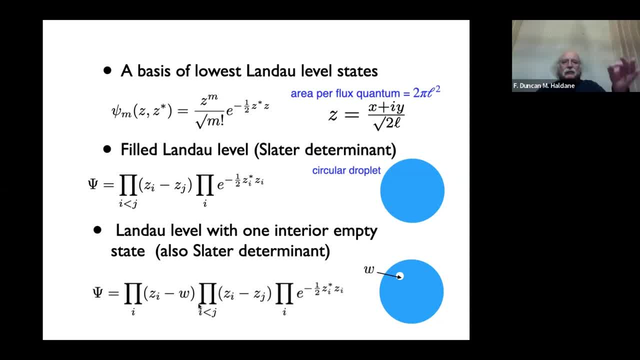 with edges, And now we can also look at the Landau level, with one empty state, interior state, which of course is still a Slater determinant- and we just have this feature that we put the orbital here at some arbitrary point And we can make a localized orbital at any point inside the 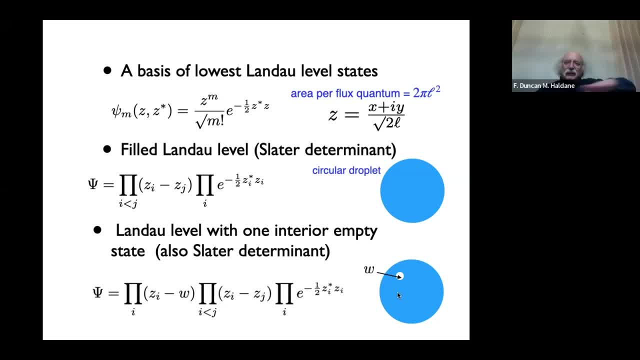 system, which is a distinction from the localized orbitals in a band insulator. The most localized orbitals in the band insulator are glued to the lattice positions and I can't adiabatically move those orbitals If I found the ones which are the most localized. 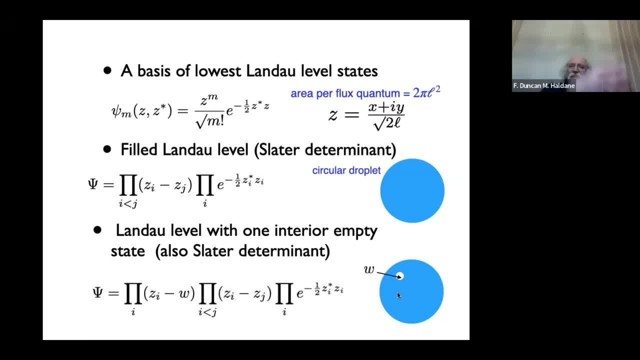 they can only be built in the band at some of the special points in the, basically at the atomic positions in the unit cell. Well, in the Landau level there was no connection whatsoever to the underlying lattice. If I go a little bit beyond the perfect degeneracy of the Landau level, 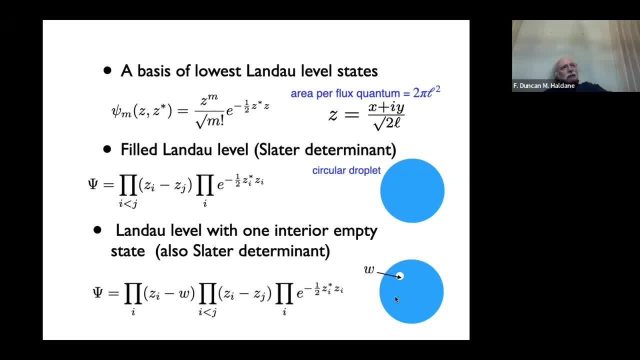 we get this Hofstadter-type spectrum. but basically the only corrections to the Landau level degeneracy are that if you have a closed orbit in one Brillouin zone somewhere there's an identical closed orbit displaced by a reciprocal vector in the next Brillouin zone And the only. 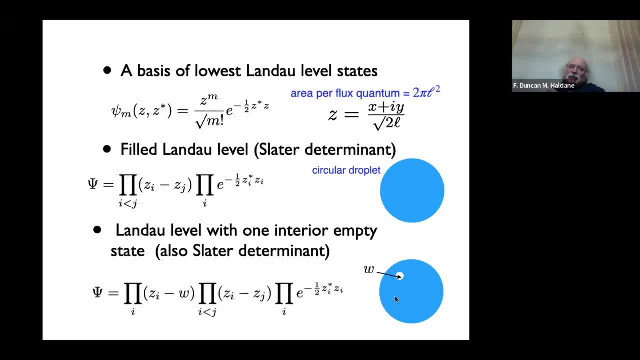 corrections which know anything about the lattice are the very exponentially weak tumbling between different closed orbits. So when the closed orbits are all well separated from each other in the Brillouin zone, then the land level becomes microscopically degenerate. And you see that in the Hofstadter model where you actually include a little bit of 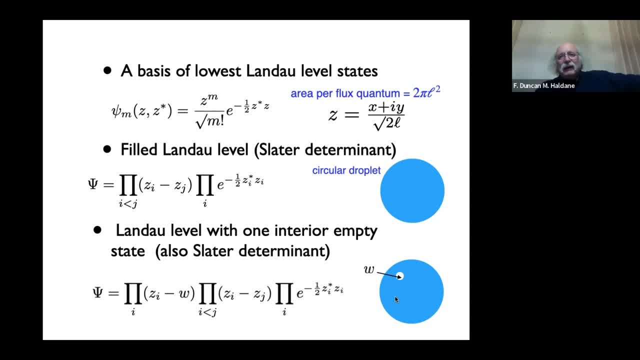 a band structure underlying it, But because the magnetic length, where the regime, where the magnetic area is much, much bigger than the area of the underlying periodic structure, there's almost no sensing. The land orbits don't really feel any change when they're 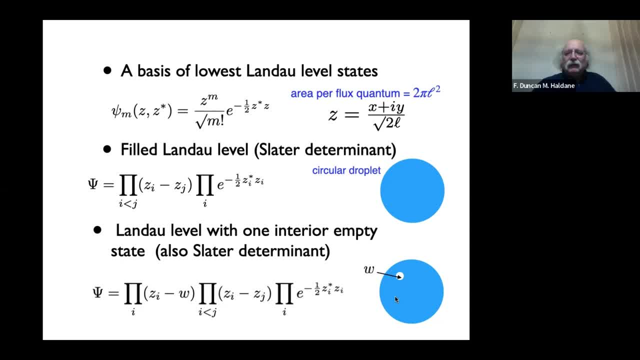 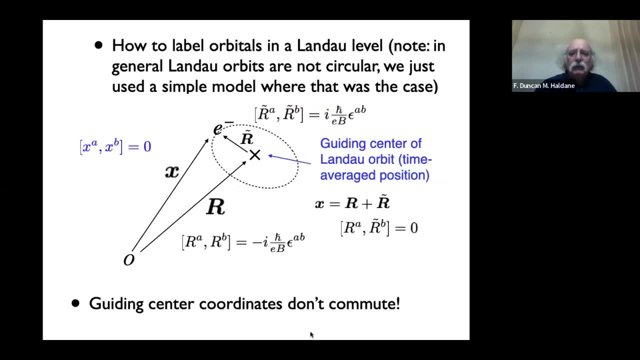 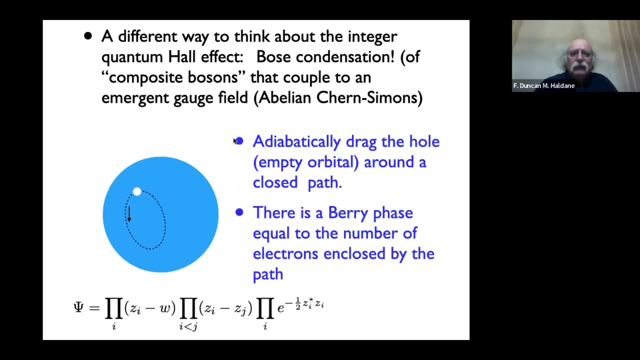 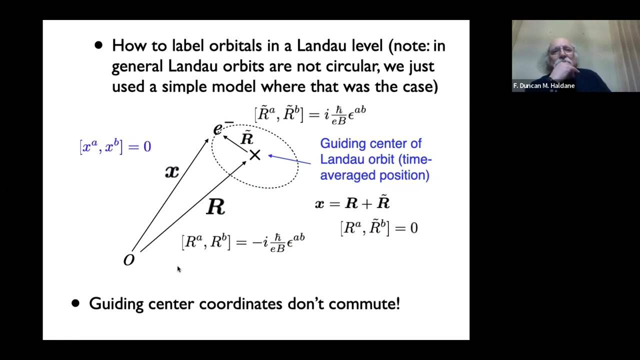 moved relative to the underlying band structure, So you can continuously evolve, continuously move the local orbital around. I'm not sure why this didn't want to advance properly. Yeah, okay, Okay. So how do we, How do we label all those orbitals in the Landau orbit? And here I've drawn a picture. 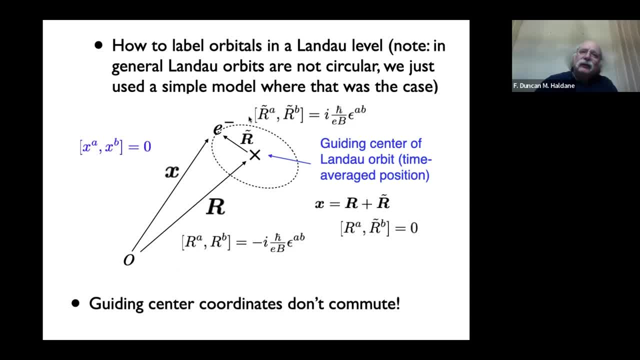 noting again that the generic Landau orbits are not circular, what actually the shape of the Landau orbit is. an image in real space is just, of course, the image rotated 90 degrees of the shape of the orbit in the Brillouin zone around some point. so a closed orbit in the Brillouin zone maps determines the shape of the 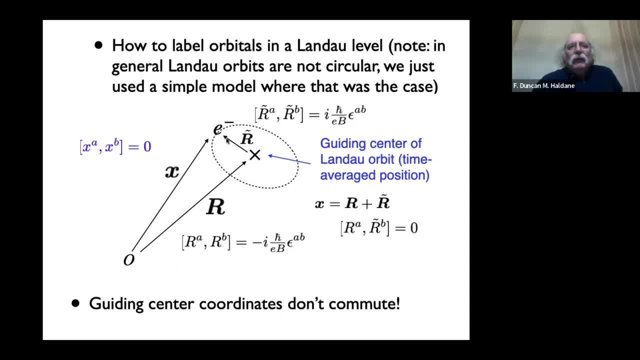 closed orbit in real space and the key point about one key point about uh Lando orbits is they have a center, they have a guiding center and the the key feature in the quantum Hall effect will end up being that the electron coordinate measured from some arbitrary origin can be divided up. 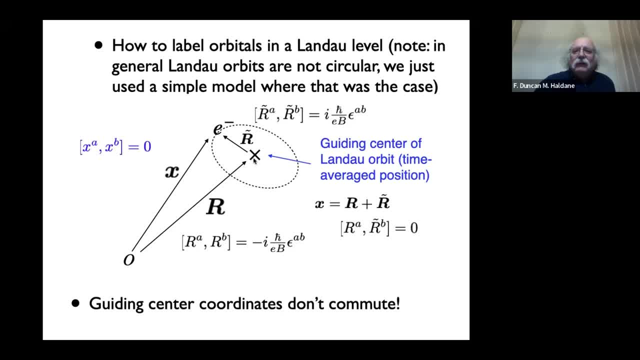 into the coordinate of the guiding center of the Lando orbit plus the Lando orbit radius vector. and the guiding center is defined such that the time independent, the time average position of it's a time average position of the electron. so there's no the the, there is no net dipole moment, no electric dipole moment of the. 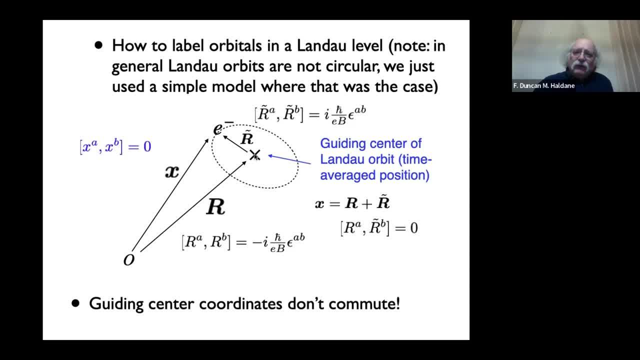 electron relative to its guiding center, but it does have what I'll define some jumping ahead a bit. I'm going to discuss the quadrupole moment now. most people have learned the electric quadrupole moment using the plas equations looking for the expansion of the field at large distances. 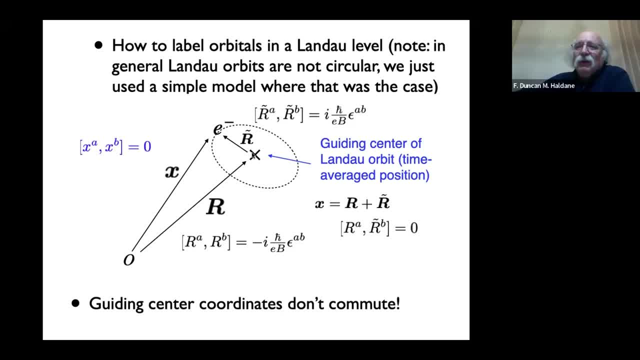 in the point charge and they work with something called the traceless quadrupole moment. but even a, even a circular orbit, has a quadrupole moment. it's not the traceless kind, it's called the primitive quadrupole moment. so the quadrupole moment really is just the, the variation, the 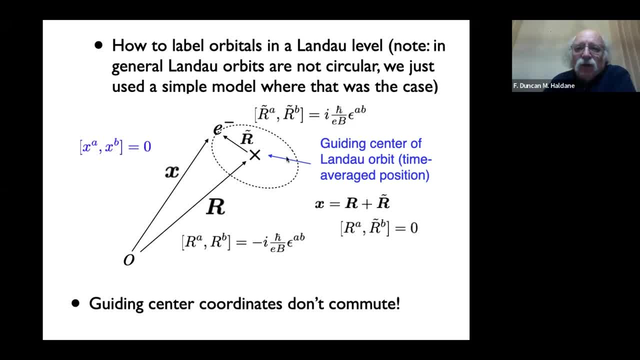 variance of the posit, of the, of the position of the charge is relative to the center of charge, and and so the fact that the, the, the electron distribution, the charge distribution of an electron in a Lando orbit is not a point charge at the center of the orbit, it's actually spread out. 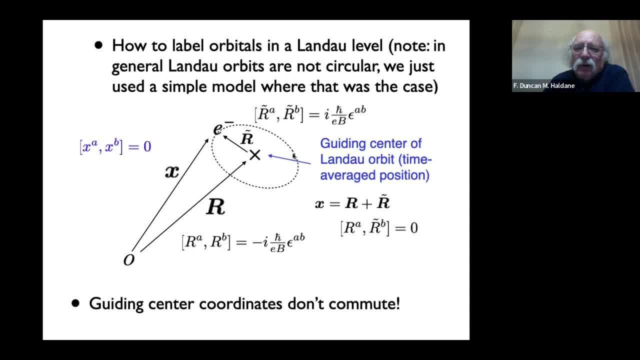 so in the lowest Lando level it's maximum in the center and it's a Gaussian-like shape, but in the higher Lando levels it's a. it's a ring-like shape, right. so the basic feature that the electron density in a Lando orbit is not concentrated as a point charge at the guiding. 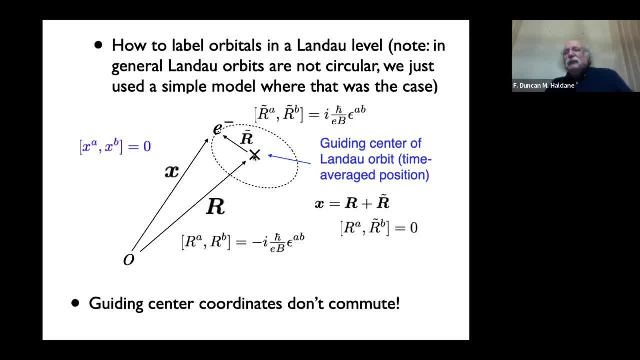 center is going to turn out to be a very important feature which I believe contains has a whole lot of importance in in the, in the quantum Hall effect. okay, so there's. so there's no dipole moment relative to the. so the, the object of the Blasphemy, is not a point charge, it's a point charge at the. 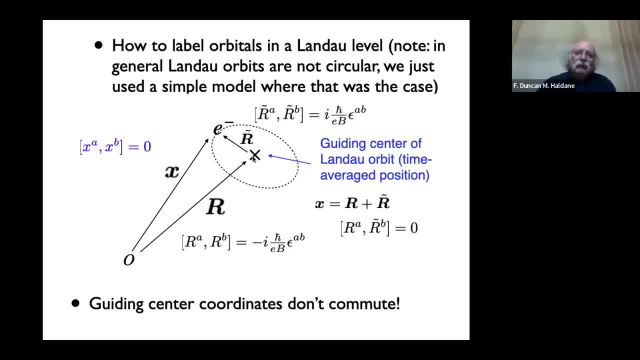 object of an electron orbiting a guiding center has no dipole moment relative to the guiding sensor, but it does have a. the general does have a, a primitive quadrupole moment, and the crucial feature of all quantum hall systems is they have an energy gap for anything that carries electric. 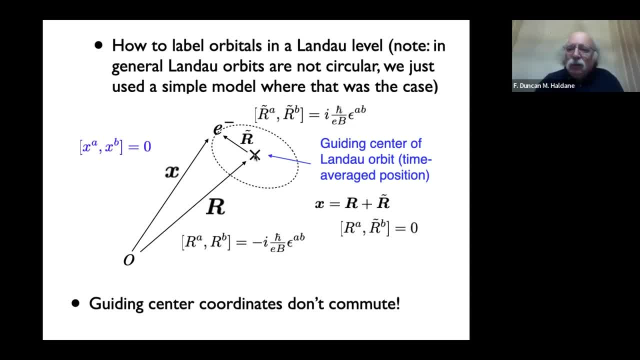 polarization. so they, the energy gap in a quantum hall system is not so much the charge gap, it's actually the gap against polarization. so the there is no in the ground state of a quantum hall system, a uniform quantum hall system. there is no electric polarization parallel to the 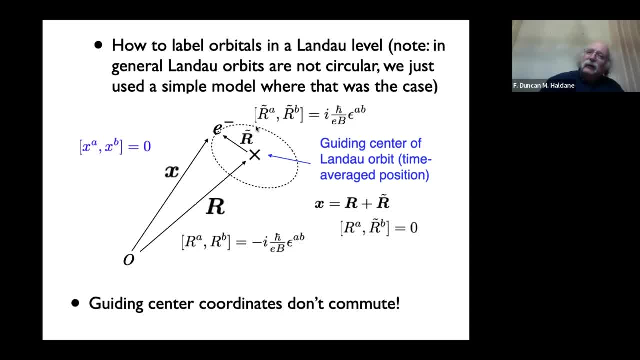 the plane in which the electrons are moving, and that's because the basic entity- say you can see in the integer hall effects so far- is a guiding center with an electron orbiting around it. in such a way there's no net quadrupole moment, no net dipole moment of. 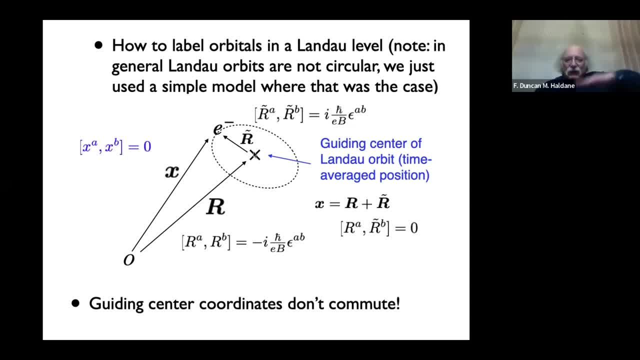 it thing. so to make a, a dipolar excitation in a quantum hall system requires is. is what the energy gap is. uh, is telling you is is restricting you. so the crucial features are going to be that the, the guiding center and the landau orbit. they commute with each other, but individually. 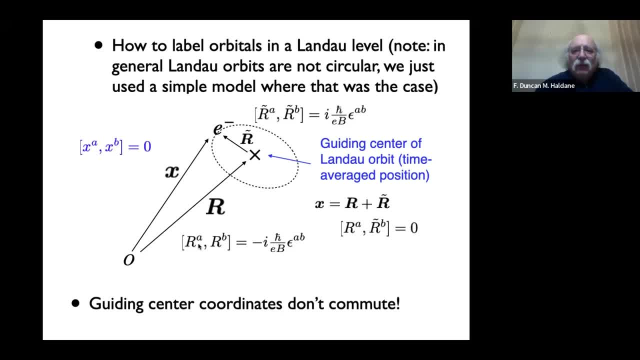 they have. they have a compass, equal and opposite, non-trivial, um chiral commutation relation. so if this one is x times y, is i times, uh, the magnetic length, a magnetic length squared, then the guiding center has minus i times the magnetic length squared. and since they commute, they maintain the correct behavior, that the actual 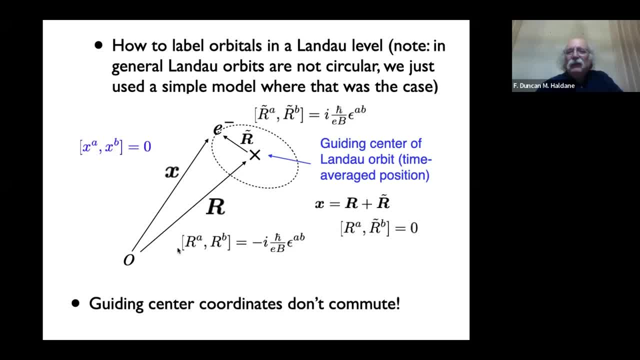 coordinate of the electron has components to commute with each other. so the crucial thing is that that we find that the magnetic length squared is minus i times the magnetic length squared. and, in particular, the guiding centers obey a non-commutative geometry and obey an uncertainty principle that i can't localize. i can't localize the position of the guiding center within an area. 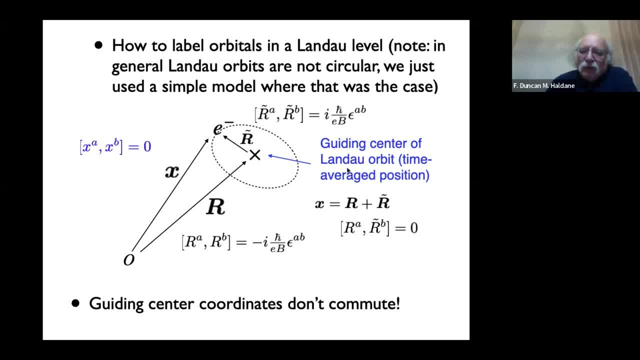 that's smaller than a magnetic flux quantum and the most and the minimum uncertainty principle states have occupy an area of one flux quantum. uh, the shape you can choose a minimal uncertainty state of of any elliptical shape function and you can choose a minimum uncertainty state of any 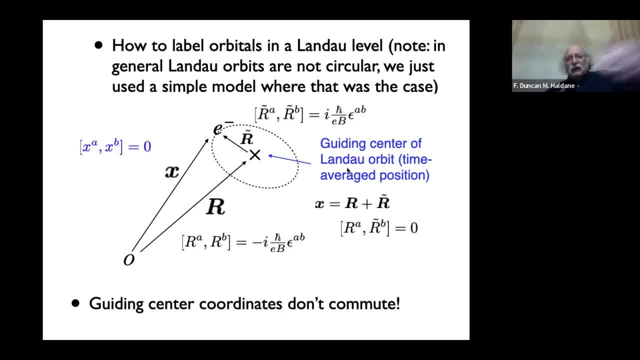 And it's like you can. you can squeeze it in the X direction and expand it in the Y direction. So there's still some choice in what the shape of the minimum uncertainty state is. But those are the most localized. Those are the Landau level analogs of the most localized Wannier orbitals. 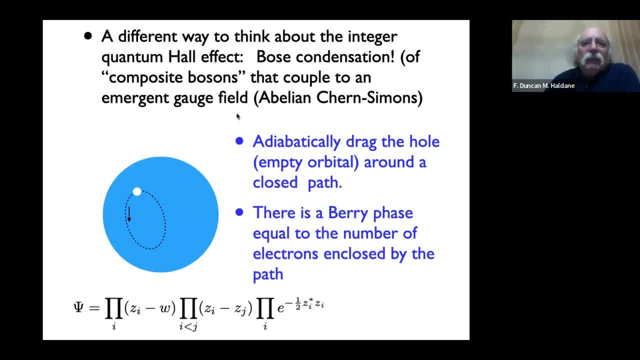 I have to click on something. OK, so this is going to give rise to a rather different way to think about this. The integer quantum Hall effect. OK, yeah, So if you're coming from band structure theory, you might think the most natural way to think about Landau levels is like filled bands right and slated determinants. 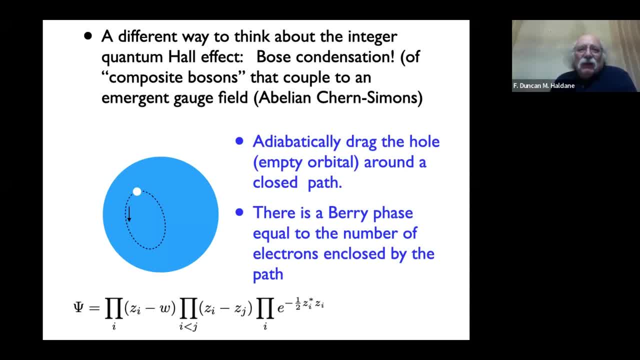 But there's a completely different way to think about the integer quantum Hall effect and think of it as a Bose condensation of composite objects. So this may seem a very complicated, Kind of far fetched way to think about just filling Landau orbitals. 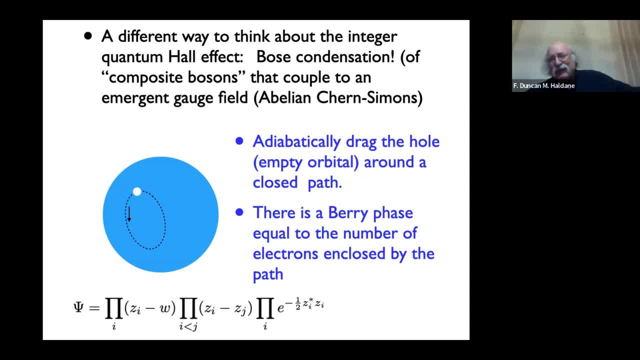 But the nice thing about this is this has an immediate generalization to the fractional Hall effect, while the, the Bose nice version here has a Works in the fractional case as well as for the integer case, even though you might find it's easier to use the free Fermion language for the integer case. So let's imagine we. so now we've got this model for the. 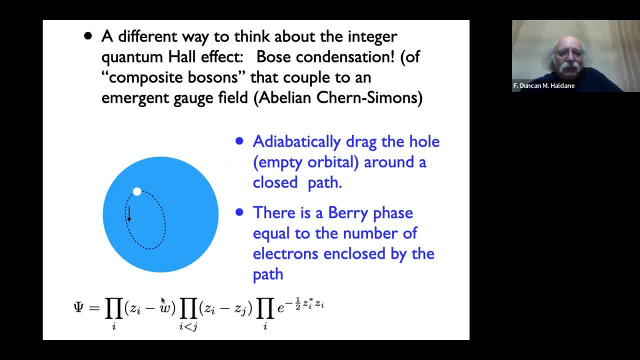 But for the quantum Hall effect was a single hole in it. So let me drag the single hole around the closed loop. The crucial thing here is that I can, idiom, cannot actually move this localized hole. Well, I couldn't intellectual move the localized when the orbital in the lattice. So this is a fundamentally different feature of lambda orbitals from block bands. 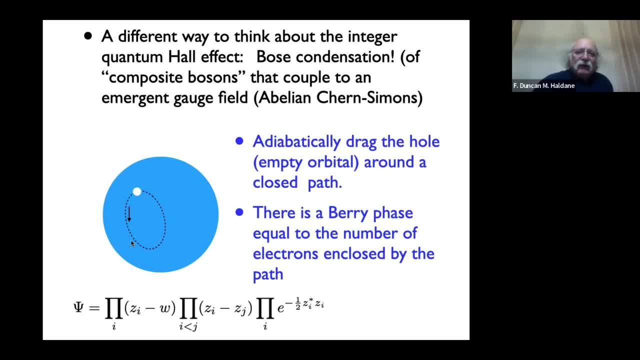 So I could, if I dragged the clothes, the mtl, the empty orbital around the closed loop, around the closed path there's going to be, there's a berry phase and if we look at the thing, this is like a little vortex. so the so if omega, if w goes. 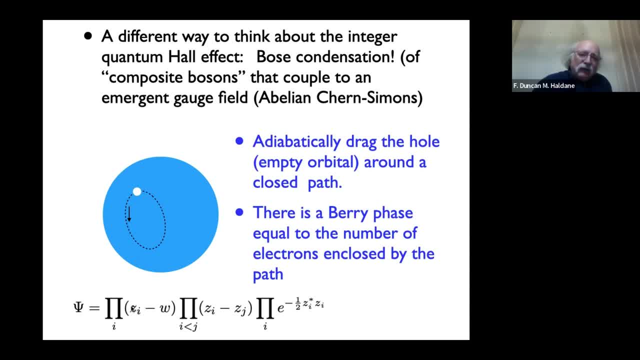 around a closed path. it picks up the wave function, picks up a phase of two pi for every electron cordon that the w encloses, the path of w encloses, and it doesn't pick up any phase for the ones which are outside the path, and that's of course the berry phase. so if i move this orbital around, 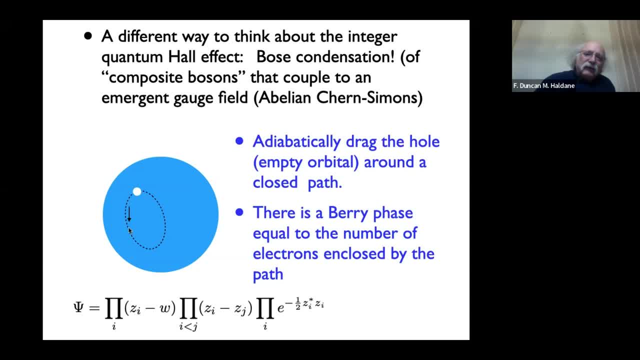 the empty orbital, all the orbitals in the, all the filled orbitals. the basis of filled orbitals in the slater determinant has to change, because they have to be orthogonal to the or they have to essentially be orthogonal to the um, the empty one, i'm moving around. so this is why. 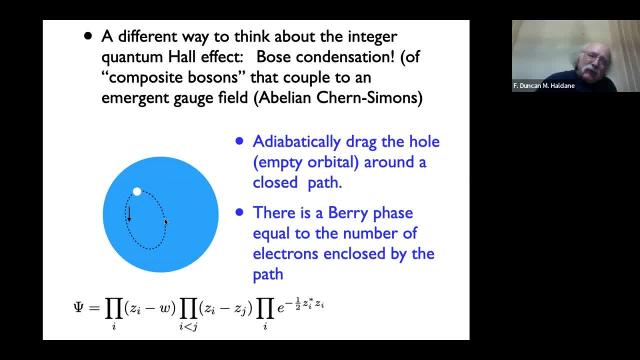 the state of the system is changing and i'm picking up the very phase when i move this around the closed loop and of course the berry phase is equal to the number of electrons enclosed by the loop. this is the arova schriefer wilczek argument. 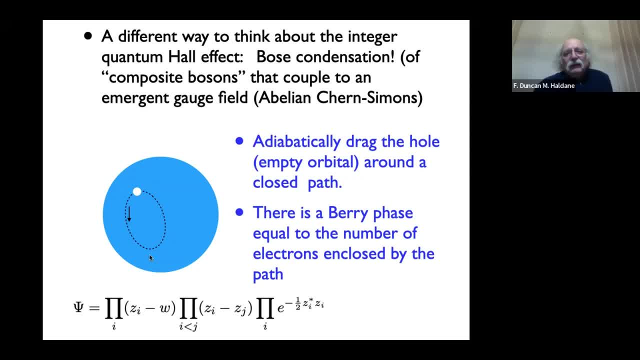 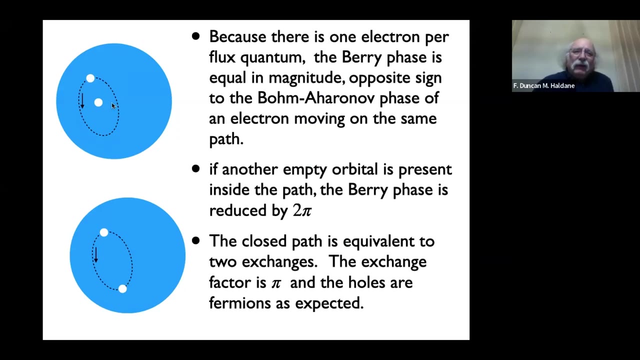 so the, the very phase, is equal to the, in this case- number of electrons contained in the loop. but since, or two pi times that, but since there's one electron for a reflux quantum, the very phase you get is, of course, equal in magnitude and opposite in uh, in sign to the boma horonoff phase that an electron would have if it was. 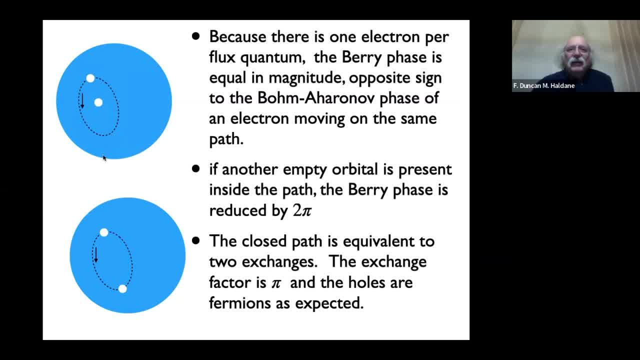 adiabatically moved along the same contour. and of course then we find that suppose there's an another empty orbital inside the the path. then the berry phase is reduced by two pi relative to what it would have been if that orbit empty orbital hadn't been there. so then 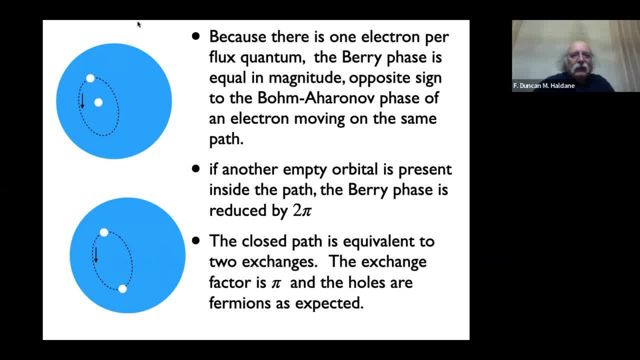 if we look at the uh, think about the exchange of this pair of things. these are, these are basically identical objects, these empty orbitals, uh. so if i exchange a pair you can, you can see that actually, a single double exchange is essentially equivalent to going around the closed path. so so a single. 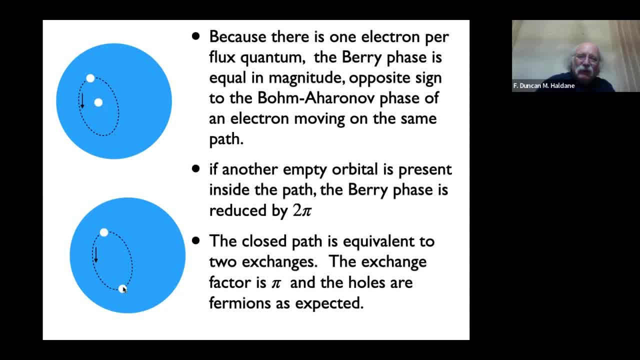 exchange picks up a factor of pi in the wave function. if i do it twice, i get back to where i started from it. so, like i, you know, what i do is it's just. once it's square and two hand training it 's. this is the um wave function, then this is the derivative. it's possible, it's just. 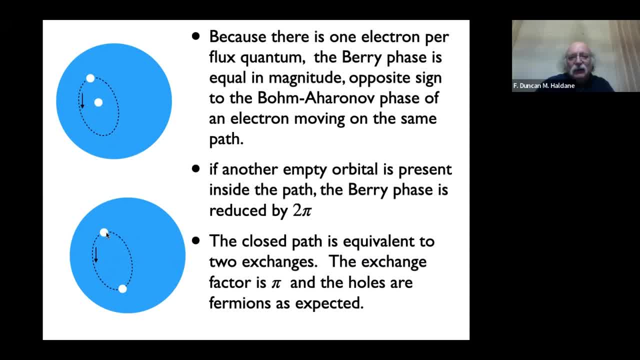 two pi, it's two pi. uh, in addition to whatever the phase is worth, from the, the berry fields, the boma, horonoff, light worn sa introduced here compensating fields. so this, this is of course telling you the that, as one expects that the holes in the 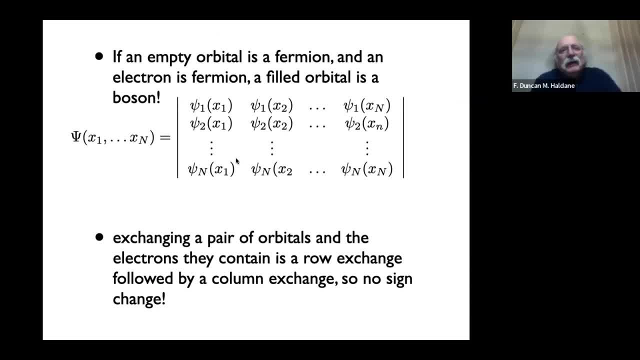 lan investments. How doesFirstenza laver level? they behave as fermions, you two means that if an empty orbital is a fermion and an electron is a fermion, then a filled orbital is a boson, And indeed the filled orbital is what one can view as the composite. 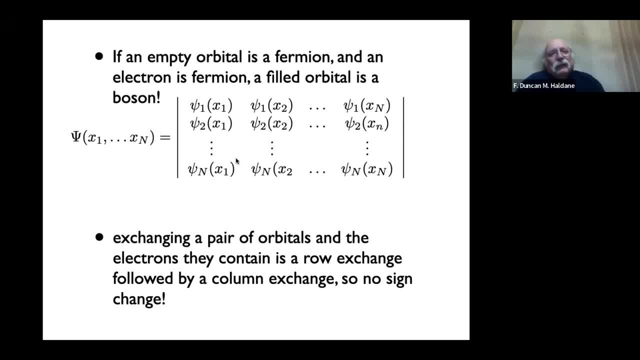 boson in the picture of the integer Hall effect. So if we think about it, let's look at the Slater determinant again. I'm swapping two filled orbitals. I'm swapping, which means I'm swapping two orbitals, I'm interchanging two rows of the Slater determinant and I'm 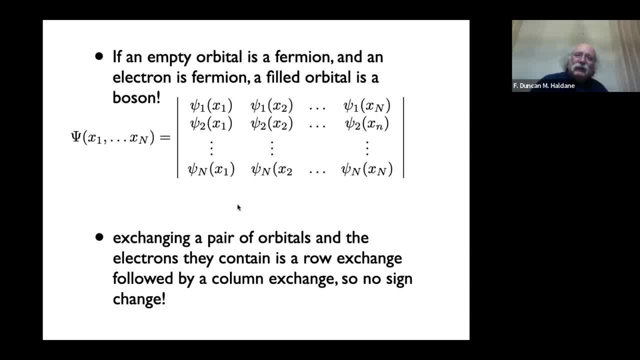 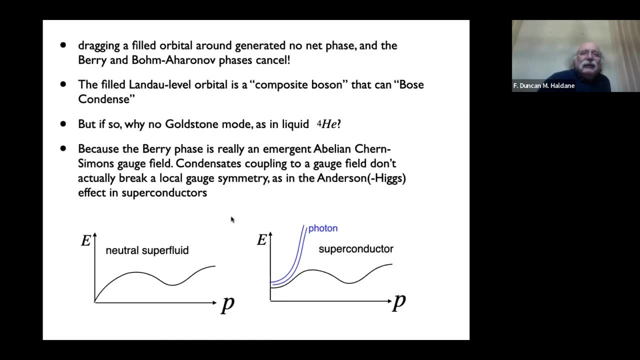 swapping two electrons, which is two columns, of course. so there's no sign change. So, indeed, exchanging a pair of filled orbitals is a bosonic process. There's no sign change of the ground state. So the And because the Berry phase and the Bohm-Horonoff phases cancel dragging a filled orbital around, 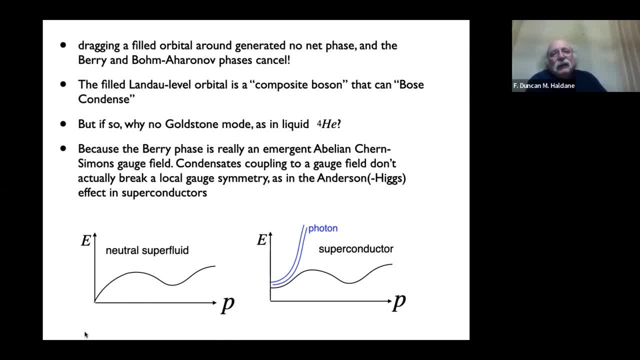 generates no net phase. So the filled orbital has no phases as it moves around and is bosonic, which basically means it can both condense. But if it can both condense, you'll ask you know, why is there no Goldstone mode? We know in liquid helium form when it both condenses. 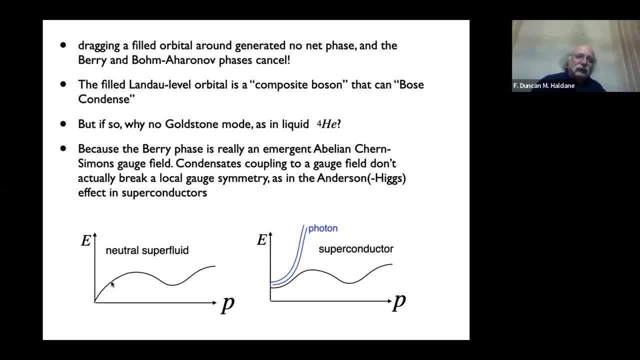 we get this linear dispersing sound wave mode which is the Goldstone mode of the Neutral Superfluid Helium 4.. And you see the same thing in atomic condensates now. But the Berry phase in this problem is actually an emergent abelian Chern-Simons field. It's not the Bohm-Horonoff. 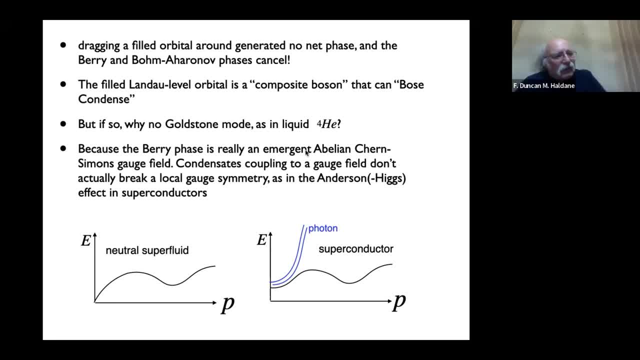 phase, although it's similar to it because the But the Berry phase, the Bohm-Horonoff. the Bohm-Horonoff is actually an emergent abelian trans-simons field, So it's not the Bohm-Horonoff phase, although it's similar to it because 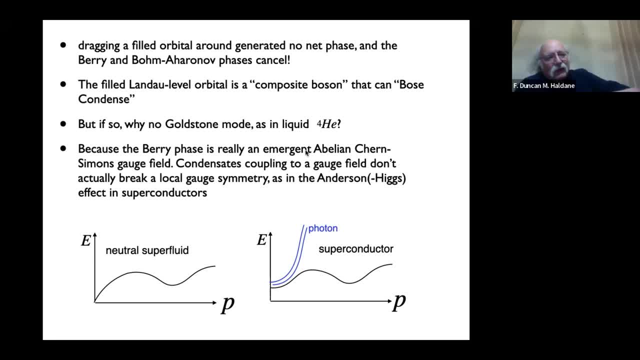 the the Berry phase is generated by a purely two plus one dimensional source. right, It's coming from moving this electron around in the background of other two dimensional electrons in the plane, So it's a distinct emergent gauge field which is purely two plus one dimensional, as opposed to the. 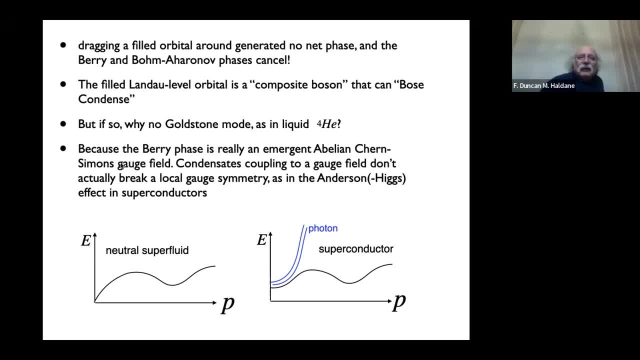 three plus one dimensional electromagnetic field. And of course we know that from Anderson that if a Bose condensate couples to a gauge field, in the case of superconductivity the electron pairs are charged, so they couple to a gauge field. 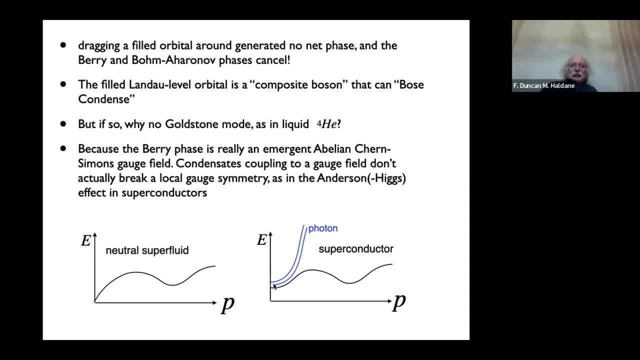 then the Goldstone mode of the neutral fluid interacts with the gauge field and becomes gapped. So in a superconductor, the sound wave of the condensate, which would be linear if it was a neutral, it would be a longitudinal phonon mode if it was a neutral fluid. 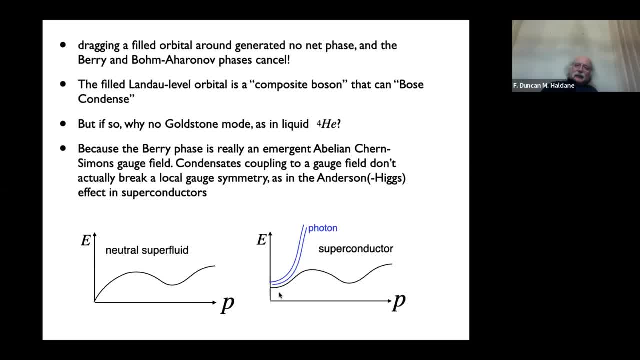 becomes the plasmon, it's gapped And of course in a superconductor. the photon is gapped inside a superconductor and the gauge process, of course the means. that is basically what eats up the Goldstone mode. So technically there's no true local gauge. symmetries can't be broken. 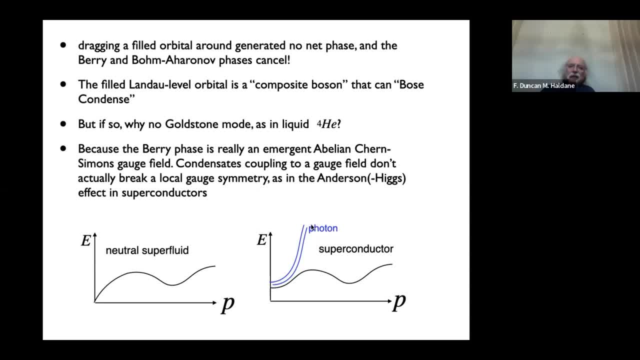 And so there's actually no broken symmetry in the quantum Hall effect, But the gauge process which in the superconductor is coupling to the electromagnetic field in the quantum Hall, is the gauge coupling to the emergent— John Simons field which removes the Goldstone mode. 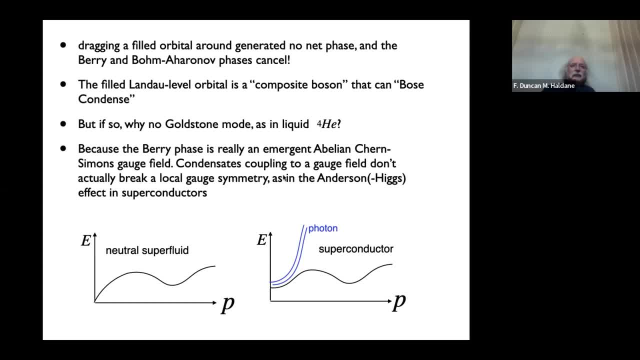 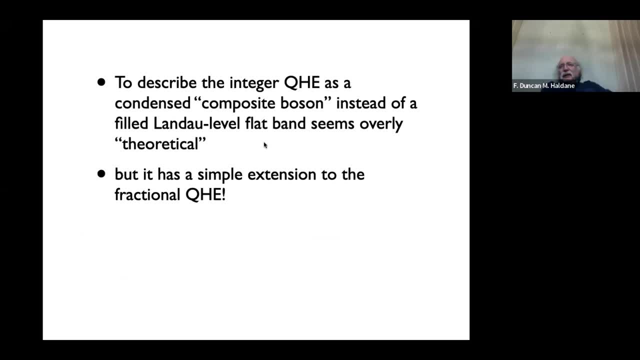 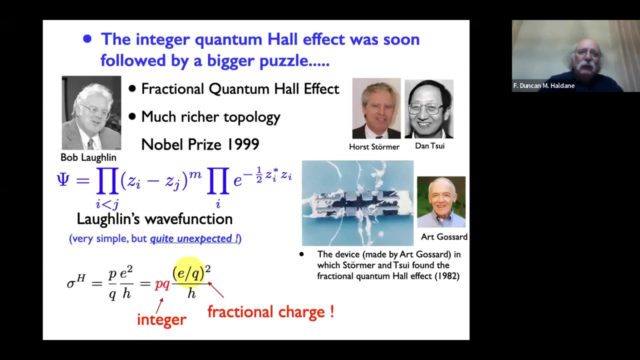 that you might expect if you had a simple Bose condensation. Okay, so describing the integer quantum Hall effect as a Bose condensed composite boson seems like a very kind of far fetched theoretical thing, but of course it has a extremely simple generalization to the fractional quantum Hall effect. 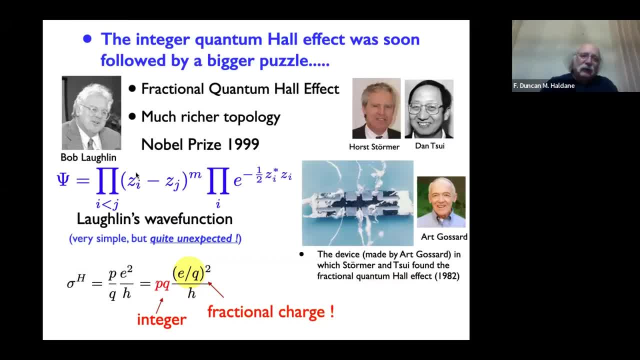 Okay, which of course is also Loflin's achievement, And of course we're dealing with the Loflin wave function, And okay, and we can write: the quantized Hall effect in general replaces integers by other integers. In fact, as we'll come to it, let's see. 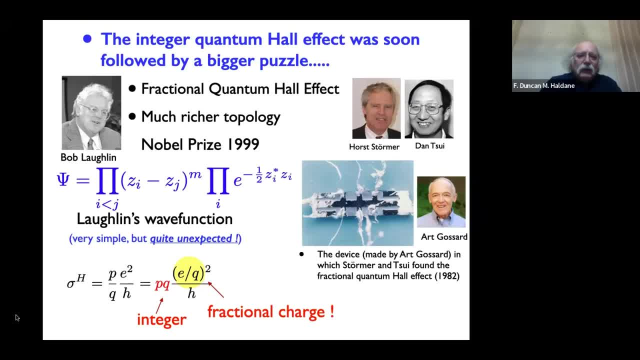 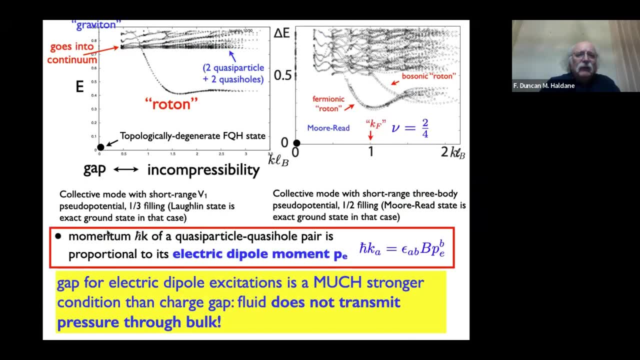 Okay, so anyway. so we're going to. we can rewrite the whole, we rewrite the Hall effect in various different ways and integers. So first to remind you what we can, what happens when you look at these problems numerically, by numerical exact diagonalization. 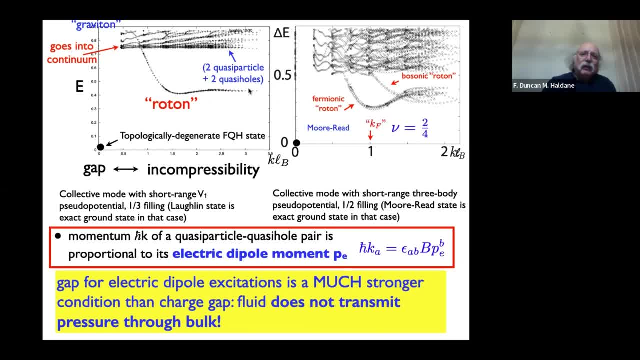 this is a diagonalizing, a toy model problem, for which the Loflin state is the exact ground state And we see that there is a along. the bottom line is essentially momentum. It's also equivalent to electric polarization. So because in a magnetic fields 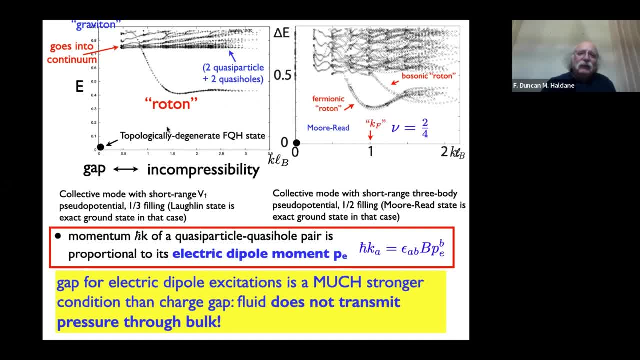 the momentum. electric dipole in a magnetic field has a momentum, So momentum is the same thing as polarization. The relation is the magnetic flux density times the dipole. moment is equal to momentum And it changes. It checks out with the right units. 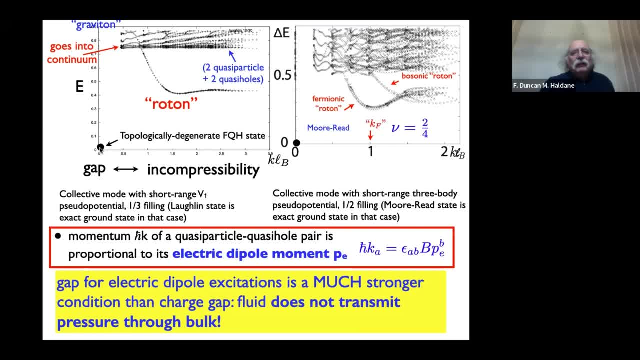 So in the quantum Hall effect, if you, certainly if you do it with periodic boundary conditions, on a Taurus, you have the famous topological degeneracy which comes from its topological order And there's a ground state, always occurs at like zero momentum. 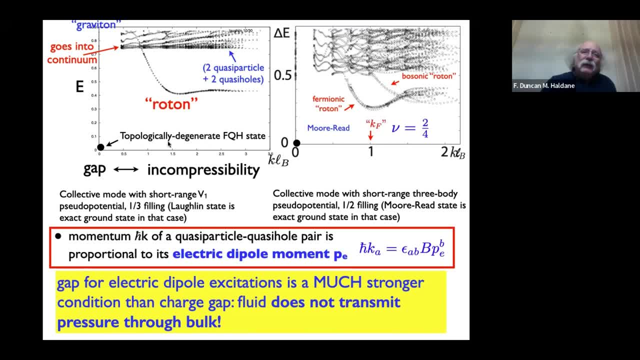 And there are no other states that low energy momentum, because all other states with finite momentum have a electric polarization. They carry electric dipole moments And there's a gap for that. Here you see, the lowest excitation is a pair of a neutral pair. 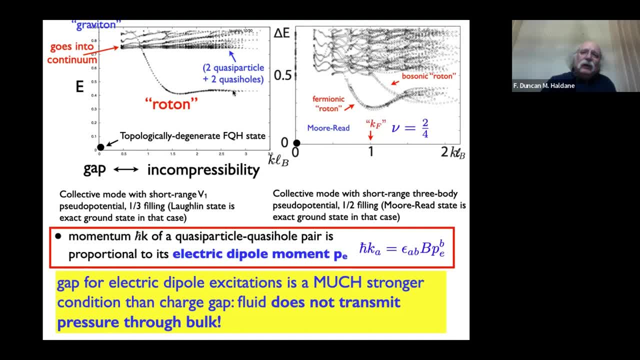 of positive and negative quasi particles which are spatially separated. So the separation turns into the momentum at large distances, While at long wavelengths we see there's something, a mode which will come up here, which this slide calls the graviton, but I will 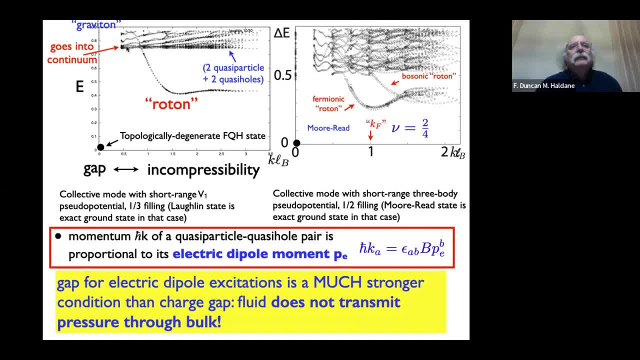 I will explain what I, what I, what I think. it is later And there's a continuum. This is the more read case. This is a non-abelian quantum Hall state. Again, this is the absolute diagonalization of an exact model which. 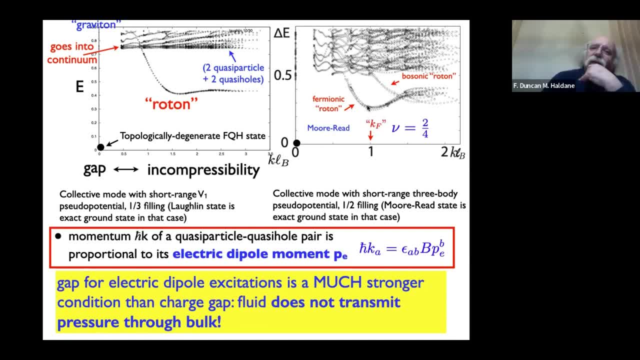 for which the more read state is is the ground state And then the more read state, the quasi particles have basically carry Majorana zero modes and the quasi particles have basically carry Majorana zero modes. So if I bring two of them together, 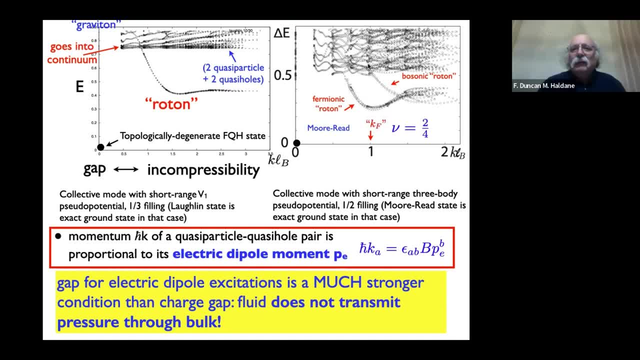 they can either come together as a fermion, which is this branch, or they can come together as a boson, on this branch, And when they're widely separated you can't tell whether they're fermions or bosons. The fermion parity is hidden in the entanglement that they leave behind. 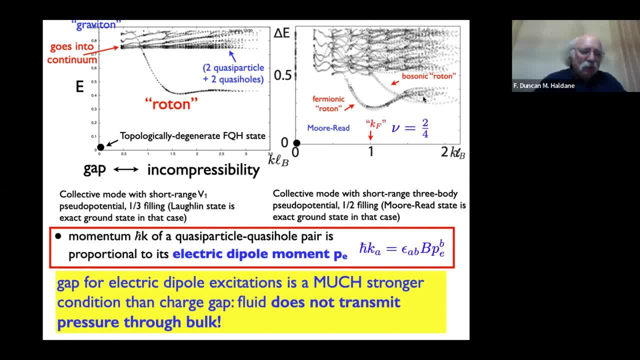 And that's the, that's the simplest form of the entanglement that people hope to use, But the Microsoft in particular hopes to use for for quantum computing And again. so we see again the feature that there's an energy gap for anything with electric dipole moment. 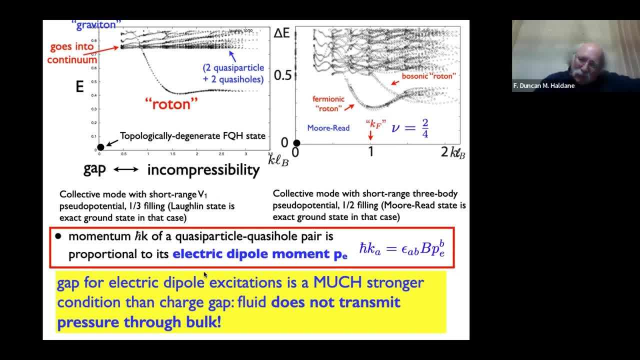 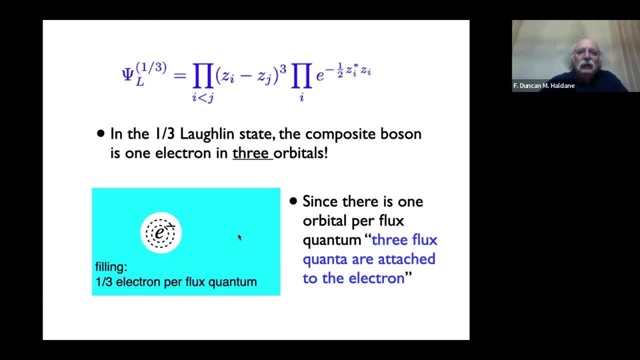 which will turn out to be why there's no dipole moment, but the fluid carries this quadrupole moment. Okay, Okay, So in the Laughlin state the composite boson is one electron, not in one orbital, but in three orbitals. 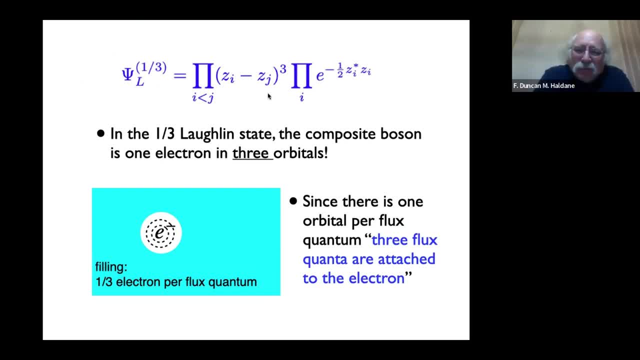 Okay, So it's definitely not the Pauli principle behind it, right? The Pauli principle says: one elect, you can't put more than one electron in one orbital, And so the you can say then, in a Slater determinant, the electron. 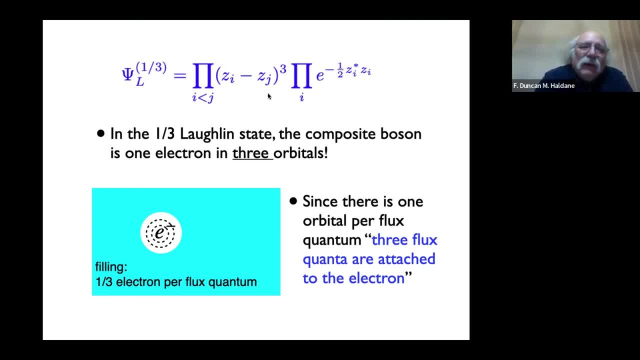 the electron owns the orbital which it occupies. But in the Laughlin state we now took the Slater determinant state and put a three here. So basically, if I think of this, so actually this electron number one is sitting in a side three hole where none of the other electrons come. 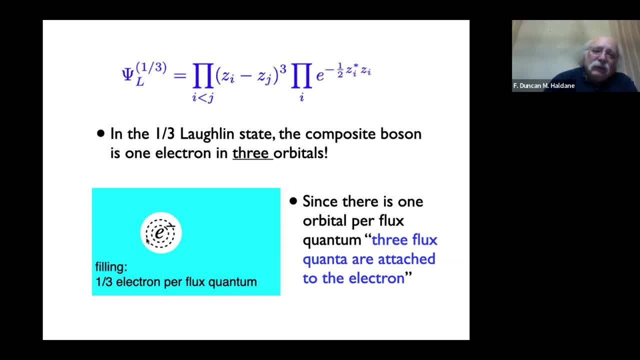 None of the electrons come closer to it than outside the side three hole. So in this case we have an electron that's sitting inside a little void, a little bubble- I've drawn it as a circle- but it actually the energy is going to determine what the actual shape of that. 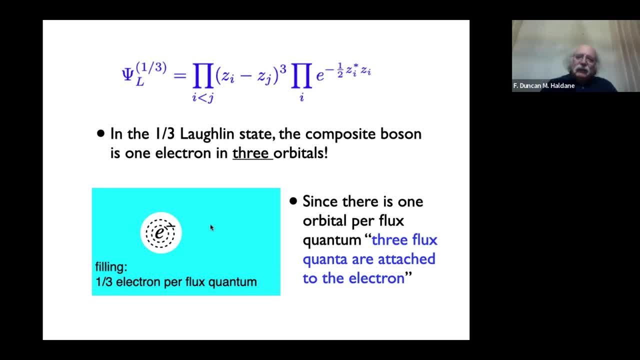 that that little bubble is, And but the language which was initially come, adopted from Chern-Simons abstract. Chern-Simons theory is that flux gets bound to particles, But the magnetic flux, of course, is not bunched up into little flux tubes. that binds to particles. 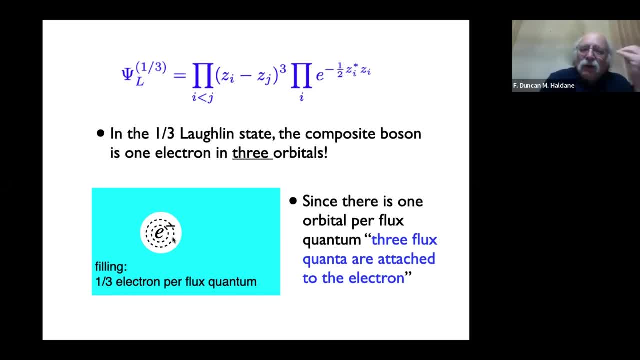 What we really mean by flux attachment is there's one electron orbital per flux quantum. So what if the electron is owning three orbitals rather than just one? then three orbitals, which means three flux quanta, are attached to the electron. So the flux quanta in flux attachment are electronic orbitals. 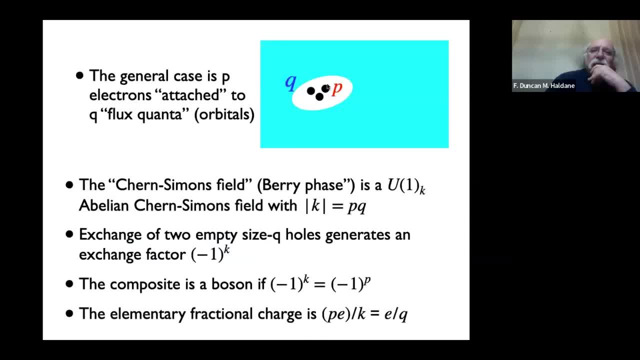 Okay, And the general case is when P electrons are attached to Q flux quanta. So we can look at the same thing. We can look at what the, and I've drawn it as an arbitrary shape because the, if, the, the potential. 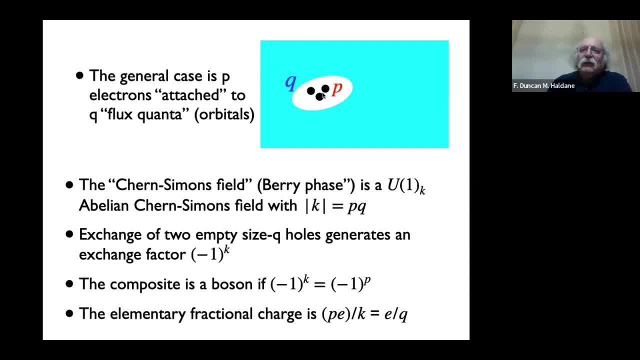 because it's the Coulomb potential that is going to stabilize this structure. It's because the electrons in the interior of the little void can can squeeze up into the middle to get as far away as possible from the other electrons which are outside the bubble. 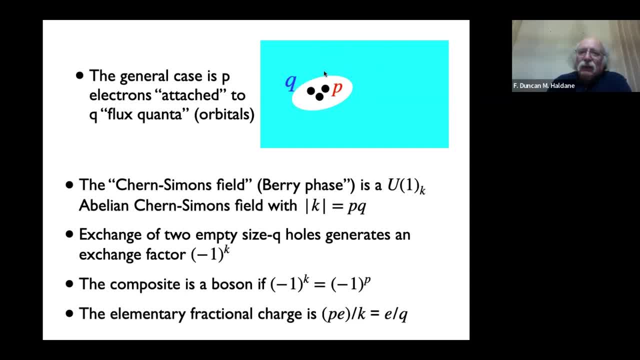 So the bubble keeps all the other electrons away from them, And so the by, by putting the charge, concentrating the charge in the central region, then we can lower our energy. Okay, So the first thing is to know what is the phase I get for interchanging empty voids. 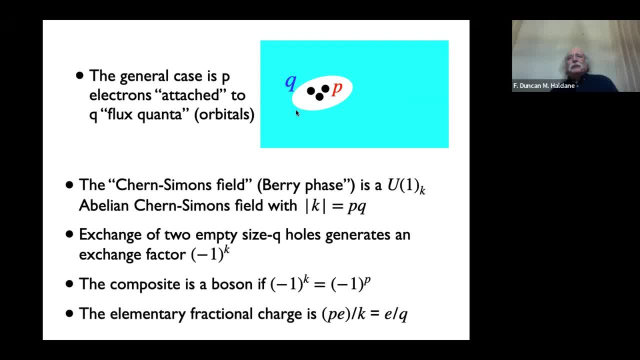 right. So we've got a phase factor when P was when Q was equal to one. we got a phase factor of of pi for interchange Here and we interpreted that as the charge when Q which this was equal to one. 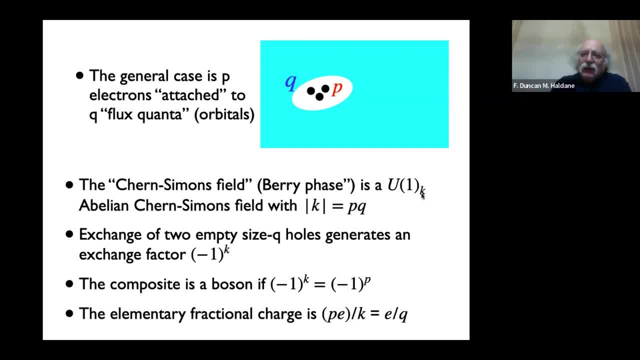 then how does this exchange the charge of of pi And what a? what does that mean if you think about an energetic proposed linear network? So this is the, this is the energy, this is the energy. this is the energy, the energy that's going to communicate, the energy that's going to. 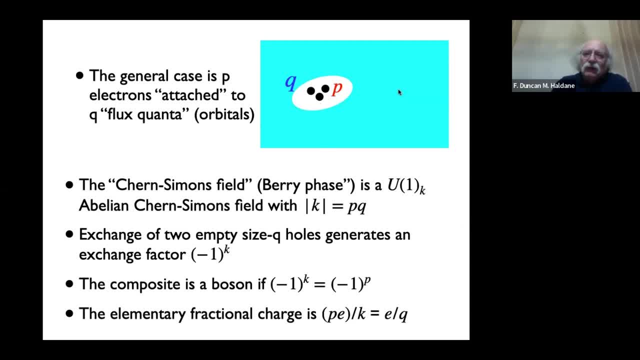 that's going to, that's going to face the energy into a, into the energy that's going to go into the electric field, And then this energy blah, blah, blah, because this is like q vortices. and then the background filling factor is p over q, so one 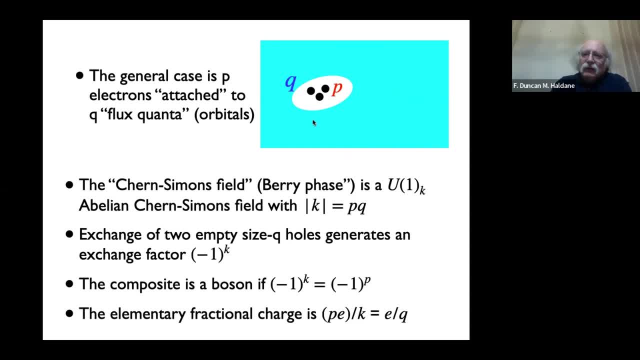 can work out what the what, the phase factor for two of these guys interchanging in exactly the same way as one did it for the naive filled lambda level case, and the phase factor is minus one to the k. okay, let's go back again. and so k has to be an integer, so the. so one of the things 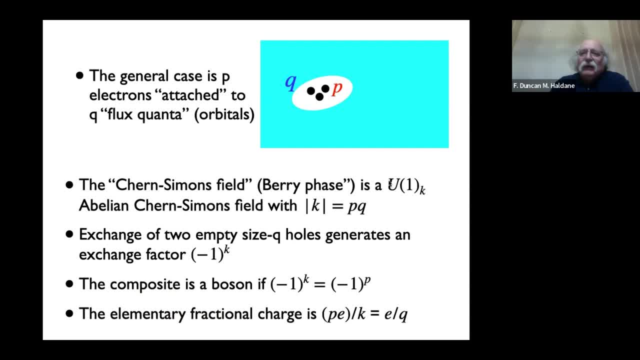 in chern simon's theory is that if it's a gauge, if it's a, if it's a, if it's a, a lee group valued theory, then there's a whole lot of stuff from the, the um, the structure factor of the lee algebra, that determines quantization. in the abelian case, the quantization is provided by the condition that 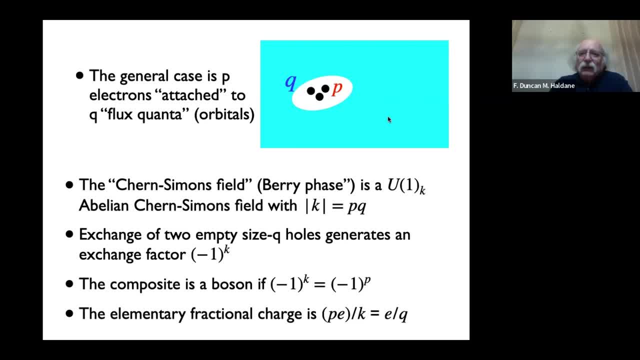 the, the basic object, the two basic objects have to behave like regular statistics. they have to have either a plus one or a minus one factor under interchange. so the void is a boson if k is even and is a fermion if k is odd. so if i want to make the composite object with electrons in it, 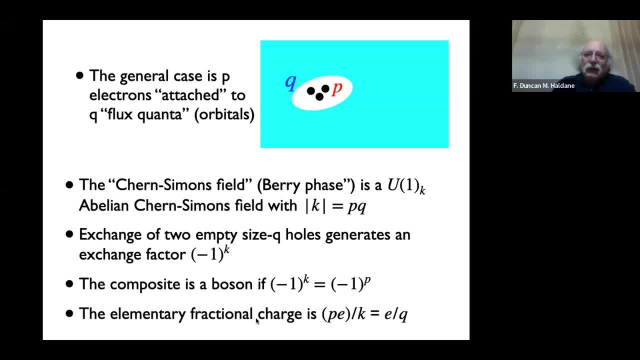 i want to have the total object to be a boson and i get the selection rule that minus one to the k has to be equal to minus one to the p. so, uh, the filling factor is p over q and originally people used to think that the, the, the two numbers in p over q, had no 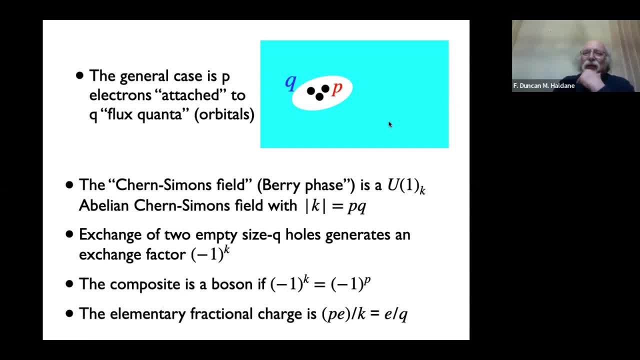 factors right. so p over q means p over q equals a half means p equals one and q equals two. but that violates. if p equals one and q equals two, then k is equal to two and p is equal to one. so that violates the both, the condition that there are a boson and indeed 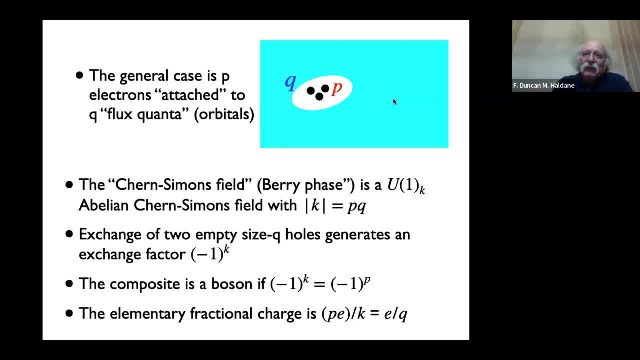 for the filling state at one half of a landau level, if in which is seen in the second landau level, at five halves, q is four and p is two. so there was a big mystery and and the ones and it and if you uh make, if the basic object can't be split up into into, into is not, it's, is not. 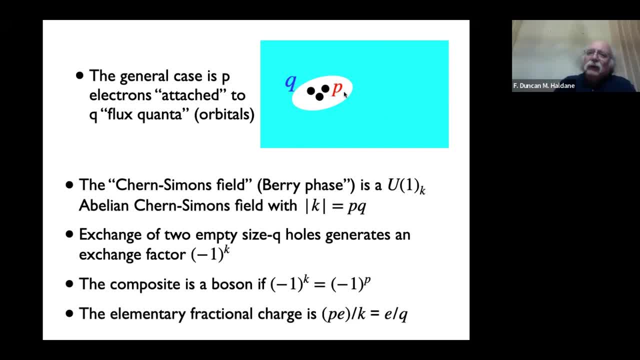 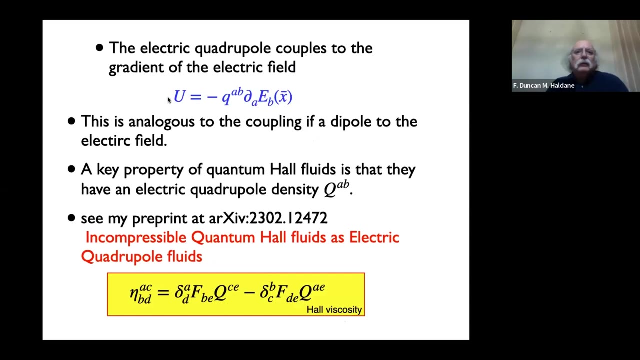 itself factorizable into bosons, then the ratio of p and q can either have a factor of one or two um. okay, so two over. so a half filling state of electrons has to be a two: two particles in four orbitals to satisfy the rule. okay, okay. so let's have a quick. let's go back to 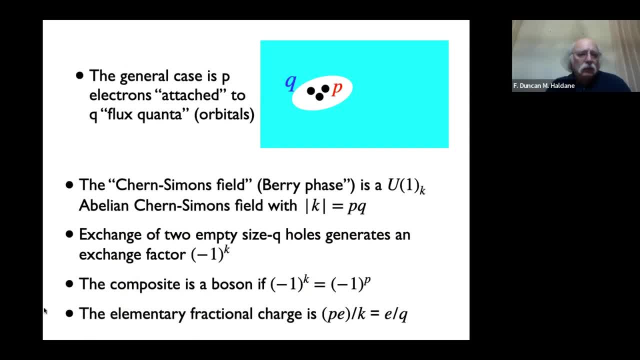 let's see. okay. so the other thing is that the elementary topological charge to excitation, which was still one electron plus or minus e in the integer hall effect, is in general um if a factor one over k of the charge of the composite boson. so this: 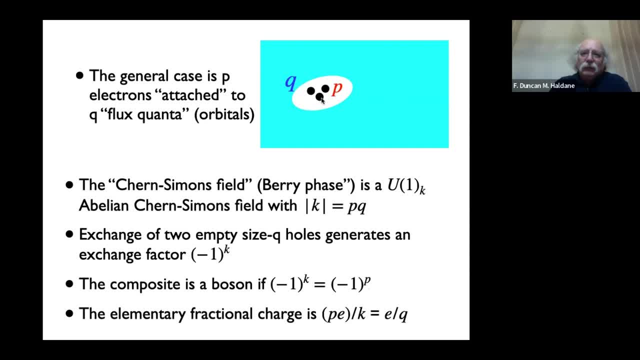 composite boson has a charge of p times e and for the Chern-Simon theory, uh, kind of the elementary vortex is the kind of flux quantum associated with charge p, e objects and uh, so that allows you to form elementary charged objects which are p, e over k, the Chern-Simon's index which is e over q, in this case. 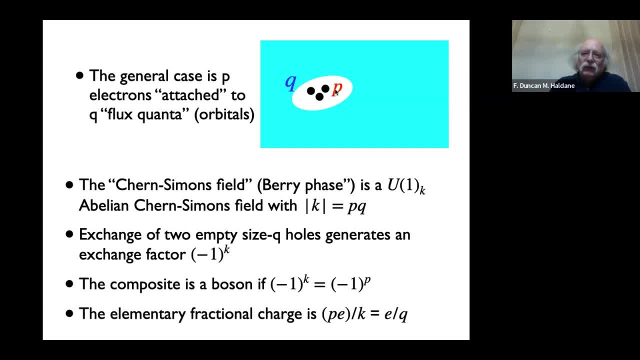 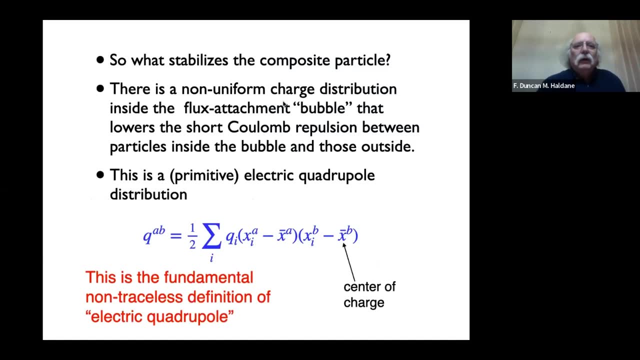 so, indeed, in the one half case, which is really um, q equals four and p equals two, the elementary charged excitation is an e by four, excitation, which you know some nonsense, okay, so another aspect. so the question then is what energetically stabilizes this composite? 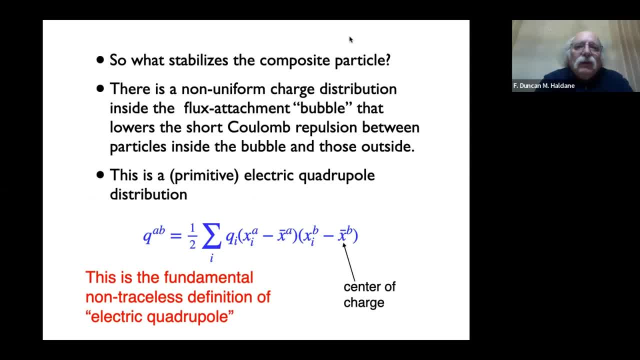 particle, and this is probably some of the new features. so there's a non-uniform charge distribution. as i said, the fact that the what stabilizes the distribution is that you put the uh electrons close to the center of the droplet to keep of the bubble, to keep them away from the stuff outside the bubble, and that's what i call a primitive. 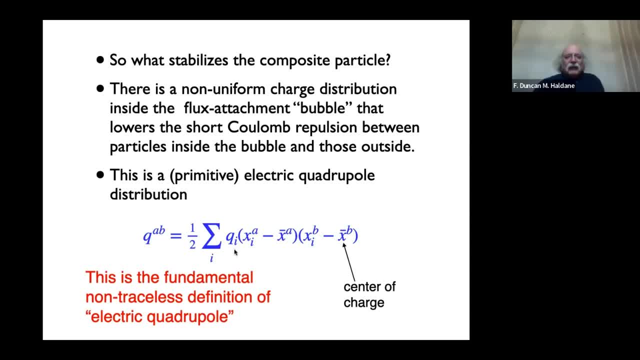 electric quadrupole distribution. this is the the correct definition of electric quadrupole. if you look on the on the united states nist site, national institute for science and technology, there's a very interesting uh tutorial on the quadrupole and most people have only learned. 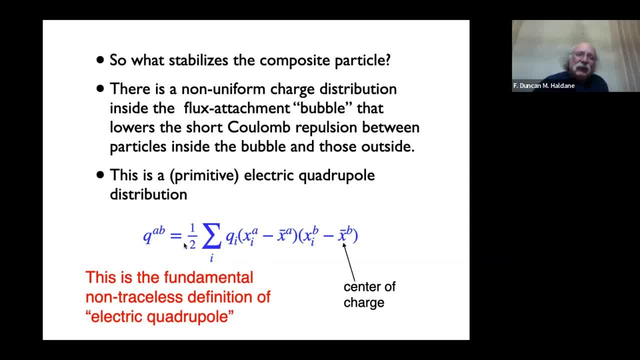 the traceless quadrupole. they're actually. there are actually four, four possible definitions in sight which are floating around in the literature. there's a question about do you use the traceless or the primitive form and do you use the factor of one half here? right, and what i 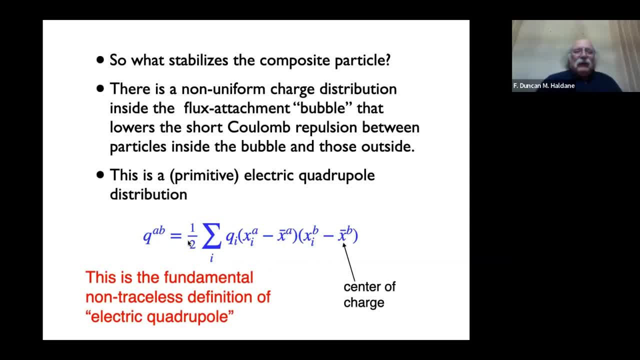 believe is the. the correct definition of an electric quadrupole is the least popular of those things. the factor. to use the factor of a half is the least popular choice, and to use the primitive rather than traceless form is the uh also the least friendly force. so you can see that this object has two upper indices. i've written my 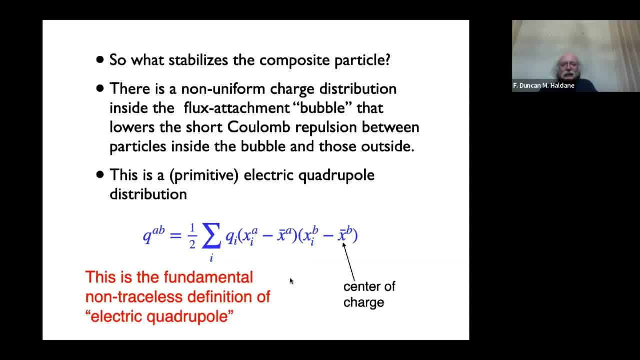 indices of my coordinates as upper indices, and if i want to write a different, a differential, it has a lower index. i'm separating covariant and contravariant indices. if you have rotational symmetry with a metric around, you can, uh, of course, raise and lower your indices to your 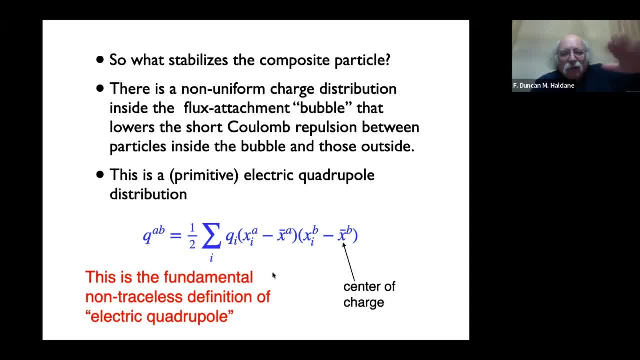 heart's content, but you're. but you're hiding the fact you're using a metric. but if you don't have rotational invariance, you actually don't have a metric. there's actually no place for a euclidean metric in condensed matter physics, except in one. 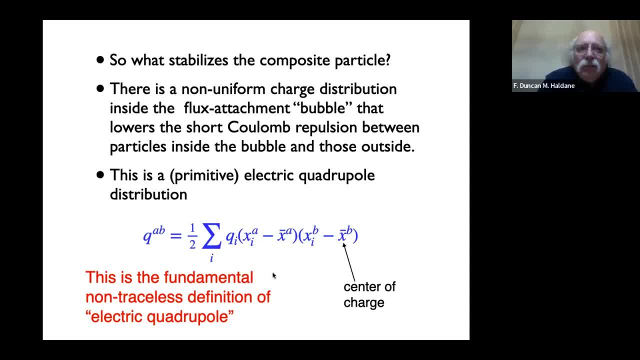 place? uh, there's no rotational, no continuous rotational symmetries in solid state physics and crystalline physics. and the only place the euclidean metric enters is that the, the, um, the nuclear, the nuclear cause, the, the. the nucleus of the atom essentially has a mass tensor which is given by newtonian. 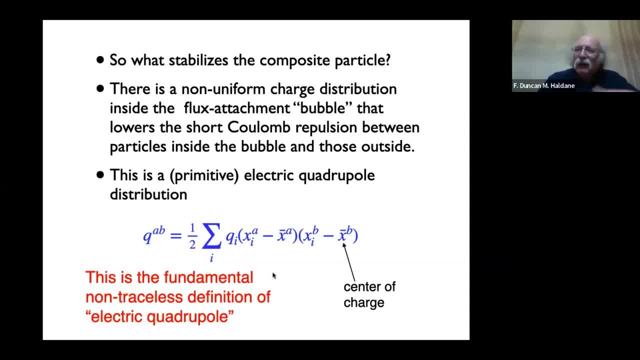 mechanics, the electrons don't. the electrons have have block band structures. they're not newtonian particles, they move around in the block bands but the, the only place but the, the nuclear coordinates have, uh treat, have, have a mass tensor which is given by their, their bare mass or 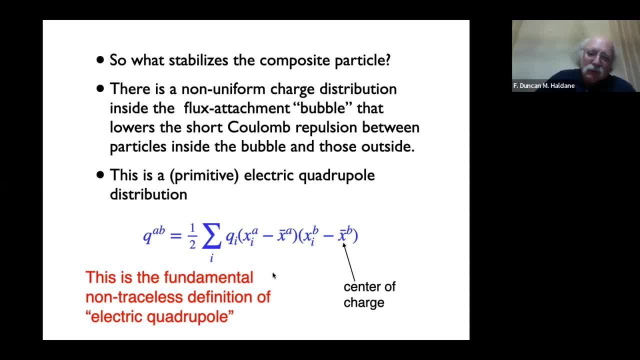 gravitational mass times, the, the, the euclidean metric, which is the, the equivalence principle, and uh. so phonon dynamics contains, through the, the kinetic energy of the nuclear coordinates, contains the, the euclidean metric. there's absolutely no other place in condensed matter where the euclidean metric has any any role. 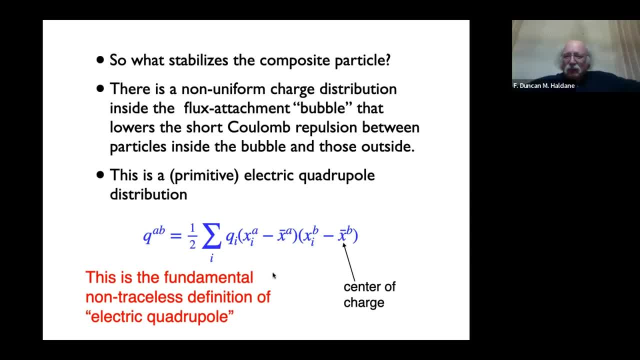 so the only place for euclidean metric is actually the laboratory frame, the, the, the empty, the, the vacuum frame, or the, the laboratory frame of the laboratory in which you're measuring the thing. so euclidean metric is only used for setting up a coordinate system, so it should not enter in any physical equation if it's. 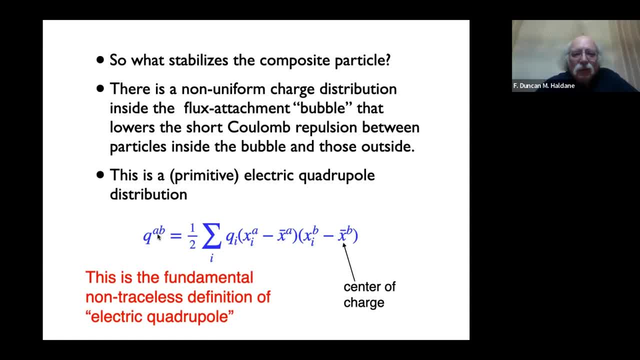 not phonon dynamics. okay, so the the actual traceless form is you subtract off the part of the quadrupole which is proportional to the dielectric tensor. okay, so any part of the quadrupole if there's a quad, if the charge is to be. 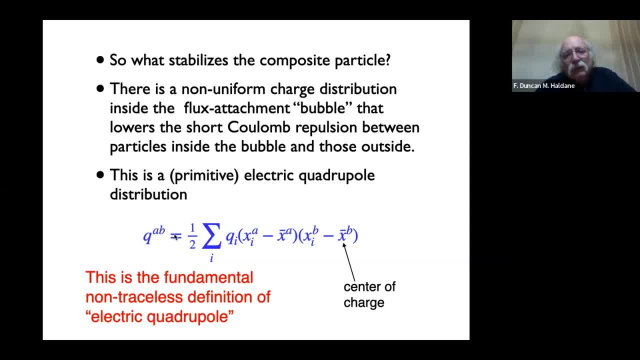 as a quadrupole. the part of the quadrupole that's proportional to the permittivity tensor or the dielectric tensor has no, has no long range field to it. that's the. you know that. that's the. that's why i use the traceless quadrupole. as you can see, if it's got two upper indices, a trace is actually. 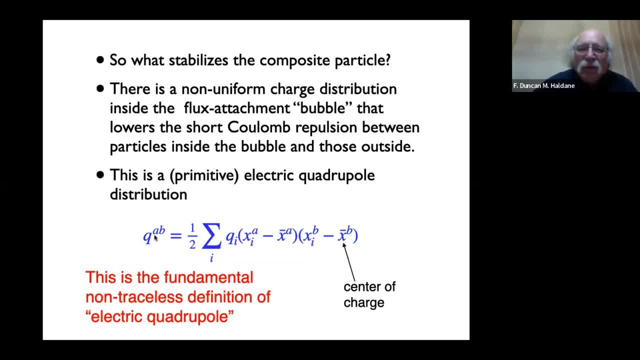 a contraction of an upper index with a lower index. so it's actually meaningless to talk. a symmetric tensor- actually a symmetric matrix- can have a trace, but a symmetric tensor cannot have a trace. it's a meaningless. it's mathematically meaningless to talk about the trace of a. 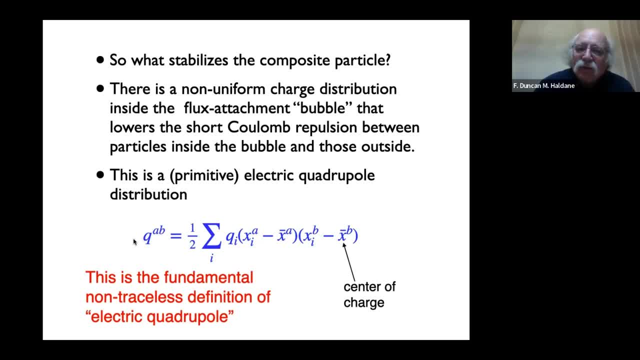 tensor. what you mean by the trace of such a tensor is to contract it with a metric, the metric being a, a symmetric tensor with two lower indices, which which you contract with that, so so trace. the proper meaning of trace is the contraction of an upper with a lower index, and so traceless. 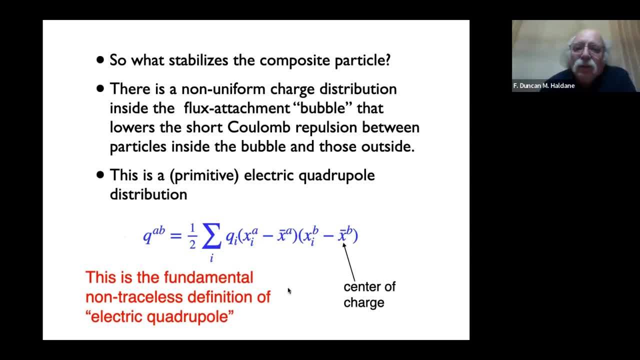 quadrupole is actually mathematically meaningless, although it's very. it's a common thing. it really means get rid of the part of the quadrupole which is proportional to the dielectric tensor, because it doesn't have a long range field. okay for laplace's equation. so there is a definition. 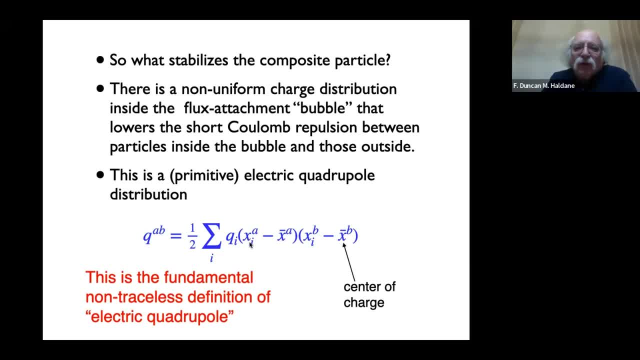 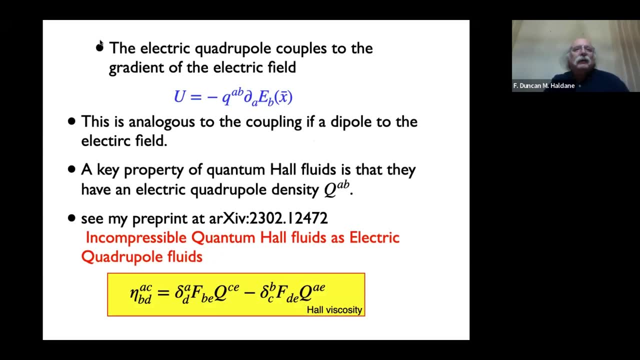 you, it's basically the variance of the positions of the charges relative to the center of charge, weighted by the actual charge. okay, and the interesting thing, the important thing about the electric quadrupole is, as i said it, it actually couples to the gradient of the electric fields, just like the charge couples to 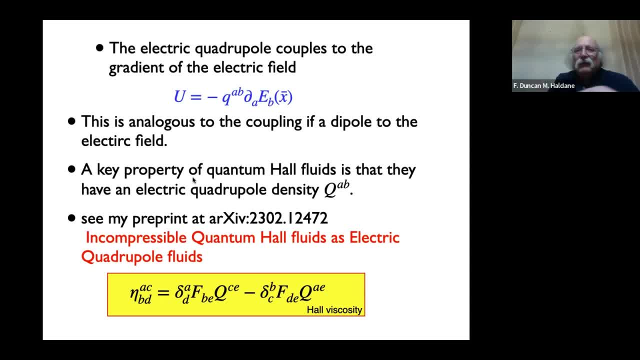 the electric potential. a dipole couples to the electric field, the quadrupole couples to the gradient of the electric fields. okay, and that will turn out to be um pretty important. well, so one thing i'll state is that the key property of all quantum fluids is that they have an electric quadrupole density, even the integer whole effect, the quadrupole. 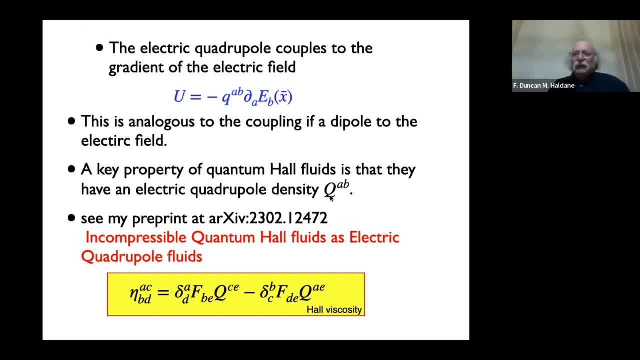 density is coming from the quadrupolar distribution of the electron orbiting around the guiding center, which is the little quadrupole. but a much more interesting quadrupole forms is the shape of the. the shape of the flux attachment bubble relative to its center is also a quadrupole thing. so the, the integer whole effect, does have a quadrupole, it it's, it's fixed by the band structure. basically. 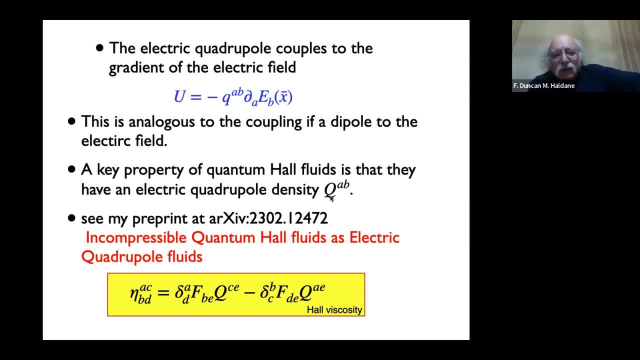 um, and so it's not a dynamical field like the of the, uh, the one associated with the shape of, with the shape of flux, attachment will be- and i have a pre-print out on that- and uh, one thing, that, uh, that that was came up in the last 10 years or so. it was discovered actually first in the quantum. 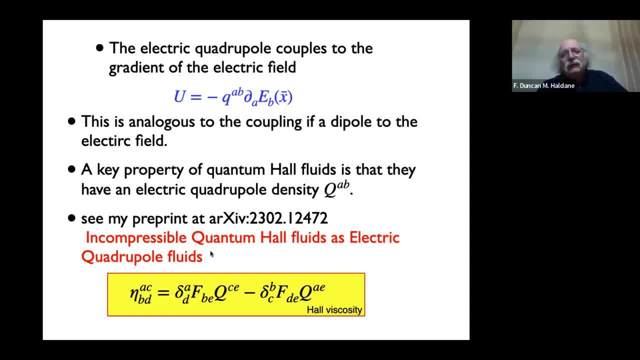 Hall effect. in the integer quantum Hall effect in the early 90s it was discovered that, uh, the whole fluid could have a viscosity. but just as the um conductivity, the whole conductivity of the whole fluid is dissipationless. so sigma xy is an anti-symmetric quantity, uh, 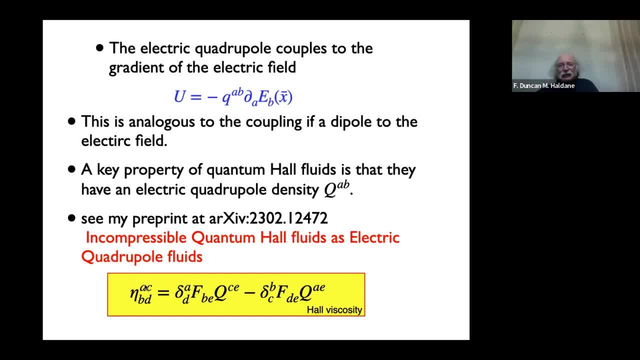 the, the viscosity is also dissipationless, and so the viscosity, of course, in general, will be the relationship between the stress in a fluid and the gradient of the flow velocity. it's dissipationless, uh, it's essentially. the stress is at right angles to the, the, the 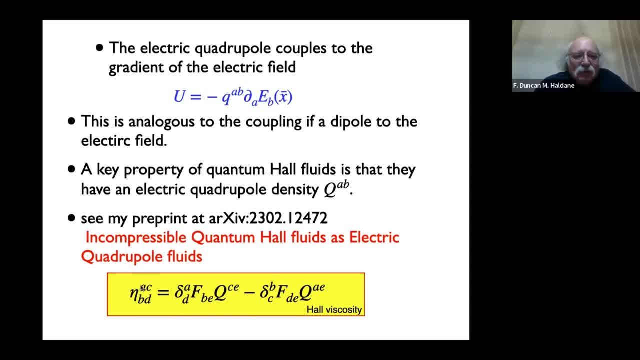 gradient of the flow velocity and indeed the, the stressed, the stress tends, the, the viscosity tensor, the stress is a uh. the proper definition of the stress uh, without using metrics and Cauchy, is: it's a. it's a tensor with an upper index and a lower index and the gradient of the 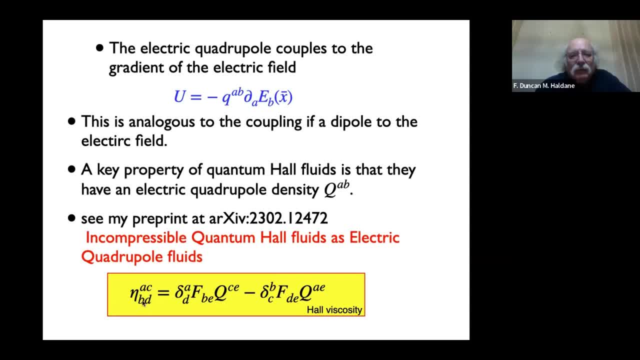 velocity is also a tensor with an upper index and a lower index, and so the viscosity is. the viscosity is anti-symmetric in exchange of the first two and the second two indices- which makes it dissipationless- actually turns out to be given by a remarkably simple formula. So it was discovered first. 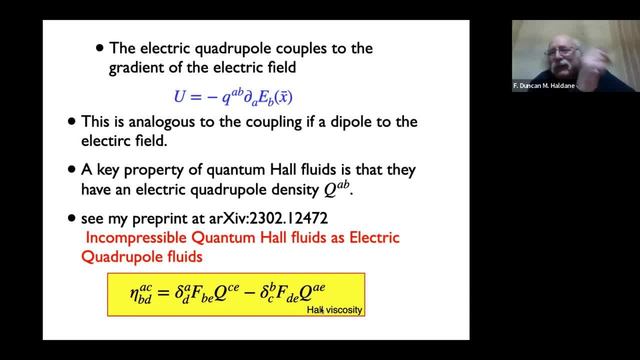 using the rotationally symmetric model and had formulas involving angular momentum and stuff like that. But formulas involving angular momentum can't be a generic formula, because there's no such thing as angular momentum in condensed matter physics. It's only a property of toy models, right? So the correct answer, which is equal to the previous answers. 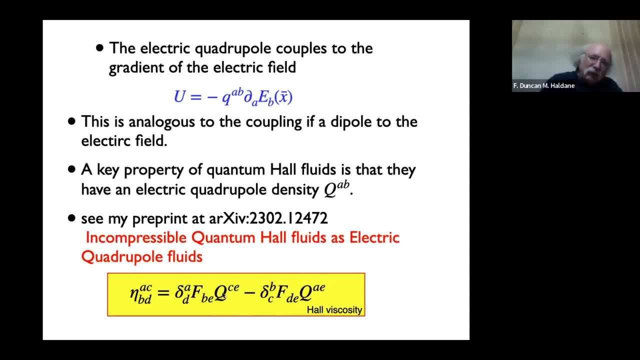 both for the fractional integer case by Avron Zogrov and Seiler and for the fractional case by Reid, turns out to be just special cases for toy models of a much more general formula which relates the viscosity, the dissipation of viscosity, to the 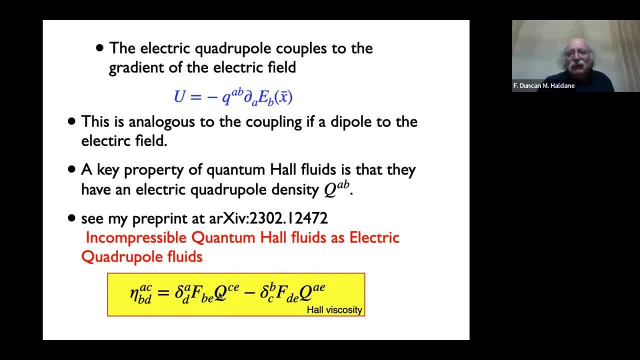 parallelism. The Faraday tensor, which is independent of handedness, is just a Faraday tensor times the quadrupole density. So the electric quadrupole has dimensions of charge times length squared. The electric quadrupole density in two dimensions has just dimensions of electric charge. 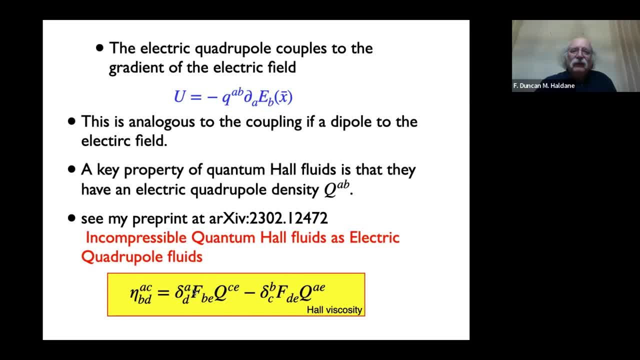 So electric charge times, magnetic flux is just Planck's constant divided by electric charge. This is a dimension, of course, of the velocity, which is by length squared, which is action per unit area, which is the dimension of viscosity. So this is a dimensionally correct formula. and you can ask why? why does the quadrupole enter in the definition of the viscosity? 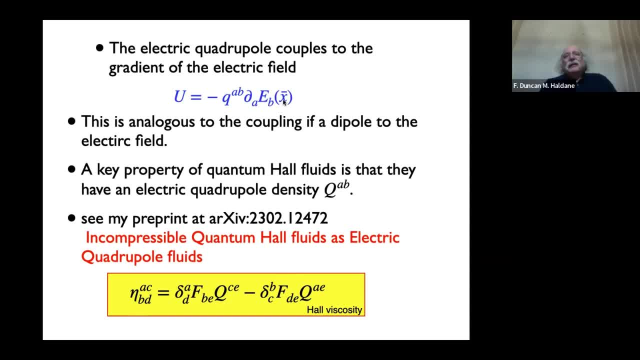 It enters precisely because of this formula Here: if the electric field inside the whole system is constant- a uniform electric field- everything flows with exactly the same velocity. The guiding centers just move. they all move at the same speed, So there's no relative motion. 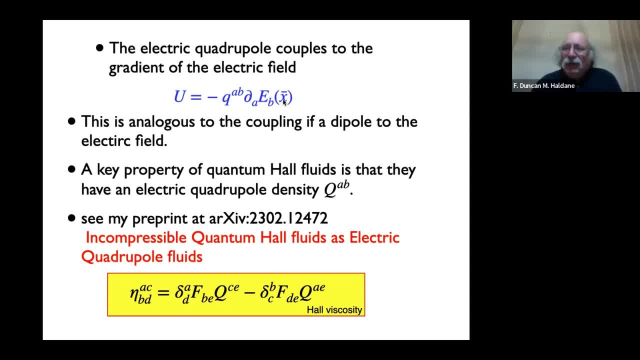 of different parts of the fluid and no gradient of the flow velocity. If the electric field is uniform, the flow velocity is just the drift velocity E over B. But if E is spatially varying, which it certainly is if you've got edges and things in your sample- 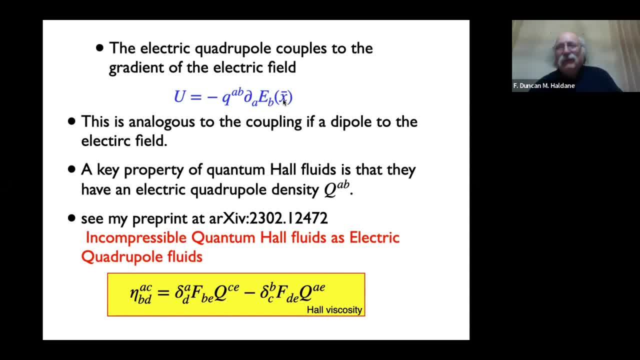 then there's a gradient of the electric fields, And then, if there's a gradient of electric field, there's a gradient of the flow velocity, but the gradient of the electric field is precisely what couples to quadrupole, So it's actually physically absolutely transparent. 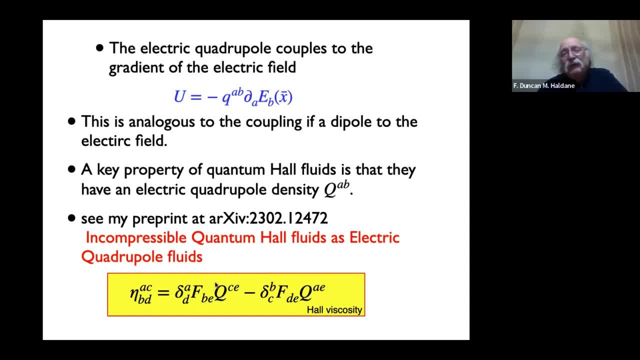 when you see the formula, that the whole viscosity just involves the magnetic fields and the quadrupole density of the fluid. So okay, So the quadrupole density occurs not only in the magnetic field, not only is it explaining the energetics of the fluid. 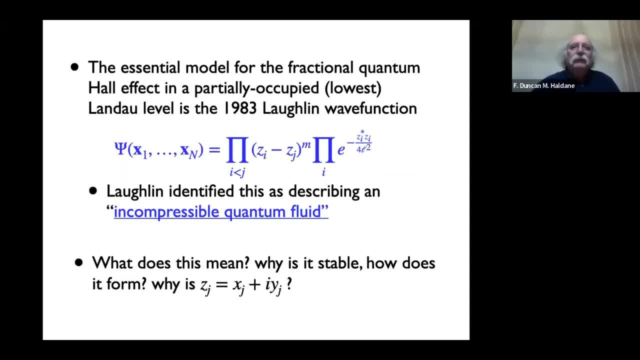 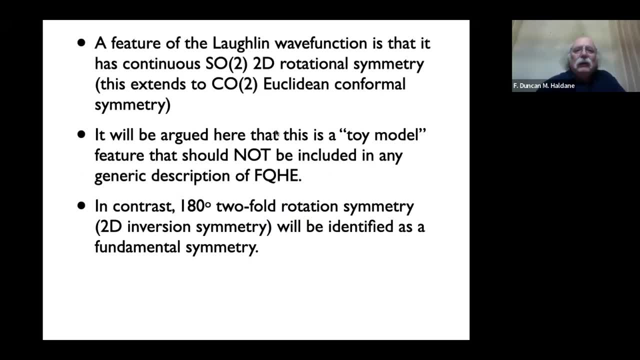 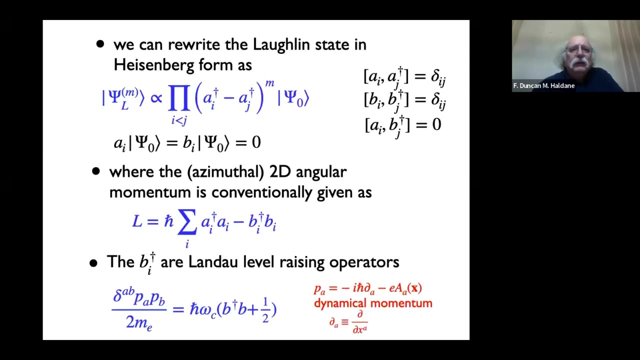 but also the okay, let's move on. Okay, so let me pass some of these slides of repetitions. So one thing about it is that the quadrupole obeys an algebra which is: let's skip that part, Okay, let's skip the whole of this. 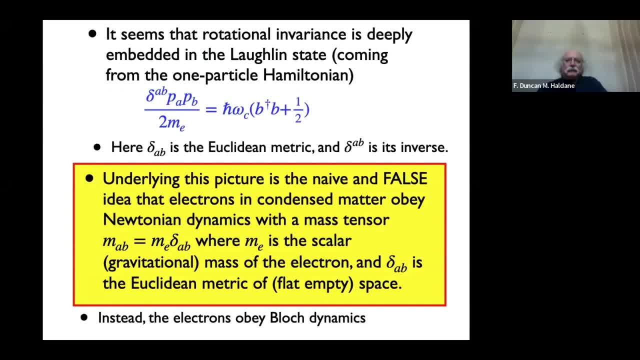 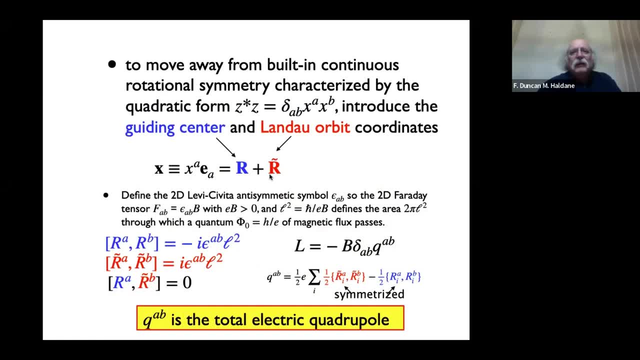 Let me skip over because I haven't got much time left. Okay, Yeah. so if I go back to the description in terms of the guiding centers and the Landau orbits, they obey this interesting algebra where the guiding centers don't commute and the Landau orbits don't commute. 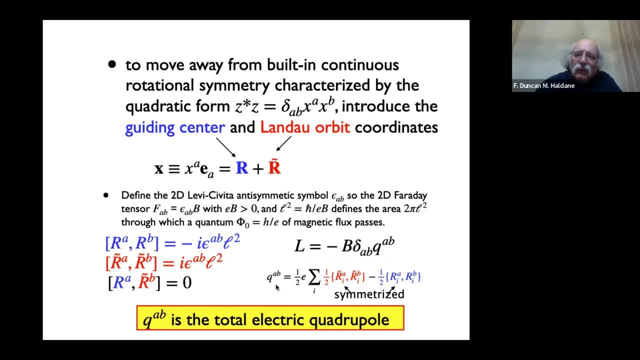 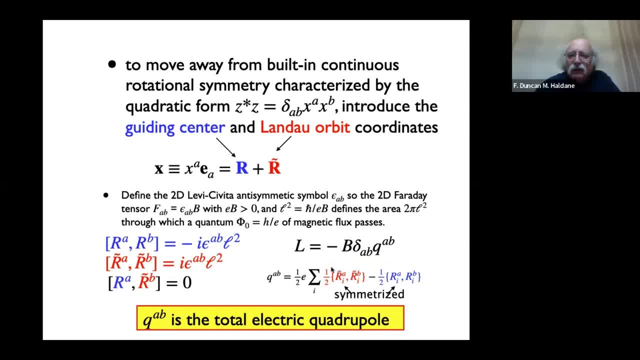 with the electron moving around its guiding center. And there's another part which, when you subtract off the background, enters with a minus sign which tells you about the shape of the that is coming is the part of the quadrupole that's emergent. 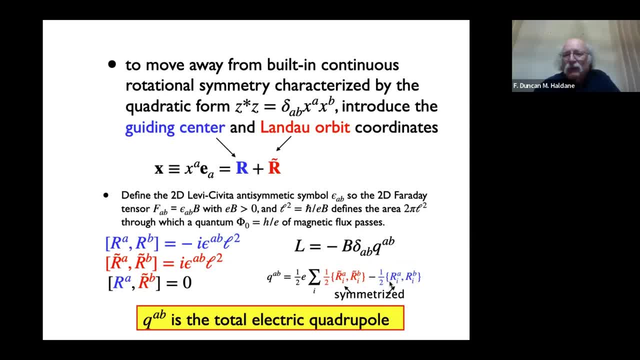 that's the shape of the flux attachment bubble. So this part is completely absent in the integer Hall effect. The quadrupoles in the integer Hall effect only come from the Landau orbit going around the guiding center which has a quadrupole. that's fixed. 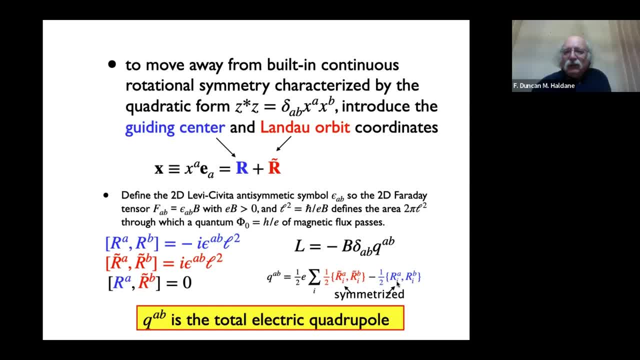 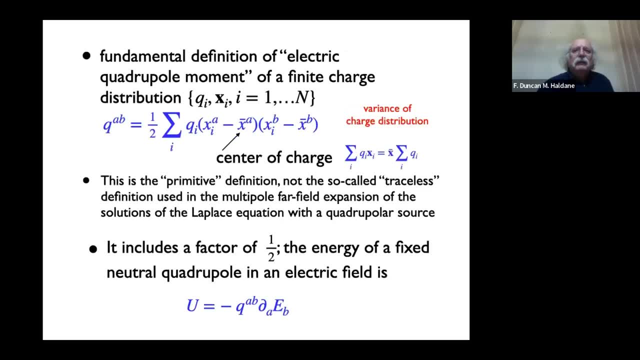 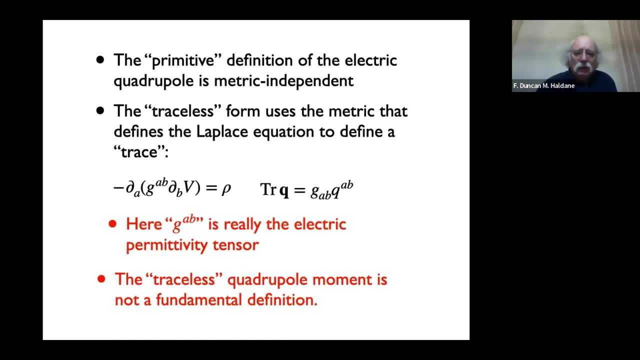 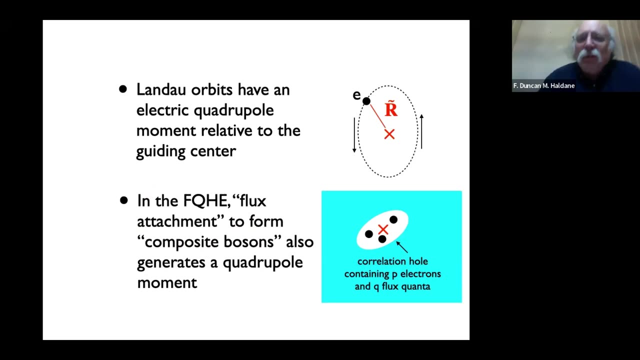 by the band structures underlying it. But this part is the emergent part, which gives you the okay. So let's see if I could move forward. Okay, This is just saying more details about the definition of the quadrupole. Let me get to. let me just finish up with pictures. 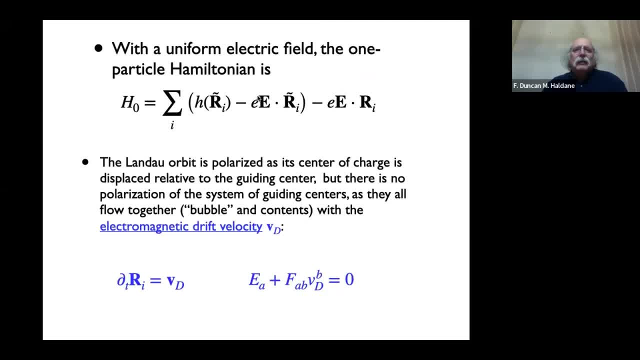 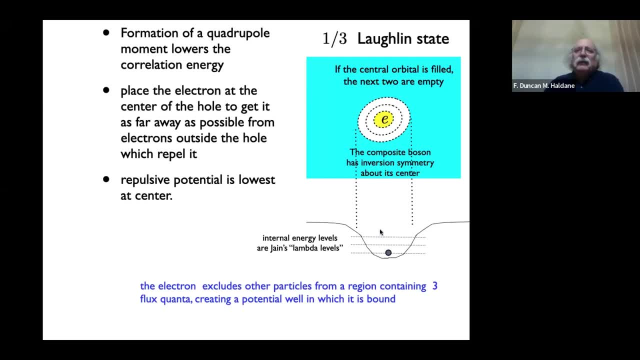 Okay, So here's a whoops. Here's a picture of the, the Laughlin state, at one third. where I've drawn it, There's the bubble and there's the electron sitting in the in its in the center of it. 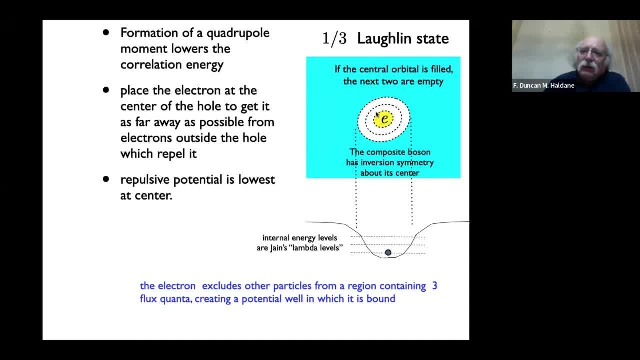 So this is very analogous, that the unit, this is the unit cell in some sense of the liquid. It's very analogous to the unit cell of a solid right In a solid. if I take solid helium and remove one, elect, one atom, there'll be a empty unit cell. 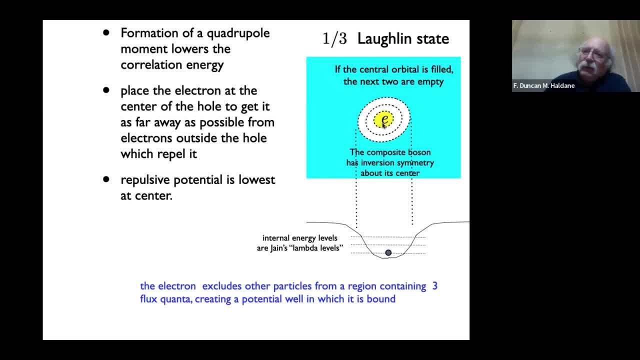 will have a attractive potential at the center because it's it's the furthest point away from all the other atoms which are repelling it. Similarly, here, the if I have an empty bubble here, there'll be a potential inside it. 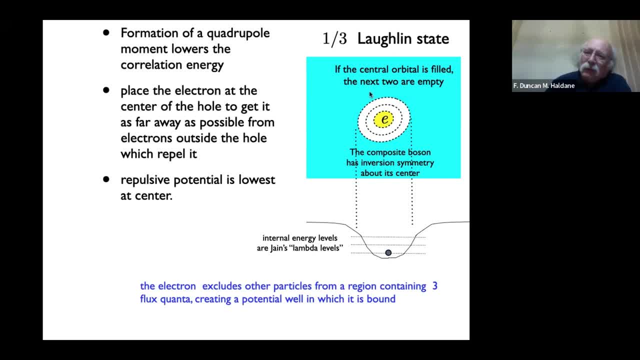 which is minimized at the middle, because that's the furthest point, that's away from the other particles, And because it's got three fluxes, it supports three, three electron states, And and there's the central one will be lowest. 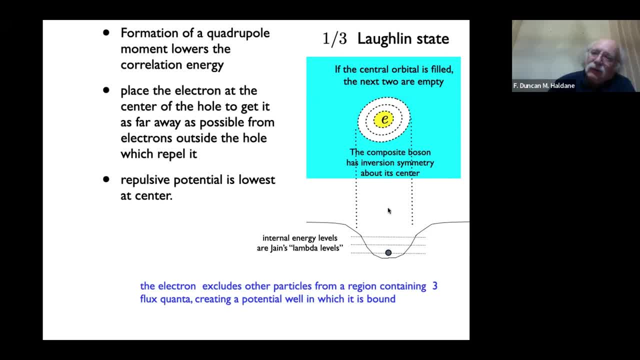 because it's closest to the middle. The next one will be higher and higher And higher. So this is a picture of the, the composite boson for the for the Laughlin state, And again, the basic principle is that the electron 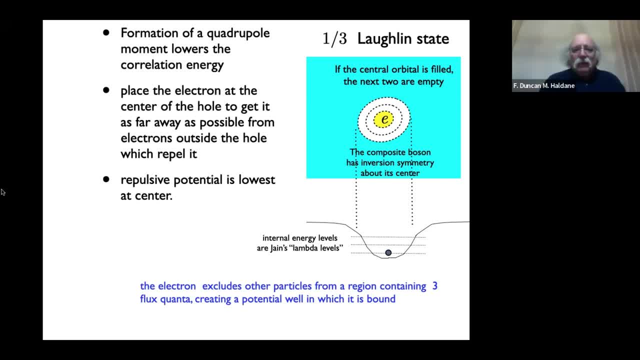 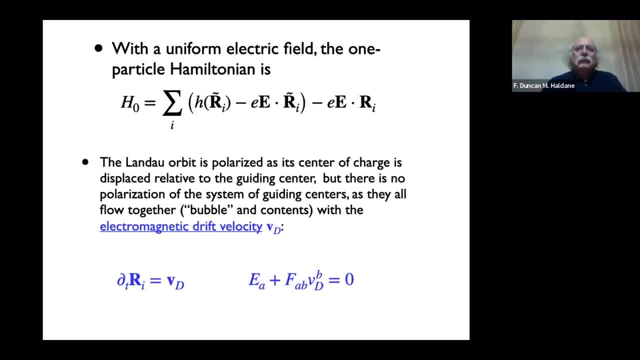 excludes the other particles from from its bubble. Okay, If I now let's move. Okay, Yeah, Let's see, Let's move on. And this is just telling you that basically the the guiding centers, if I apply an electric field to the problem, 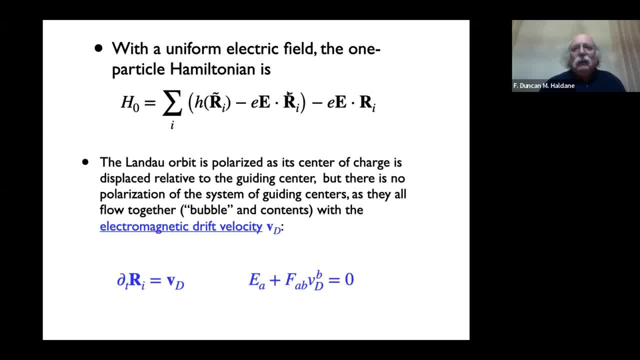 the electric field actually does distort the shape of the Lambda orbit. But when it acts, the part of electric field that acts on the guiding center just makes it. if it's a uniform electric field, just makes them all move at the drift velocity. 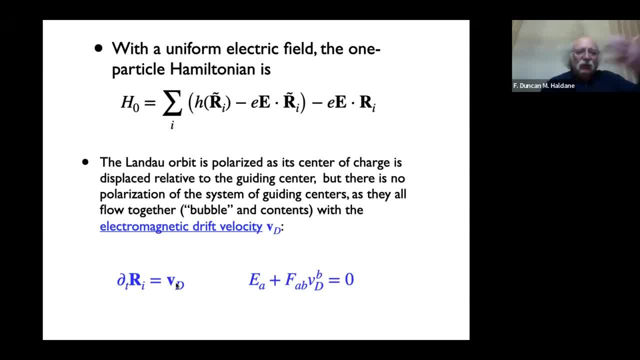 So that's why there's no, no, no distortion of the shape of the bubble due to uniform electric fields, but quadratic. but. but gradients of electric fields cause a distortion of the shape of the of the flux attachment, because they couple to the quadrupole moment. 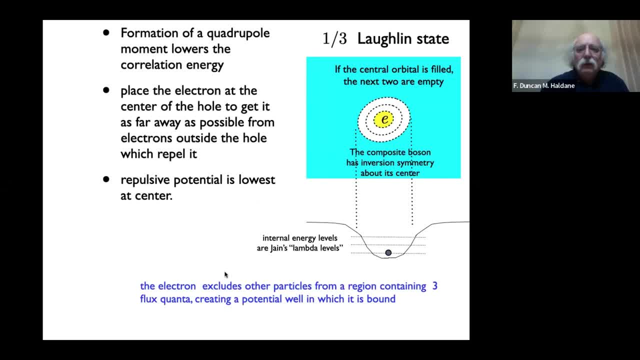 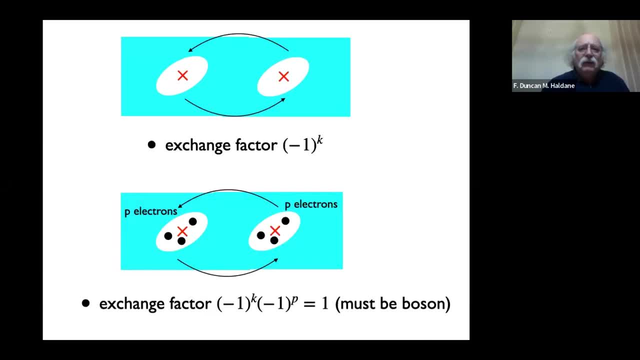 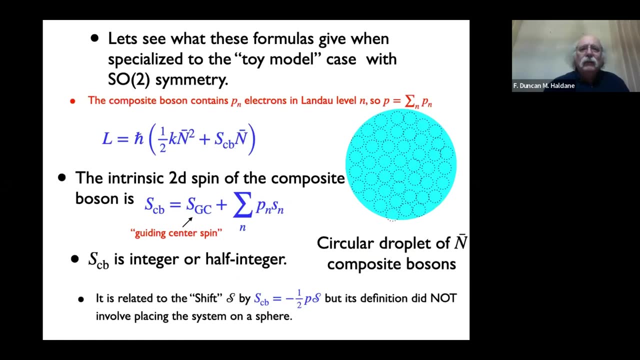 Okay, Okay. So let's see Going the wrong way. So let's just look at a few pictures. right, Let's look at get away from Chern-Simon theory, Okay, So one of the things we can see in the 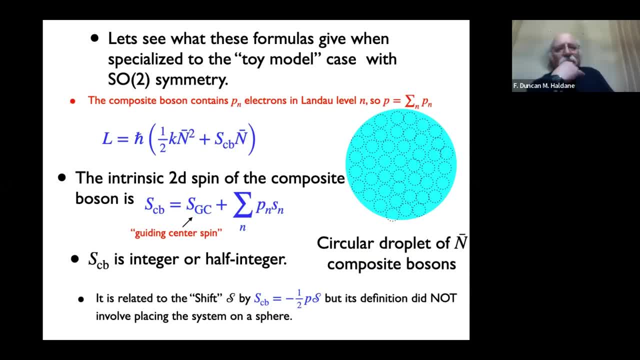 if one actually does look at rotational symmetry. take the toy models where you could take which the Lofven state is one of the toy models, cause it's got a, it's got a rotational symmetry. If I actually calculate the angular momentum. 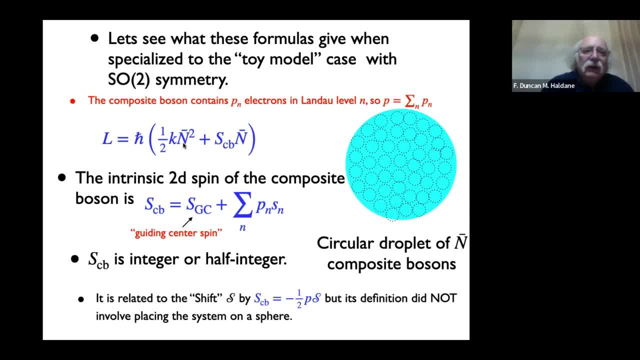 of one of these droplets. it's actually interesting because the angular momentum contains a part which is quadratic in the number of composite particles and another part- correct me if I'm wrong- another part- correction part- that's linear in number. So the first part involves the Chern-Simon's index K. 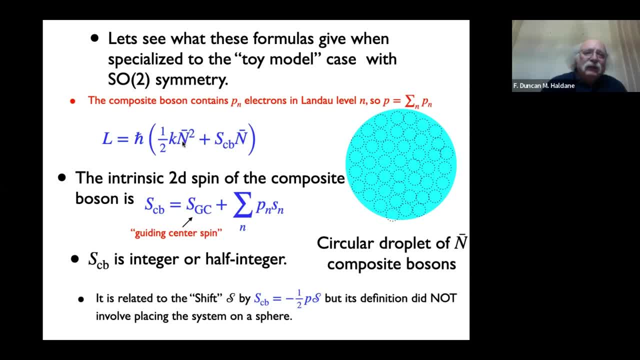 And this is a problem, that this is a super extensive part that you have to remove by subtracting the background And the in the rotationally invariant models, the shape of the quadrupole of the distribution is quantized because of angular momentum quantization. 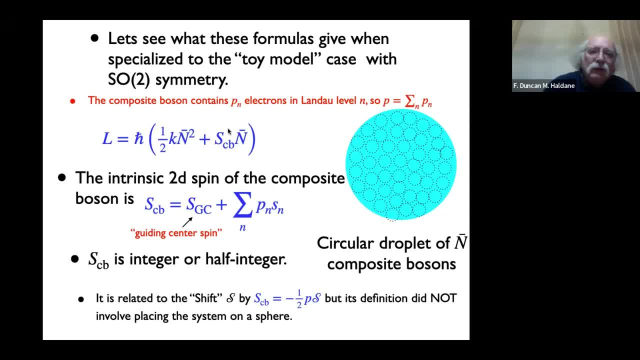 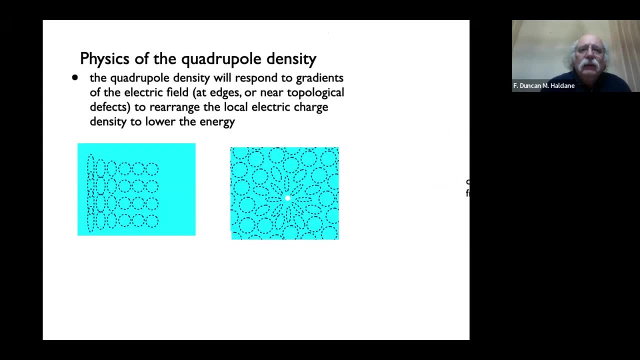 And these were the formulas for the whole viscosity which were originally discovered in the toy models, which involves the angular momentum of the composite boson. But let's, let's move on. So again one can. let's have a look. 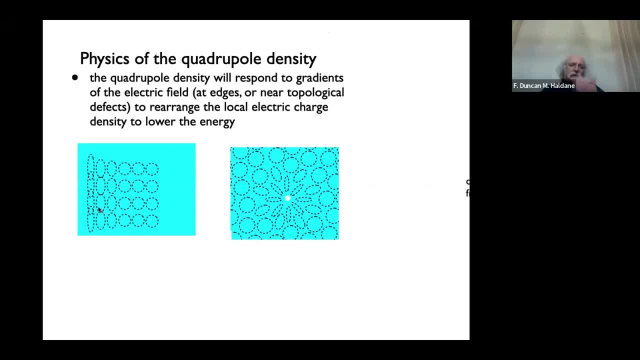 So the quadrupole density is. this gives rise to this kind of new feature, And we can see that if we're near the edge of a sample there will be a gradient of the electric field. And if we're near the edge of a sample, 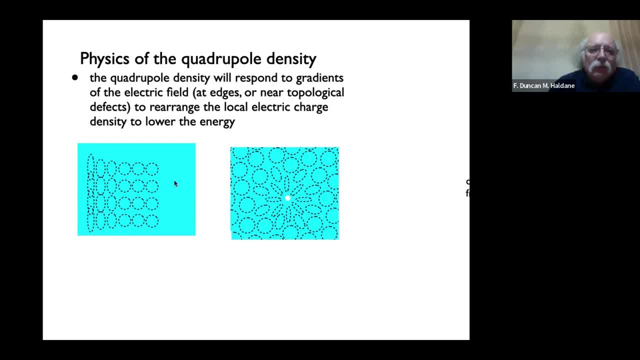 there will be a gradient of the electric field. There's the, the edge of a sample. the electric field will kind of look like a quadratic function and the there'll be differential flow of the fluid and the electric field gradient will actually act to deform the shape of the quadrupole set. 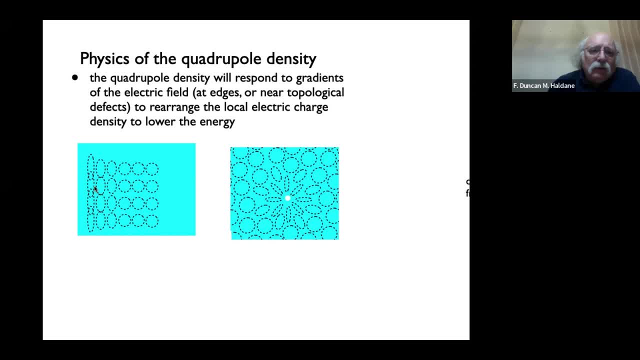 And so the shape of these things, the- if there's, if there's a gradient of a quadrupole density, you have a polarization. If there's a double derivative of the quadrupole, it's like the gradient of the polarization. 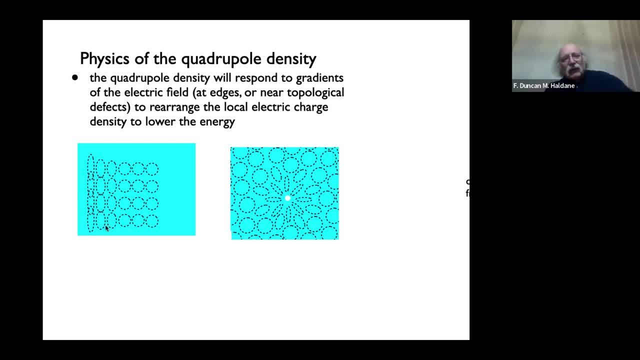 which is a bound charge represented. So the deviation of the quadrupole from or spatial variation of the quadrupole gives rise to a bound charge which allows you to screen things, For example, near a topological, near a quasi-hole. 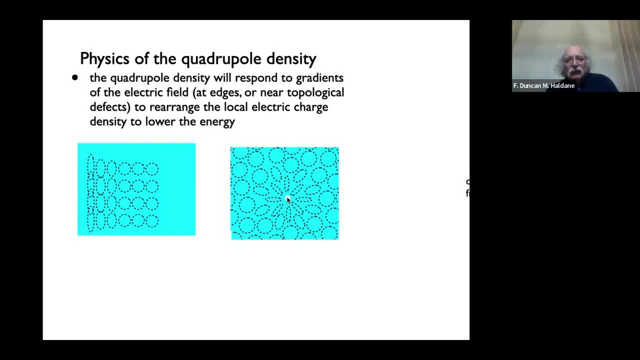 there'll be a strong electric fields which is non with, which is not a non-uniform and it can be partially screened. The charge, the point charge, can be spread out by deviation, by causing deviations of the quadrupole shape locally. 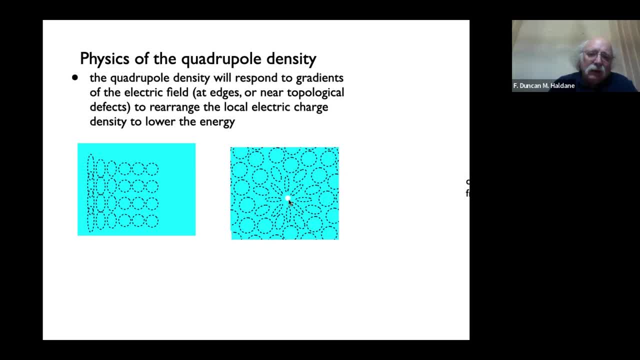 This is very analogous to something that's known as skirmions in quantum Hall-Ferrer magnets. So there's a large, a great analogy between the dynamics of the quadrupoles in the quadrupolar fluid and the dynamics of the ferromagnetic order parameter. 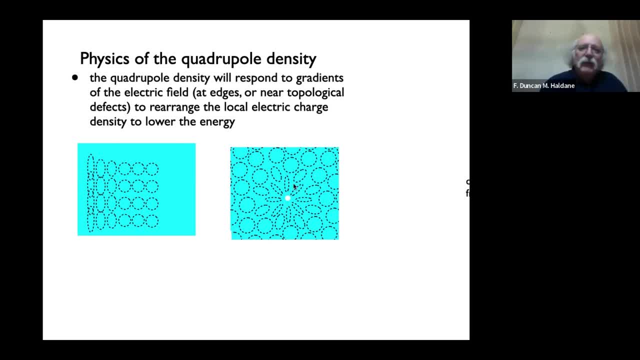 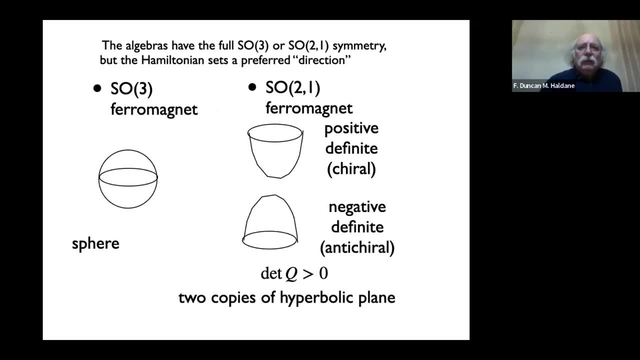 in quantum Hall-Ferrer magnets where you have skirmions and things. I guess I'm kind of almost out of time in this thing. Let's have a quick look. Let me show you some more pictures of things. So one thing that emerges that one sees very nicely. 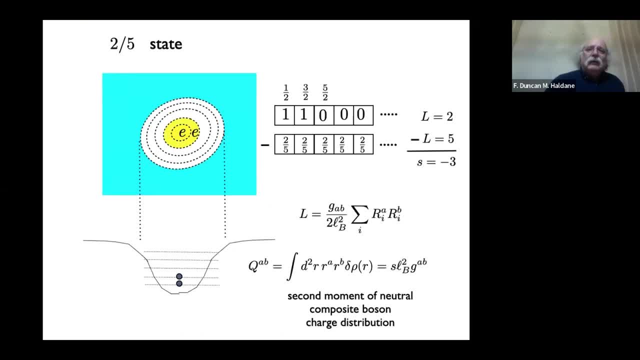 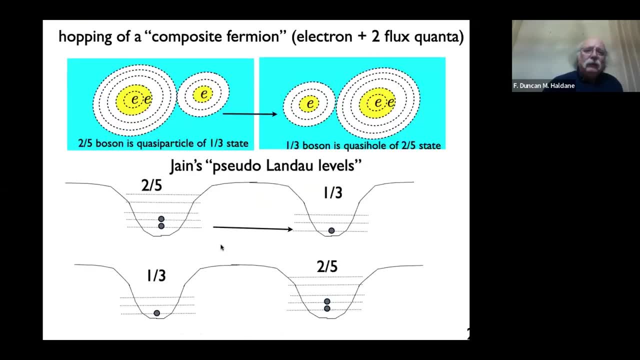 in the composite boson picture is what happens as I go from the sequence one-third to two-fifth, for example, And we can now start to make contact with the alternative description, due to Jane of quasi, of composite fermions. So if I have the two-fifth state, 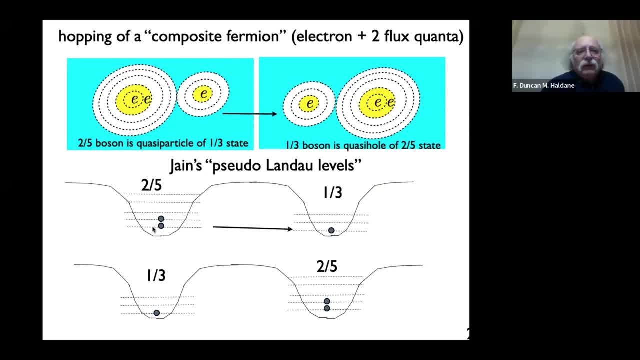 I have two particles in five fluxes and they're going to be five, five orbitals in the center of the little void And of course the ones closest to the central one is the lowest, the next one up, And we should fill these orbitals. 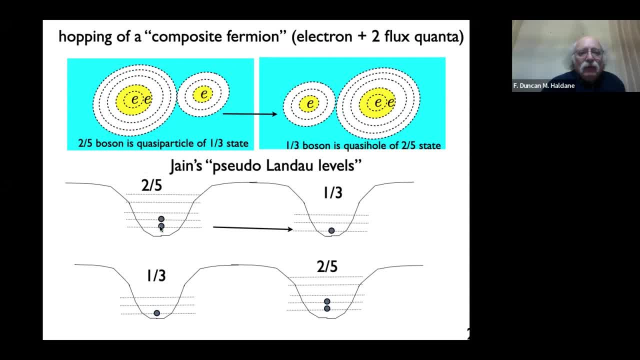 in the Pauli principle order: right Go from the lowest. the second, the third- And this is very reminiscent of filling Landau- levels up. And so the composite fermion language for the for describing the things like the one-third, two-fifth, 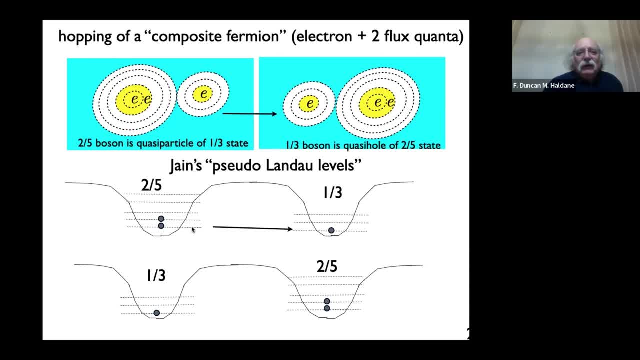 three-seventh sequence would associate, essentially introduce the things called Lambda levels, which is, or pseudo Lambda levels, And we could actually see that the pseudo Lambda levels are in fact just the different levels inside the composite fermion. So in the Jane picture this would be occupying two. 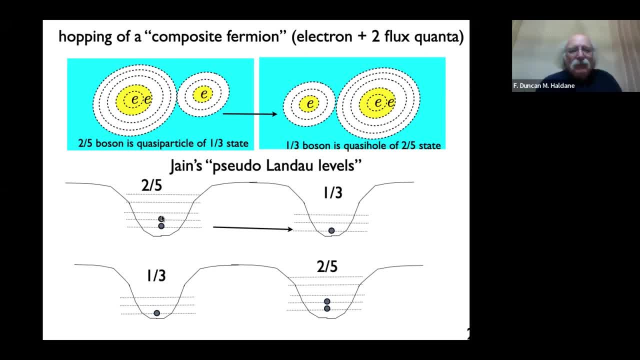 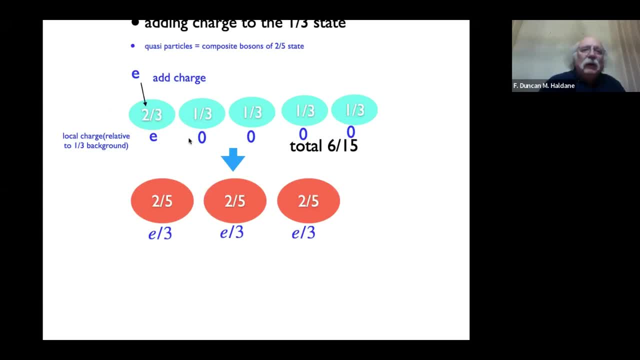 the lowest, two pseudo-landau levels. and now we can see that if i, and if i look more closely, let's see if i can find the picture, let's, let's dope the. let's see what happens when we add charges to the loughlin. 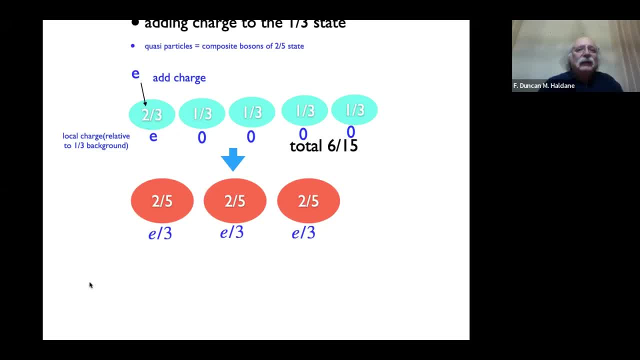 state. if we dope the loughlin state in the same way as doping a semiconductor, we add a charge to it. so where's that charge going to go? initially, if the loughlin state is made out of these units, which are one particle owning three orbitals, the charge should go into one of them and it'll change. 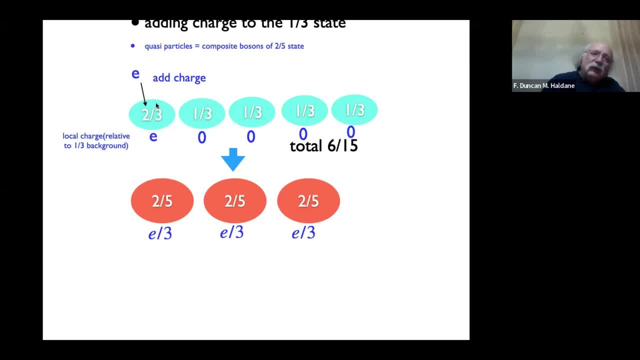 it to two-thirds, so we'll have an object here which is not a different from all the others. it's actually going to be a fermion. these guys are bosons by adding an electron to it. it's a fermion, that's a. this is a local. this has a local excess charge of one one electron. 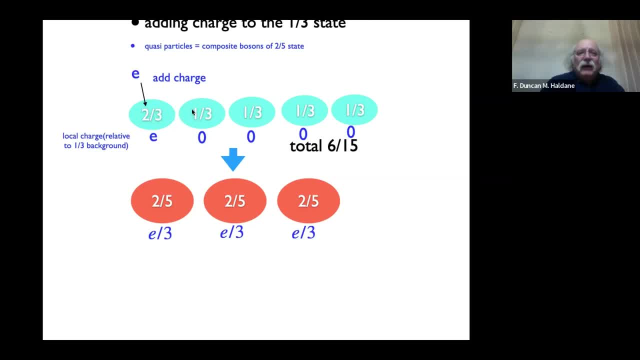 but we can see that if i actually combine it with a, four of the neutral bosons, so i have two, three, four, five, six. i've got six particles in 15 orbitals. uh, that's exactly what you need to make. three, two-fifths states. so every time i add an. 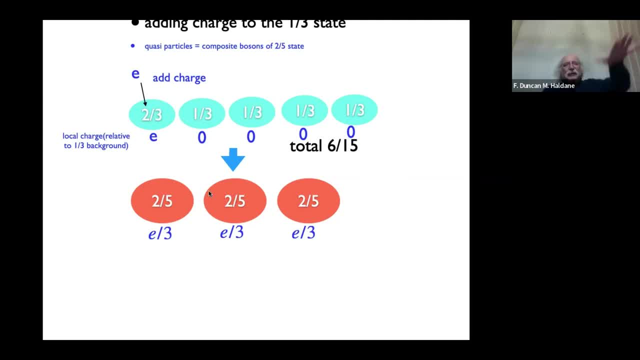 electron to the one-third loughlin state. it splits up into three plus a third charge objects which are in fact little droplets of the two-fifths state, which is the next one up in the sequence in the in the main sequence of quantum hall states above. 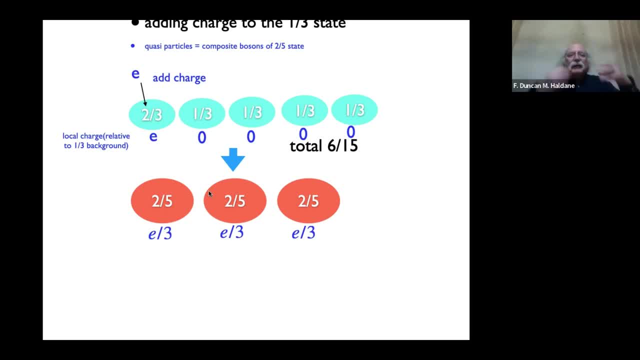 one-third. and so as i, each time i add another electron i get three more of these two-fifths droplets and i lose. and each time i add electron i lose four of my. i lose five of my uh, of my one-third droplets. so i'm gradually diluting the one-third bosons which are condensed and 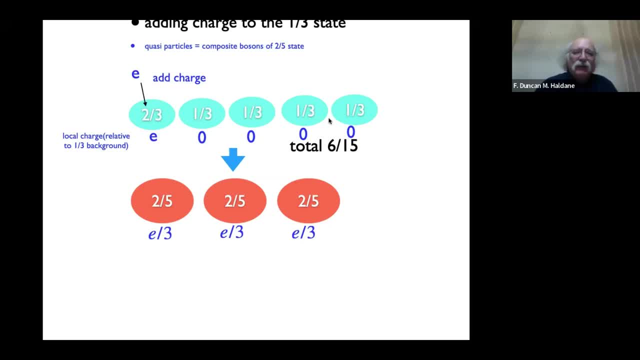 filling them up with lots of isolated two-fifths bosons. the two-fifths bosons will coalesce and condense and then you'll get left as you continue to fill. then you'll have a two-fifths state with isolated, uncondensed one-third bosons floating around. 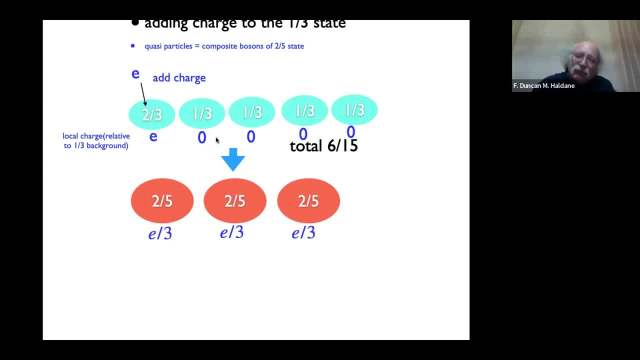 and eventually they all disappear when you get to two-fifths. so the the sequence of of what happens as you fill these things makes a lot of sense and you can see in the composite boson language. but now let's see how what charge transport does inside the system. 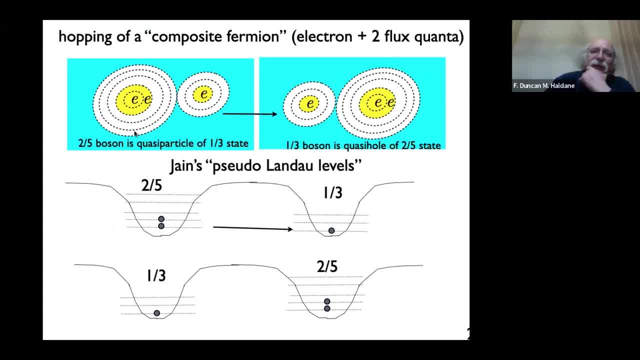 so here is a two-fifths state, a two-fifths uh unit cell, the two-fifths boson, which i really, which is really the analog of the unit cell, and the solid. it's the fundamental unit of the fluids. i've got a two-fifths one next door to a one-third, so there's an excess charge of one-third here. 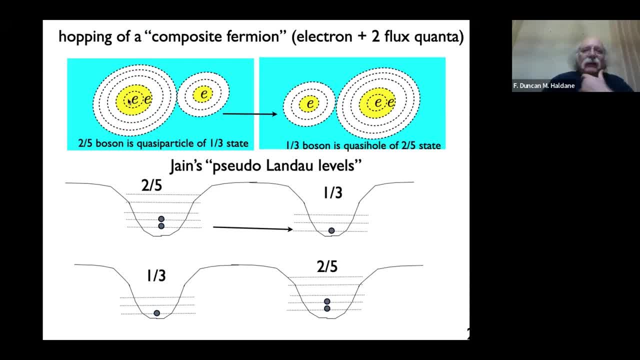 this is a quasi particle of the loughlin state, which is right. so there's no particle whole symmetry of the loughlin state. of course it's. the quasi whole is very different from the whole. the quasi whole is just an empty. a single is zero electrons in one flux is the quasi whole. 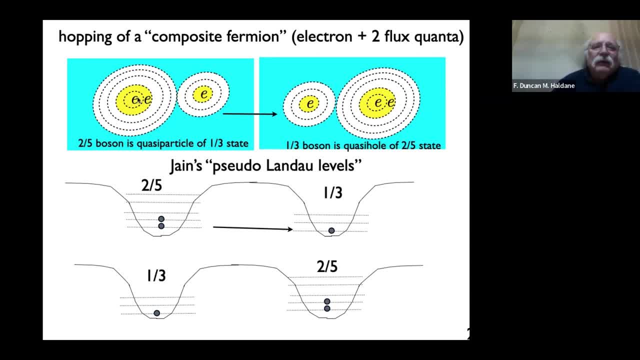 the quasi particle is two electrons in five. but if the charge wants to move around, if we think about how charge moves in a dope solid, it doesn't. the unit cell doesn't move. the electron hops from one unit. an extra electron in one unit cell will just hop to the next unit. 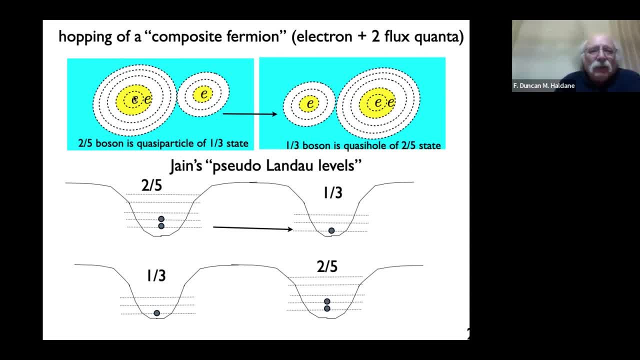 cell. so you can see, what actually hops is not the electron itself, but the electric. one of these electrons will move. it'll take two flux quanta with it. so what will hop is an electron plus two flux quanta, leaving behind a one-third here and the two-fifths here, and the thing that moved is precisely the composite fermion of of uh. 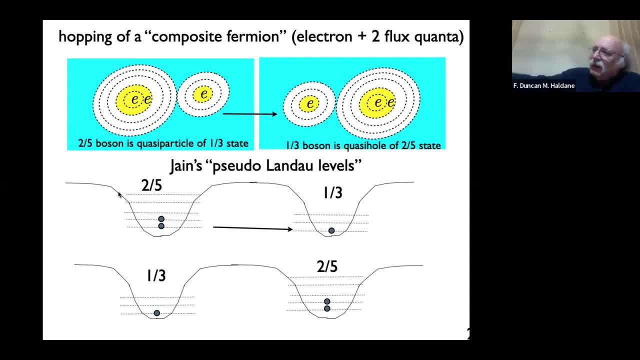 jane's picture and looking at dynamics, uh, one actually can see the composite fermions moving around when you do things like that. so that's the one-third here and the two-fifths here and the other two-fifths here and the two-fifths here and the other two-fifths here and the other two-fifths. 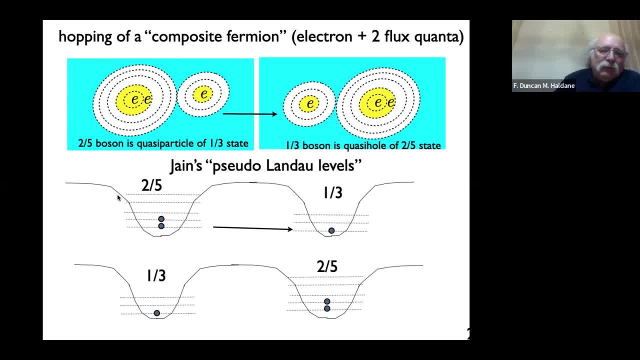 like put a kind of grating a grating and look at interference effects in, in, in, in doped um states. so you have a. you have a complementarity between the composite boson picture, which is describing something like the unit cell of the fluid, and the composite fermions, which describe the uh, the. 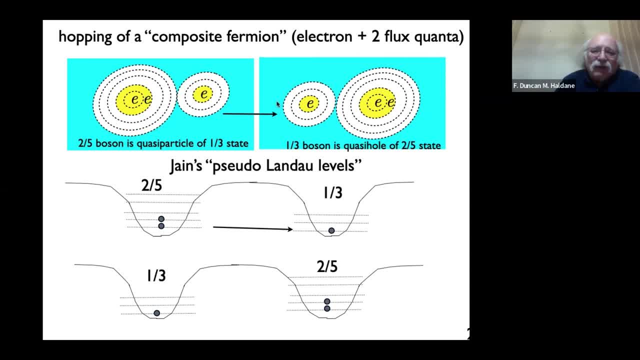 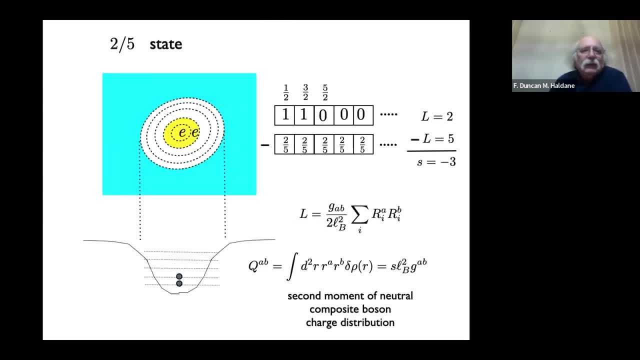 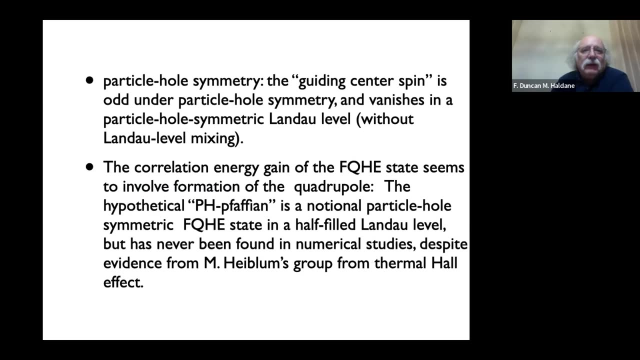 in these simple fluids, the, the mobile charges when you dope them. okay, okay. so so i guess, um, There's a lot of things one can do in this problem, but I think the most interesting thing is to try and understand the dynamics better. And so I will say that, if I look at the 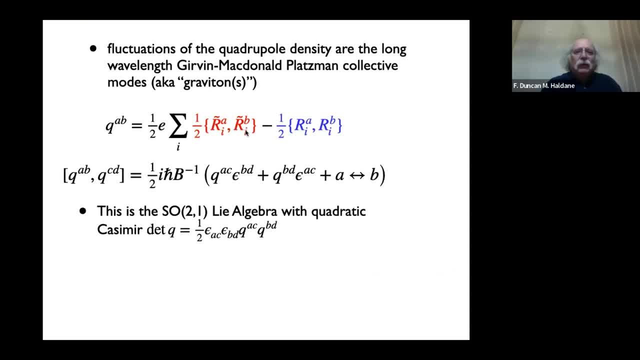 if I look at this operator, which is the quadrupole operator, and look at its commutation relations, it actually obeys a Lie algebra. OK, so this is quadratic. So when I commute two quadratics, I get one pair of, of the, of the of the coordinates get killed by the commutation relation. 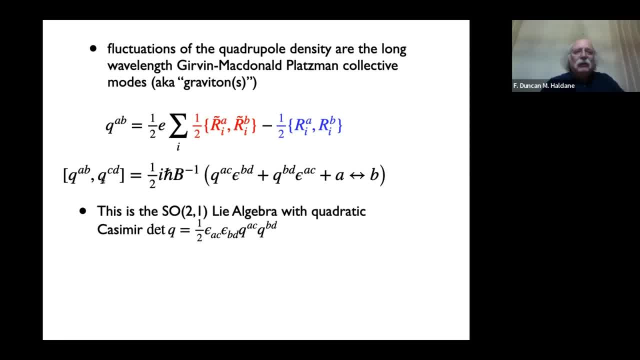 I get left with the quadratic part. So this is quadrupole. commuting with quadrupole is quadrupole, But this is not the. this is. this is a Lie algebra. It is actually the SO2,1 Lie algebra, And the Casimir of this algebra is the determinant. 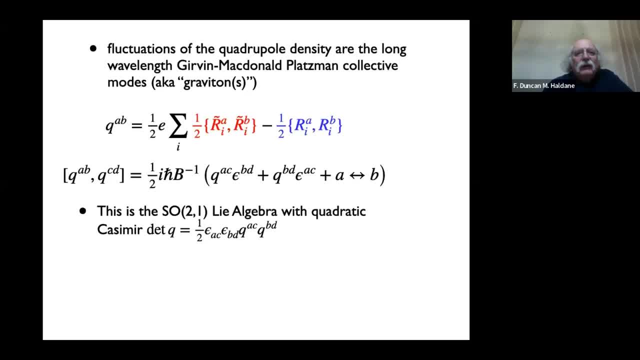 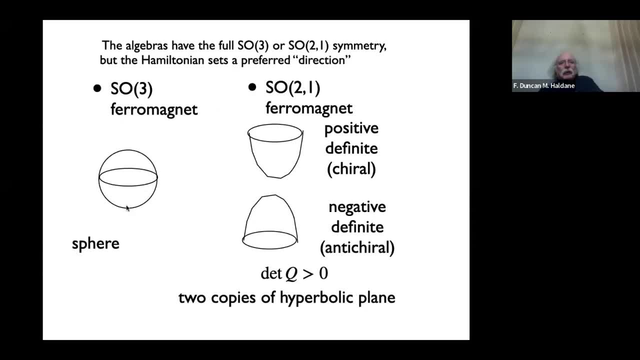 Of the quadrupole, So see if I can find the picture. Yeah, so that should be the quadrupole. fluid is very analogous to a ferromagnet. If it, if the algebra was SO3, it would be a ferromagnet and the order primity would be the direction of the direction of a vector. 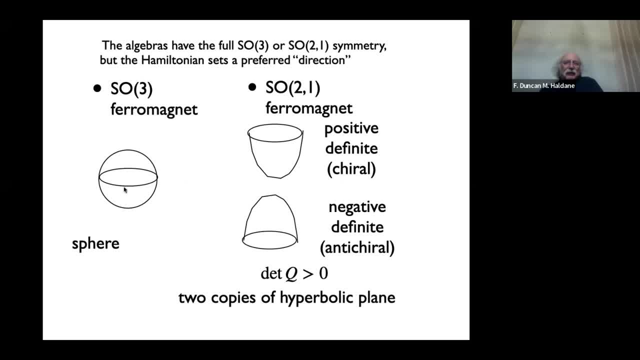 If I want to get the ferromagnet, I put a Zeeman field on it Which makes the gives it a preferential direction to put the spin in. The quadrupole dynamics is the SO2,1 version of the ferromagnet. 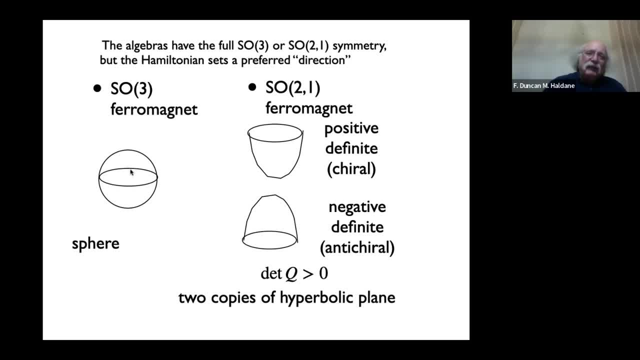 So, instead of the Casimir in this case is x squared plus y squared plus z squared, The Casimir in this one is x squared plus y squared minus z squared, So the, so the analog of the sphere is actually too. hyperbolic Surfaces which actually map into the, the, each each a map into the, into the Poincare disk or the hyperbolic plane. 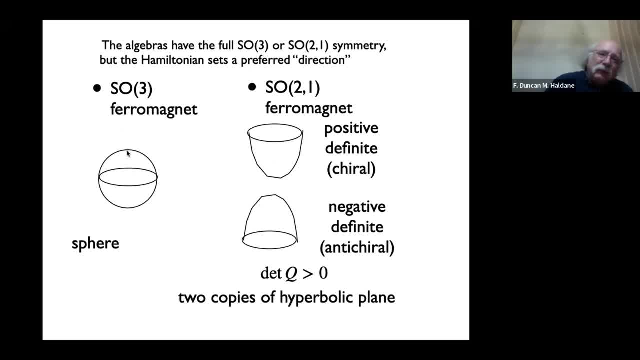 But now there are two branches of it here in the, in the algebra of the SO3.. You have a ladder of states going down, going between plus s and minus s. In this one you have either have a ladder of states going from s up to infinity, a semi infinite ladder. 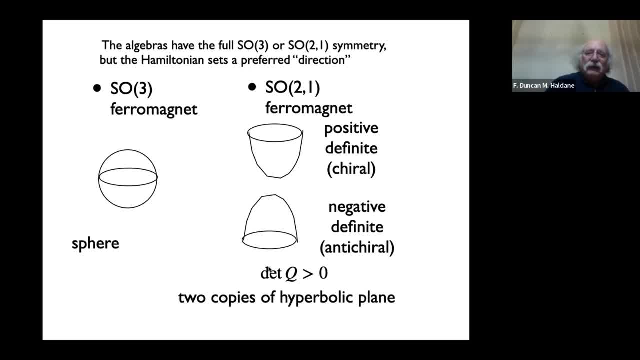 or you have a ladder going from, from the minus s down to minus s, Down to minus infinity. And so there are two kinds of the quadrupoles: the definite tensors, The- they can either be positive, definite or negative definite- And indeed the, the guiding the land, the orbit part. quadrupole is a positive, definite tensor. 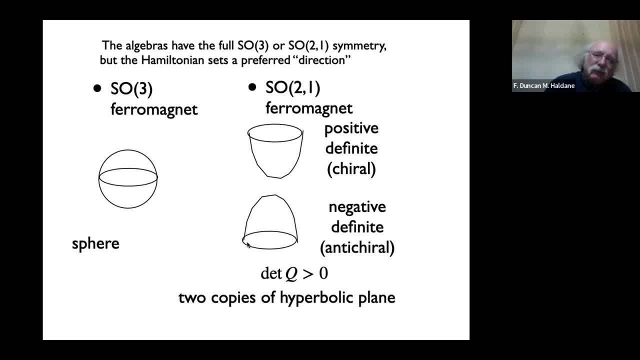 And the and the land, though The guiding center one is is negative, definite, But it's also the guiding center One is also odd on the particle whole symmetry of the lander level. So if I do an anti-loft in state by particularly holding the, the, the guiding centers within the lander level, 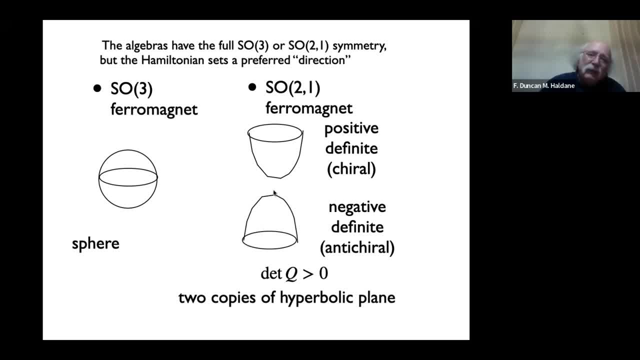 I actually also get it turns it into a positive one. So there's a big interest, interesting feature: What could happen at the half filling of the of a lander level? The quadrupole moment is odd on the particle whole transformations. This picture suggests that. 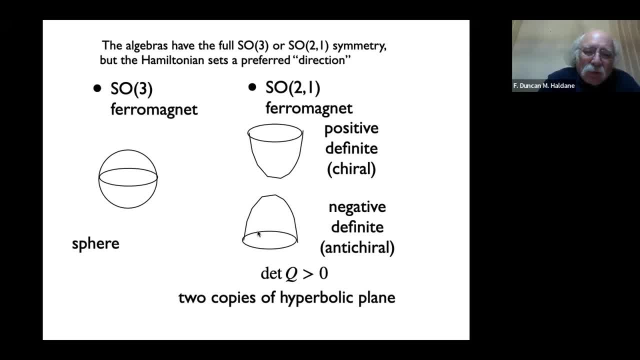 That that you need a quadrupole moment to get any energy gain to stabilize flux attachment. So there's a huge controversy about about what happens in the half filled lander level, because Thermal Hall effect measurements in the second level level- half filled sort of being- have suggested a particle whole, symmetric quantum whole state. 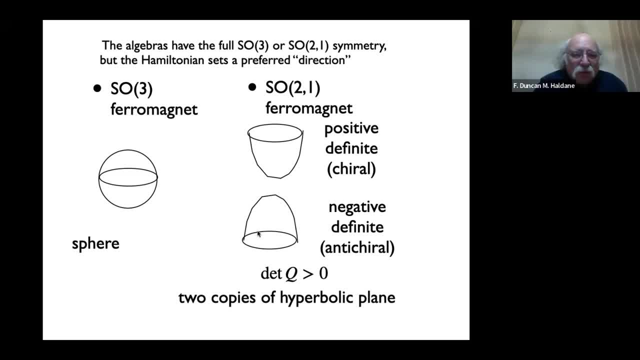 The quadrupole idea actually rules out the possibility of particle whole symmetric States, And So there's actually suggests a principle that something like the Liebschor's to Mattis principle in spin chains that if you actually have a Particle whole symmetric lander level and any two body interaction within a particle within a lander level is particle symmetric. 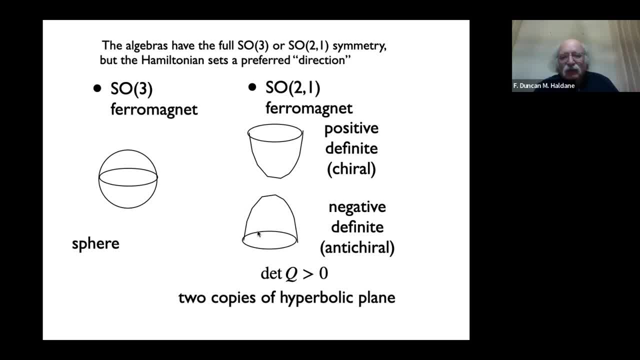 Then you either, to have a quantum whole state, you have to spontaneously break particle symmetry, And the potentially broken states would be either the more read Fafian or it's anti Fafian particle whole conjugate, So that so something that comes out of the energetics makes a strong suggestion that the only way the the experimental results. 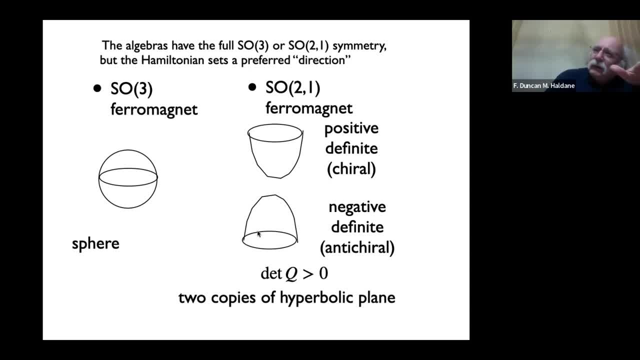 So we've actually got experimental results on On a untwisted Bernal stack bilayer graphene. We show definitively that you either in that system You either get a gapless system, a circle composite Fermi liquid, which is particle whole, symmetric with but not a quantum whole state, or you get some. you see both the Fafian and the anti Fafian a different places in this rather complicated 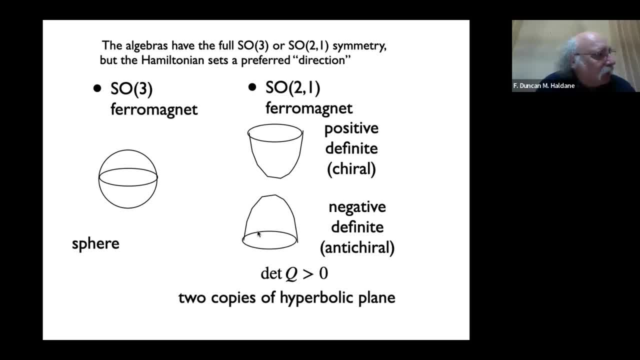 But now twisted but now untwisted graphing thing. The interactions in that one are slightly different from the interactions in the gallium arsenide system, Where, where they are the thermal whole measurements that seem to be compatible with a particle whole, symmetric case. but the solution for that may well be that. 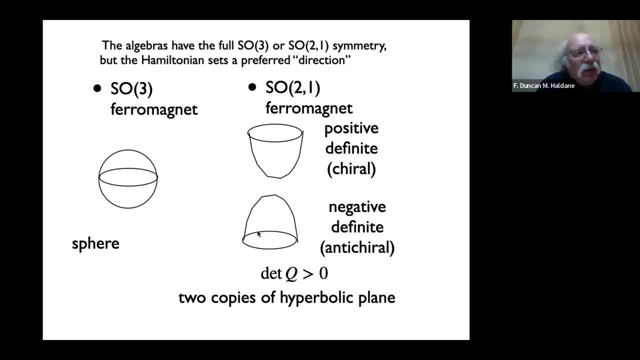 Once you include lander level mixing, you generate three body and full body type interactions between the guiding centers which break particle symmetry. So it could be that the experimental stuff about the five half state Having It has a thermal whole effect Equal to the filling factor, which is a signal, which is which would be compatible with particle symmetry but doesn't require it. 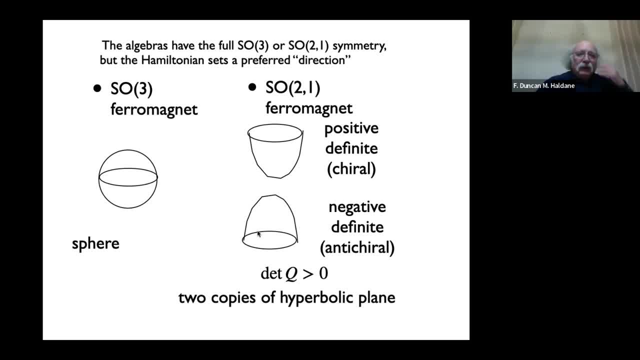 You know that could be resolved by this, by the fact it needs part of the whole mixing, particle interaction, particle mixing to get a level, mixing to get the thing. So anyway, we have an interesting dynamics of the order of the quadruple thing. it's kind of like a ferromagnet, but 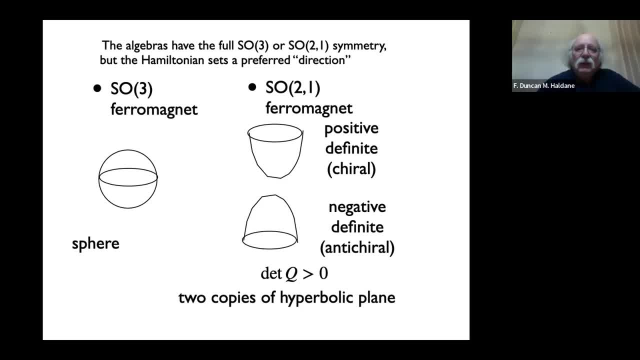 Slightly different. Slightly different because it's so two comma one, And what else is there in this thing? so there's a lot of kind of interesting things that seem to emerge from from from understanding that the corner whole fluids are quadruple fluids. 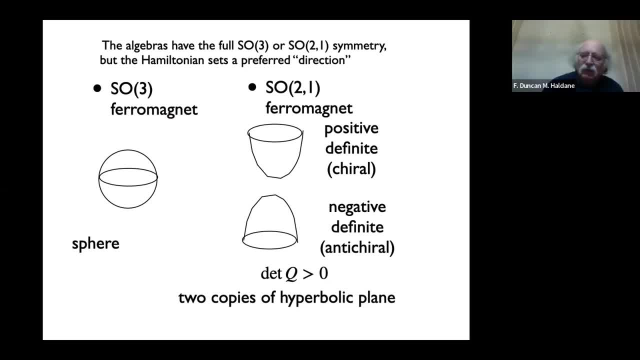 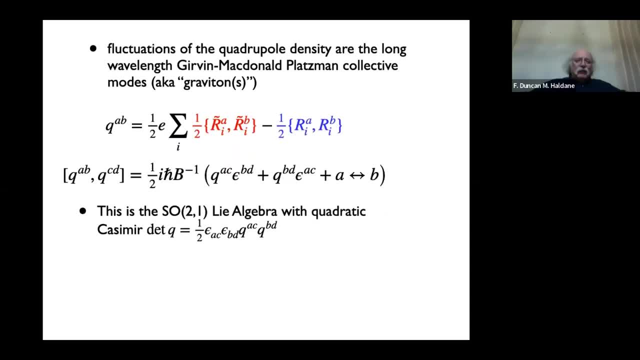 Another feature- funny to finish- I'm not sure if I've got a slide on it- Is that If you have a dipole, if you have a polarization, Then if the polarizer, If the polarizer, If the polarized state terminates right at the boundary. 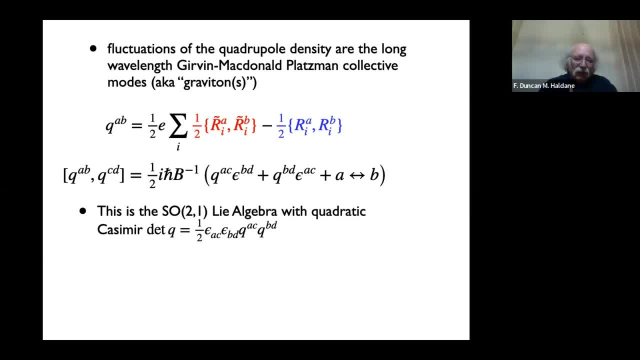 Then there's an electric charge on the boundary and bound charge which is proportional to the normal component of electric polarization at the boundary. that comes out of the standard boundary conditions one learns about in electromagnetism. If you have a quadruple density, that terminates. 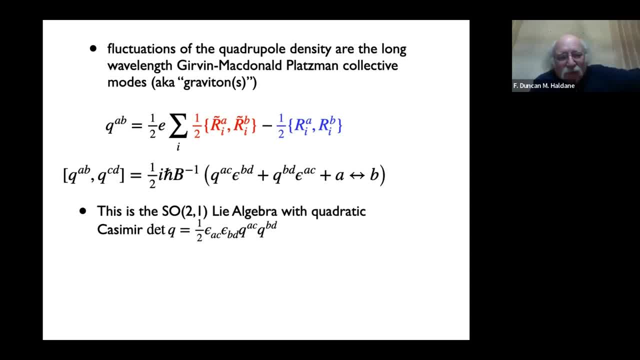 Abruptly, as it would do at the edge of the quantum Hall State. If the quantum whole liquid as a quadruple moment and and the portable density and there's no quadruple outside the quantum whole liquid, It's the same principle. shows. it shows you that you get a dipole moment on the boundary. 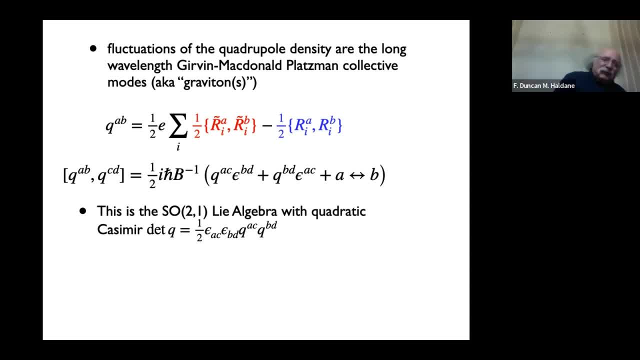 So, just like a discontinuity, the dipole moment gives you a charge on the boundary of discontinuity. in the quadruple density gives you a dipole moment on the boundary. and indeed when you look at the look at the edges of The fractional whole effect, you see dipoles on the boundary. 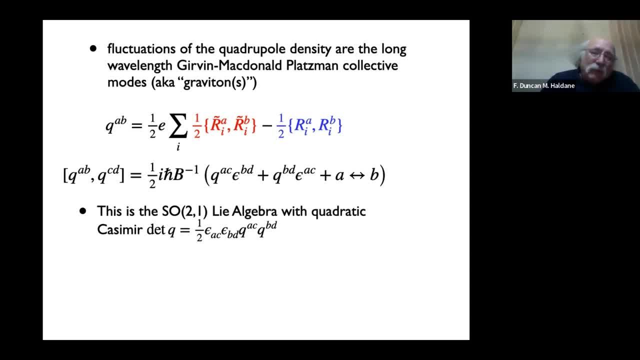 And they come from the quadruple moment in the integer whole effect. in the integer whole effect, the lipos just come from the form factor of the land or level set. When you the shape of the lamina orbit and it's distribution, The shape of the lambda orbit and it's distribution, 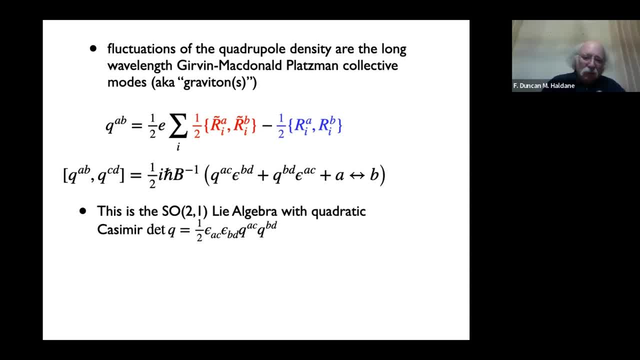 When you come to the boundary, when you come to the boundary, And so the quadruple, immediately, Immediately, as a, you immediately get a complete, complete description of the dipoles that are found on the edges of quantum Hall states, which wasn't really properly explained before. 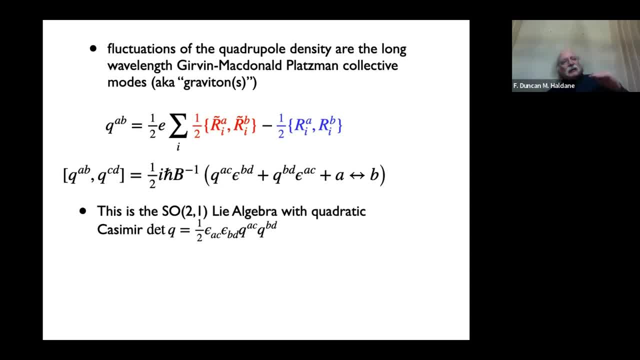 So it's a- I believe it's a very significant new characterization. Quantum Hall fluids are electric quadrupole fluids, as well as having all their interesting topological properties And the geometric properties and the energetic properties are contained within the quadrupole part. 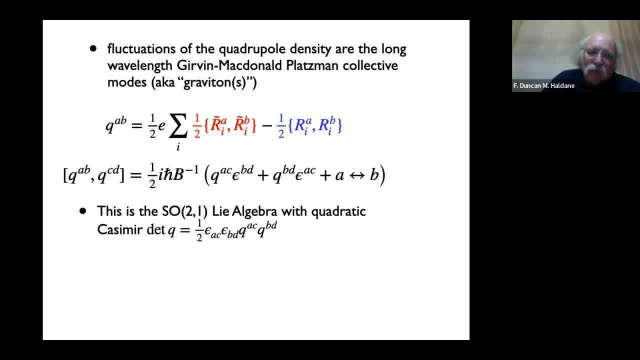 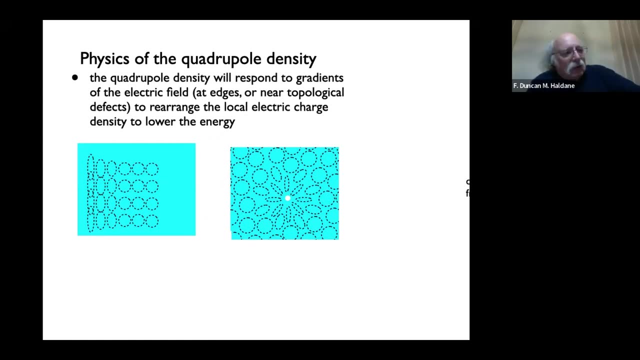 So there may be some hope in understanding the mechanisms and the energetics of these states by chasing this one. So I guess I've sort of run out of time. So there's a picture. I think it gives you a new, a new angle on looking at these things. 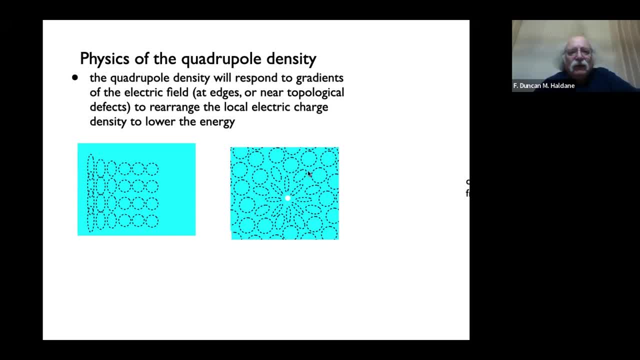 The quadrupole and the relation to the flow velocity is giving you a much more fluid dynamics kind of picture of quantum Hall states, Even though it's it's dissipation of fluid dynamics, right, Because the fluid dynamics is being controlled by the electromagnetic field, which completely fixes the flow velocities. 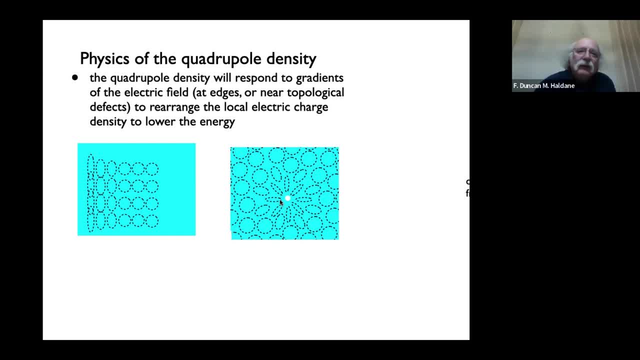 But otherwise it's. it somehow is giving one a new, a new line, a new line of things. So I think I should stop there, because we've gone 10 minutes over time already, But so we'll leave it at that, Thank you. 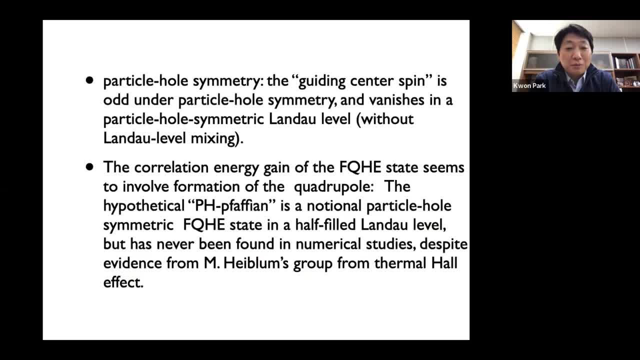 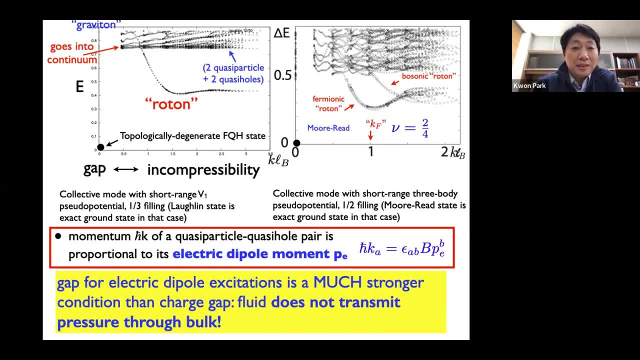 Let me leave you with a slide. OK, thank you. That's why, OK, thank you, OK, thank you. So are there any questions or comments? Let me so somewhat, Not direct question. Let me try to apply this framework to: I met up with you in three dimensions. 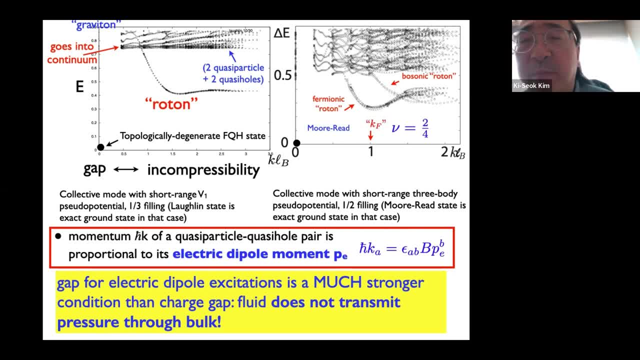 So I mean in the view, In the perspective of effective theory, if I drew some, some metric and if I intuit out 5. I will have some terms, I mean gravitational and electric, And so then I will have, I'm expecting I will have some on a level of some two energy in three plus one. 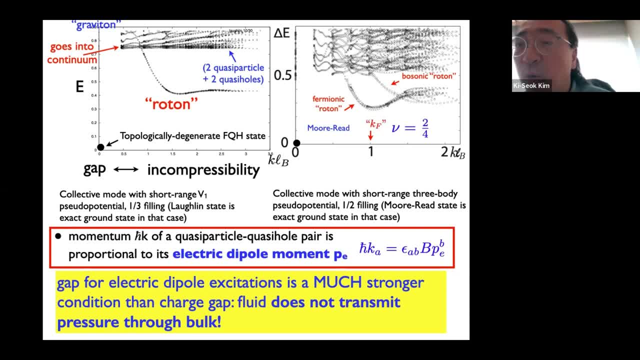 But so, but I want to understand some original. Can I have some helpful moment in bioformian system in three plus one dimension, like fractional quantum mode? you mentioned that it's the origin would be some column infraction minimization under strong magnetic field. so in 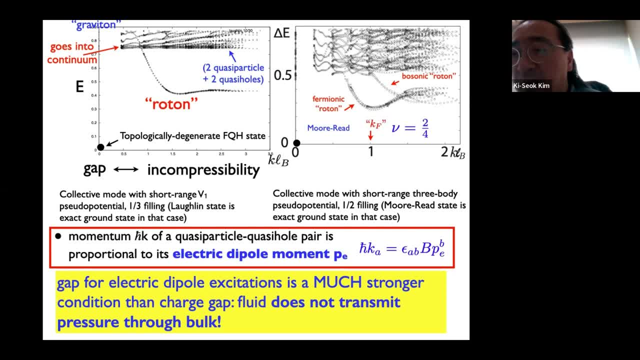 bioformian. can i some make some quadruple moment for fundamentally, yeah, in in paraformians. you said it would like a pile formula. sorry, high system, oh, piles, uh, yeah, i, i guess um a lot of these things in the involved gap, i mean most of the topological states involved. 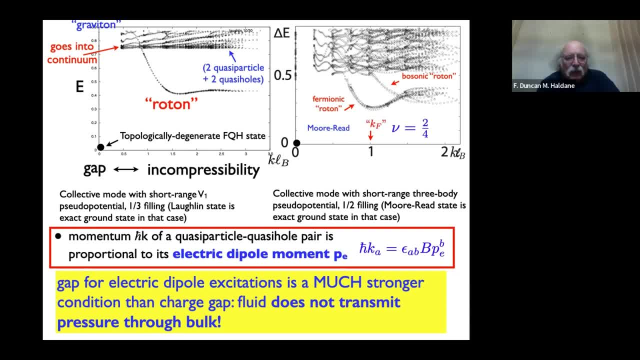 gaps. systems, okay, which are. they may be gapless on edges, but bulk gaps which protect, uh, which? so the protective thing, to apology, is the bulk gaps, uh, i, i mean with wild fermions. um, one learns a lot of things from wild fermions. for example, if you want a 3d quantum hall effect, right, yeah, the whole effect is defined in latin in planes. 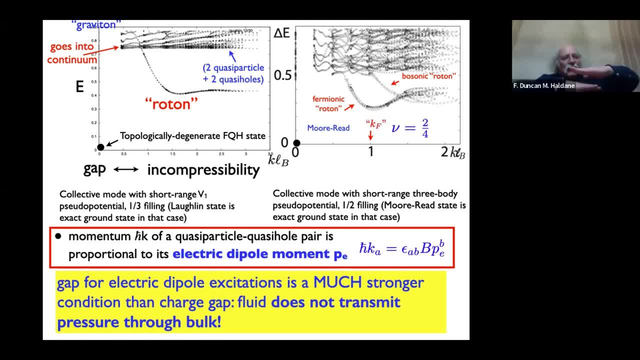 right, lattice planes. so a 3d hall effect is really a 3d stack of lattice planes. each of one is exhibiting a quantum whole effect, right, and one actually can see how does. and so and uh, as our has known that if you have a stack of these, um, these, these planes, then the edge sheet, this, the 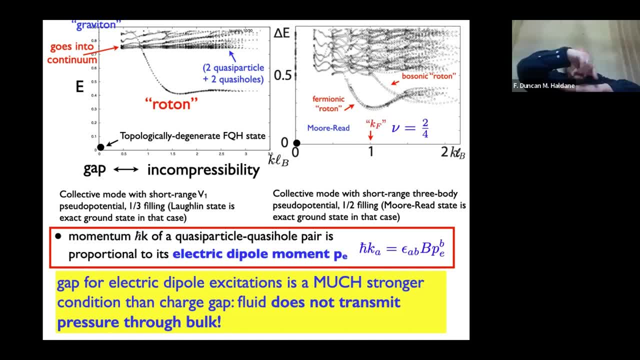 each of the planes has the has a chiral edge mode, so there's a whole sheath of chiral edge mode modes on the sides of the cylindrical arrangement, and the interesting thing there, which relates to wild fermions, is that then you could ask the question: how do you actually um? 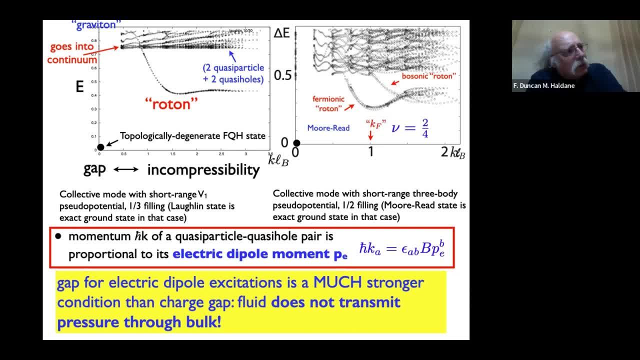 uh, how do you, how do you generate, how do you get a, how does, how would, how would you form a 3d quantum whole state? it turns out that if i have a wild fermion system, right, if i nucleate a pair of wild fermions and and separate them. 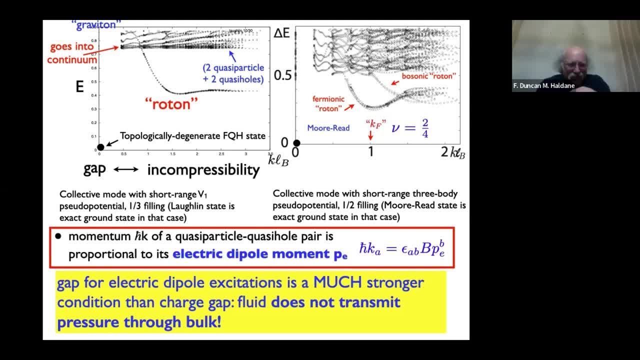 uh, you get this, uh, fermi arc, if you look, if you now take a look at the look at the system, if you, if you look at, look at your 3d system, uh, any, any time you see, if you look at it, you might be seeing in one direction. you'll see the one wild. 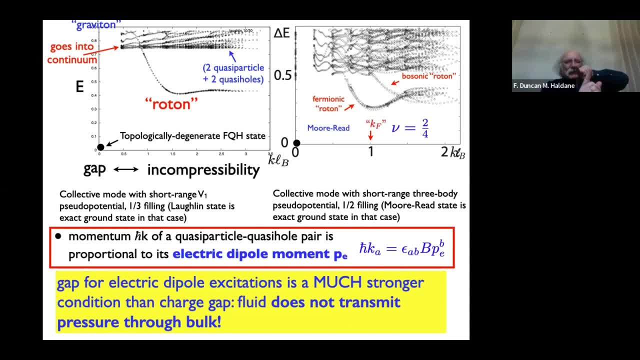 point in front of the other wild point and that and a surface which is perpendicular to that direction won't have any interesting properties. but if i look at it on a surface where, from an angle where i can see the two wild points separated right, then when they give rise to a projection on 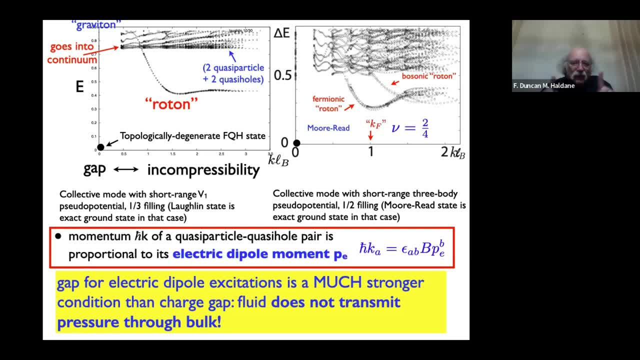 the surface, which is this, while the the fermi arc which vishwanath pointed out, right. yeah, so on the edge, on any edge, where if you look through vertically you see two wild points, two wild, two wild fermi points or little, you'll have a fermi arc. 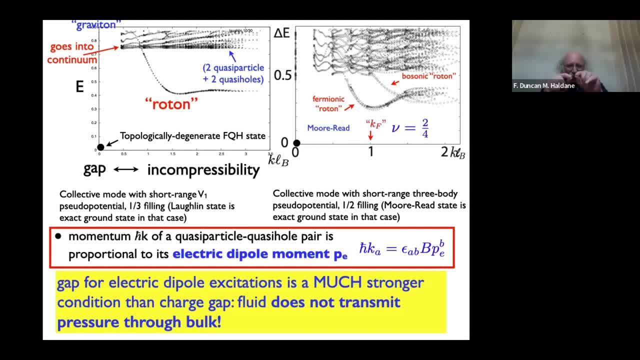 joining those two things and as you pull the two wild points apart the length of the fermi arc gets bigger. but when the two pile wild points get to opposite sides of the bruin zone they can annihilate with each other and they will leave the fermi arc over the 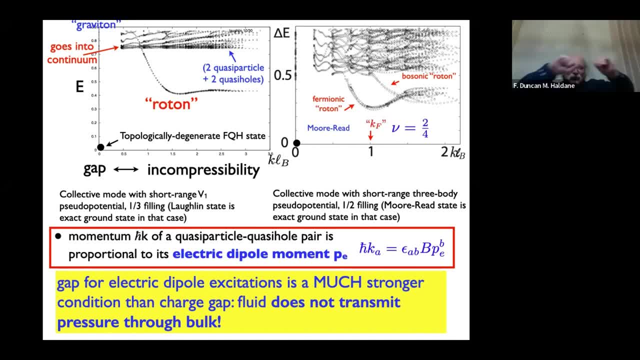 over that face of the crystal, on the on the facet of the crystal, that fermi arc will continue from one side of the blue end zone to the other side of the blue end zone and indeed that's just the chiral edge state you get of a 3d quantum Hall system. so the wild Fermi points allow you to 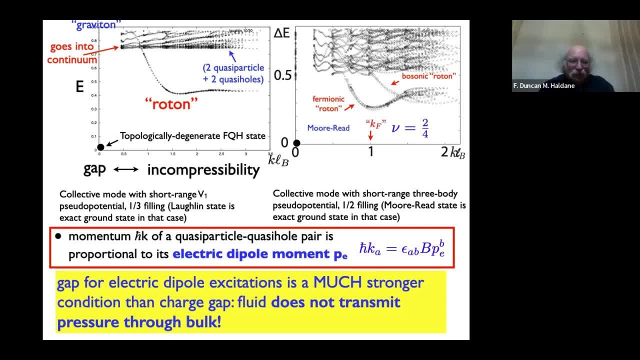 interpolate between a non-3D whole system, a regular, a regular hand insulator, and a three-dimensional quantum Hall system, which is a stack of a stack of planes individually exhibiting quantum Hall effects. so of course, the um, a family of planes, is labeled by a reciprocal vector normal to them, right and uh, that's entering in the formula for the whole of. 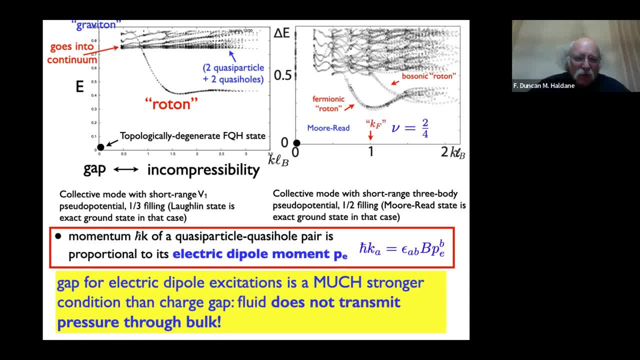 the 3D Hall conductance has to have dimensions of ohms to the minus one times meters to the. So it's e squared over h times a reciprocal vector, basically e squared over h being ohms to the minus one. So the lattice planes are indexed by a primitive reciprocal vector. 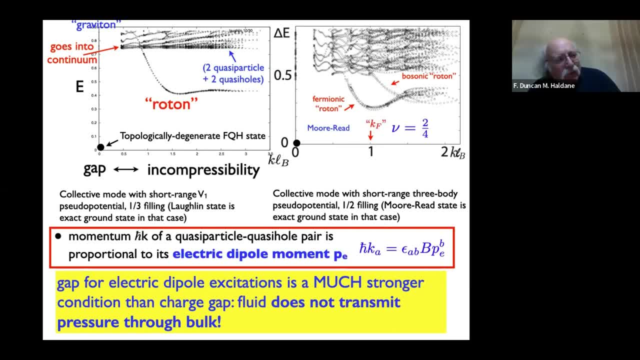 So the rational or integer Hall quantization is the number multiplying that reciprocal vector, right? So there's a reciprocal vector which is a stacking of the whole planes, forming a 3D kind of stack, And the number multiplying that is a rational or an integer which gives you either a fractional 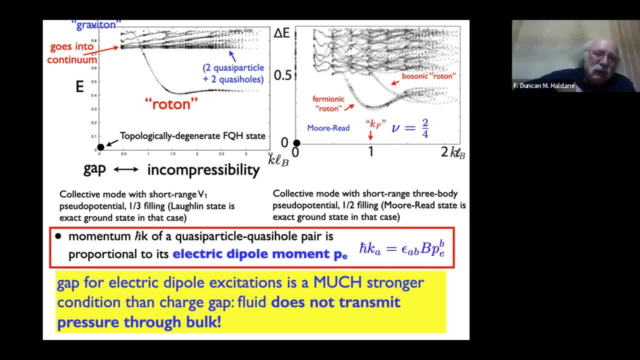 or an integer Hall effect in the individual. So but to go between, at least for the integer case, to go between a band insulator and a gapped band insulator and a gapped Hall insulator, quantum Hall insulator, which is a stack of 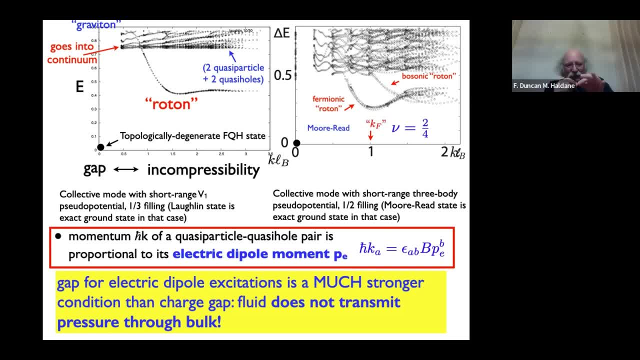 planes involves an intermediate, gappers phase, which where you've got where the bulk has these Dirac points or wild points, And they annihilate and they leave. they leave an edge state, a Fermi arc on the edge. 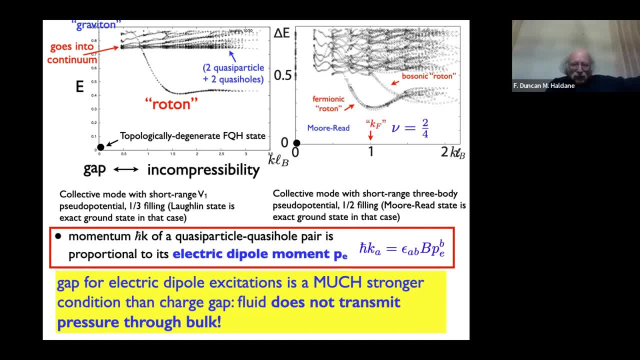 and they annihilate again and the bulk becomes gapped again when the two wild points have annihilated. So you're not in a, you're in a more critical regime when you have like wild points. So it's not so. but yeah, there's certainly a lot of interesting things to be sorted out. 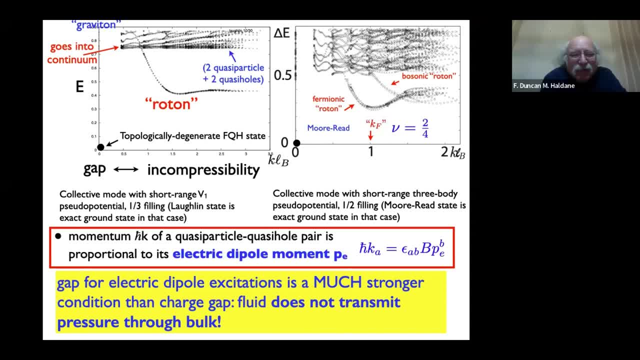 in topological states which are not gapped right- I mean it's still even in the quantum Hall problem- To actually fully understand the, the composite Fermi liquid, which is a which has this particle Hall symmetric character. There are these interesting ideas that that that Damson has put out, but they're not very. 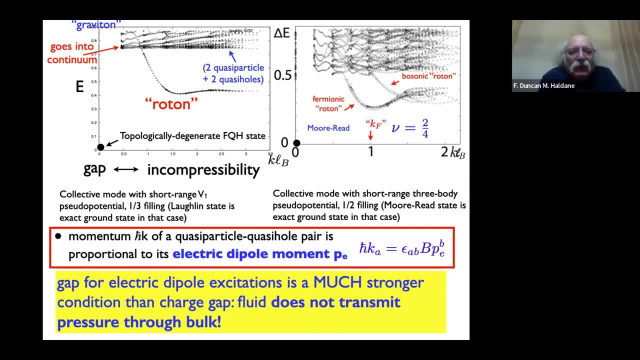 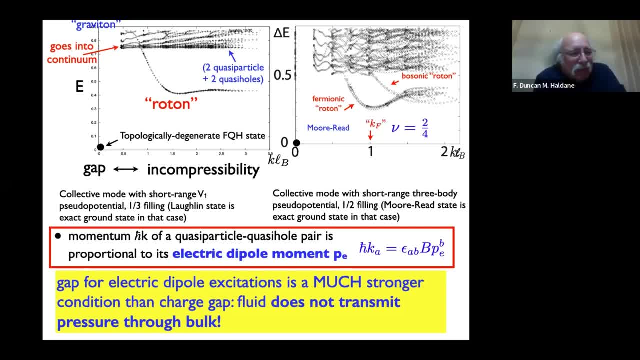 the yourself, and much of what we fantastic wrote earlier about, I think, took place in World Minority temperatures. So it's it's all quite interesting. It's niceINKR. uhhh, hi, I'm comes, or Anthony E, without, without, just put it what you chose, Mirta. 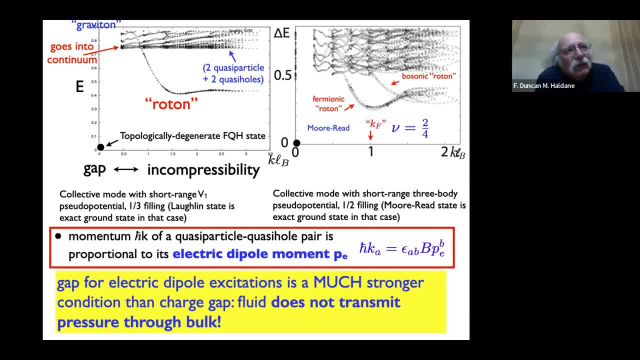 Yeah, it was very nice to put it. I want to say thank you as well. It is very interesting, Great thing. Thank you so much. Thank you for the talk. Really It was cool. It's a pleasure, Thank you. 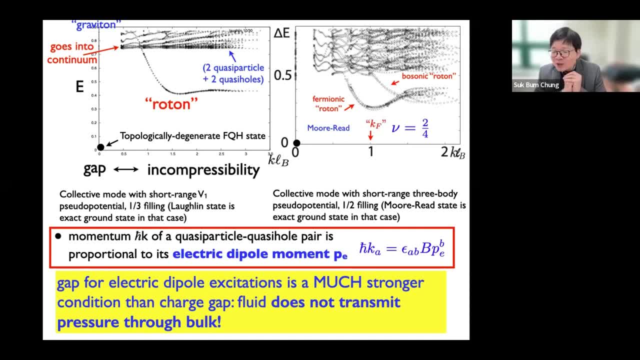 So now I'm short of time, So over to Oh, a, a, a big one. So and Okay, And I mean you're relating this to both, to I mean your two points you were making- is that their fluctuation would lead. 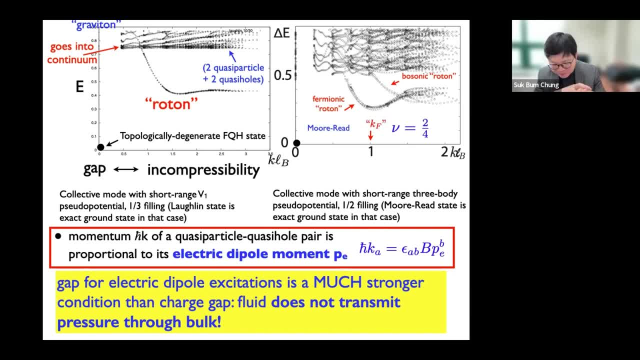 to this Gerben-Platzmann. Yeah, so Gerben-Platzmann Also. they give rise to the whole viscosity. So I'm just wondering: are we supposed to think that this whole viscosity should be an important parameter in deriving the Gerben-Platzmann McDonald's moves? 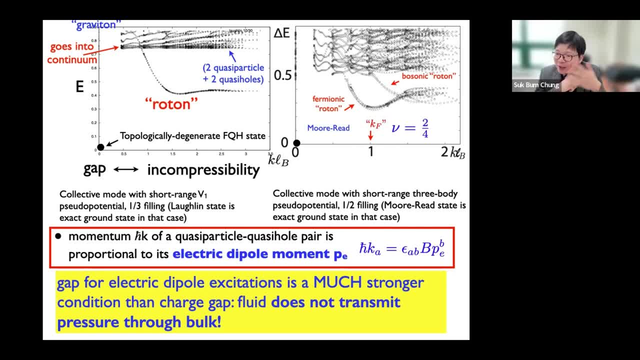 Well, the? I mean, should there be some natural way to relate these two? I'm saying that the system is actually like a. If I can, let's find this slide again. Okay, I mean, can you formulate this, Gerben-Platzmann? 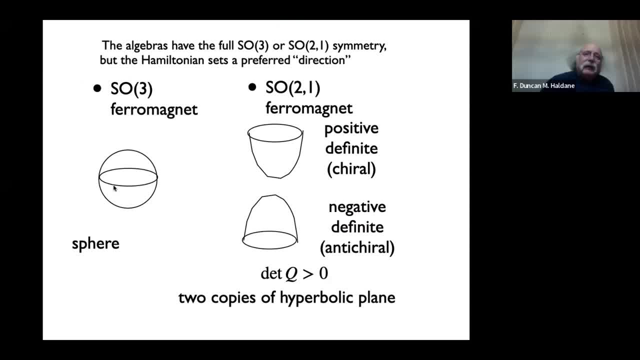 McDonald's move. Yeah, yeah, yeah, It's precisely this. I mean, I guess it was an earlier attempt, by which I think is not which I disagree with- which- Sundy and Kibbleson and my student, the AJ Park, they got my student. 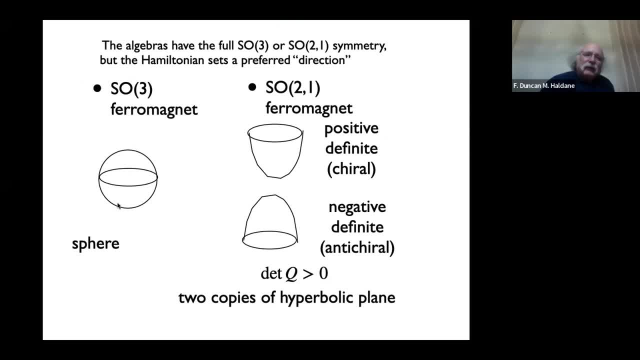 the AJ Park and they got my student the AJ Park and they got my student the AJ Park to work on it, But they wanted to have a nematic transition. But actually this is the Here's the issue- that 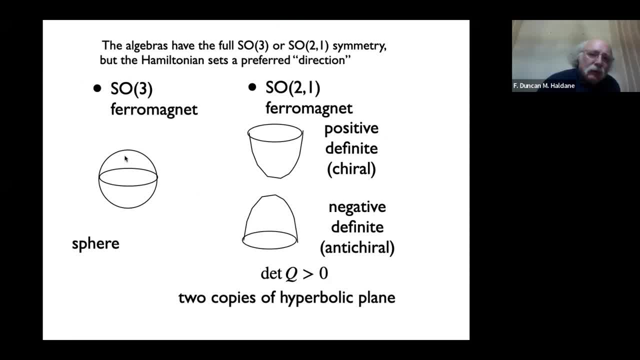 the algebra of the commutation relations of the quadruple field are precisely SO2,1.. Okay, So if I have a ferromagnet, of course a ferromagnet. if it's Heisenberg ferromagnet, it can point in all directions, right. 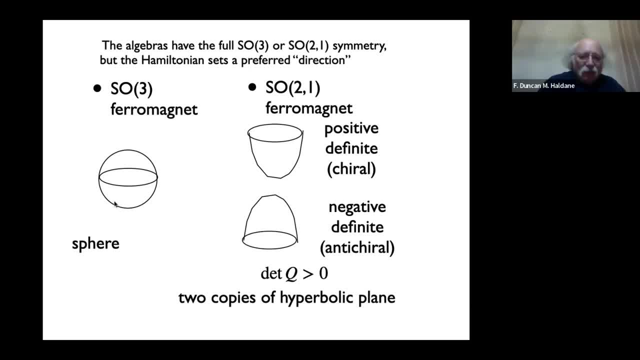 There's no choice, It's: all directions are equally good. So the analogy is not so much, but it's gapless. then right, The analogy is not the Heisenberg ferromagnet, but the Heisenberg ferromagnet with a Zeeman coupling to it, right? 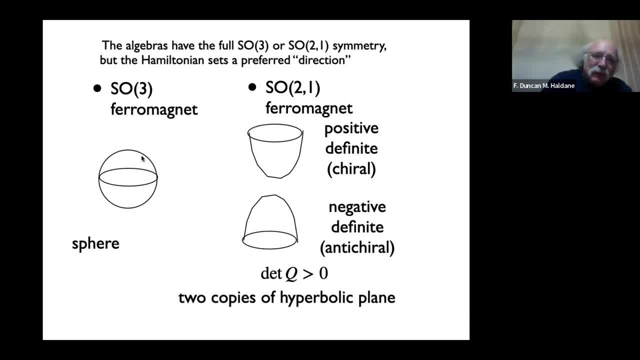 So the Zeeman coupling fixes a particular point, a particular direction on the sphere where, if the ferromagnet or the parameter points along that direction, it minimizes its energy. So the Zeeman term singles out a preferred direction for the ferromagnetic order parameter. 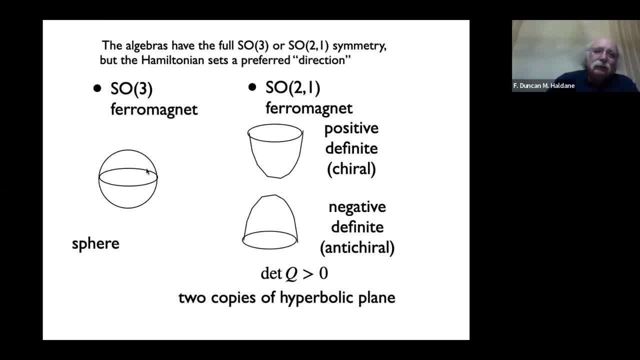 to what to point in, right, But all points, without that preferred direction, all points are equivalent. These hyperboloids they're also, every point on them is equivalent because they're like a mapping to the Poincare disk or the hyperboloids. 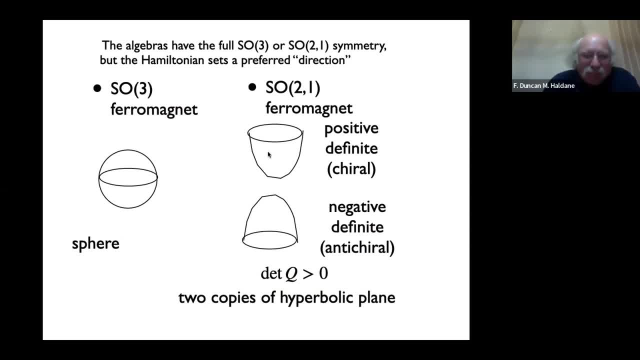 They're like a mapping to the hyperbolic plane and all points in the hyperbolic plane are also equivalent to each other. So if this is a quadrupole tensor with two asymmetric tensor with two upper indices, we can rescale it to look like a metric. 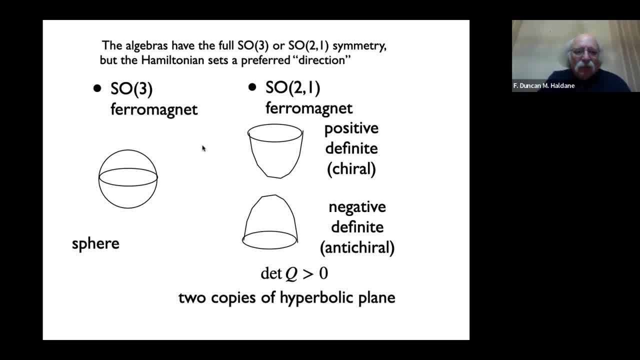 It's not a metric because it's not used for a coordinate system. I was confused a long time about this issue. In fact, what I believe now is- I mean this: there's some stuff on this slide which is, I actually believe, that the Wen-Z term. 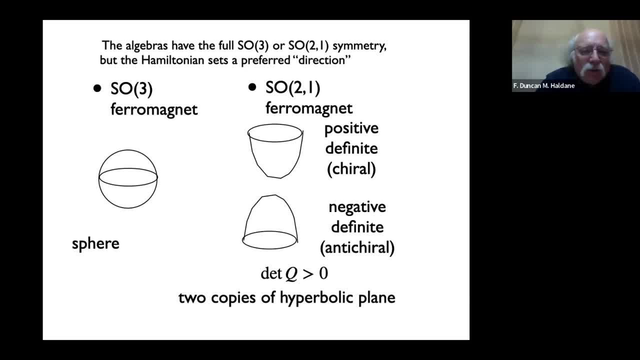 is fundamentally inappropriate and not part of the quantum Hall story. The Wen-Z term is very specific to the toy model with rotational invariance And so the you can look at. I have a preprint out but you can look at it if you actually 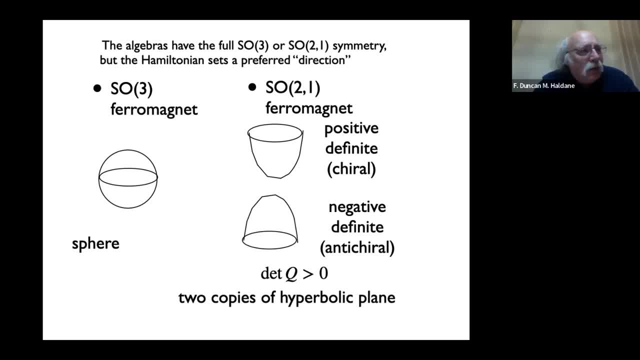 so initially I was very impressed by the remark that you know, you put things on a curved surface, the quantum Hall on a sphere, and you have this extra part of the electron density which is proportional to the Gaussian curvature. right, This was this kind of 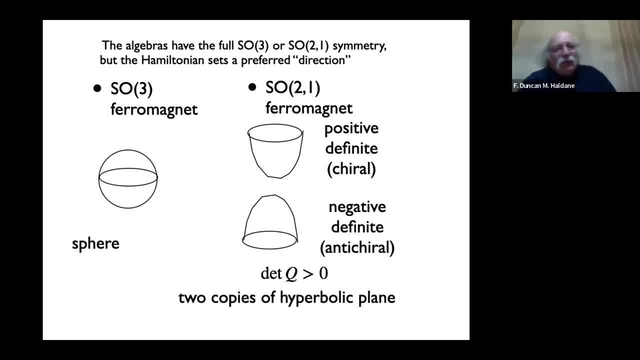 so, and then that suggested this idea that whole viscosity was, and then the amount of excess charge was related to the shift and the whole viscosity. So it gave this idea, which I think is actually a fundamentally incorrect idea, And that's pretty. 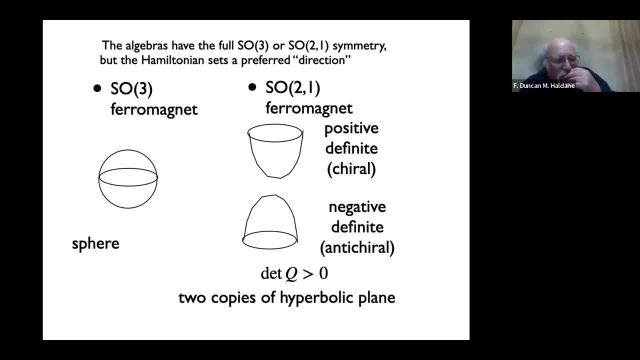 most people, theorists, people in this field, have come up with this idea from the original paper of Avron that says that the whole viscosity is somehow a response to background curvature and metrics. But actually there's no Gaussian curvature of any kind. no Gaussian curvature. 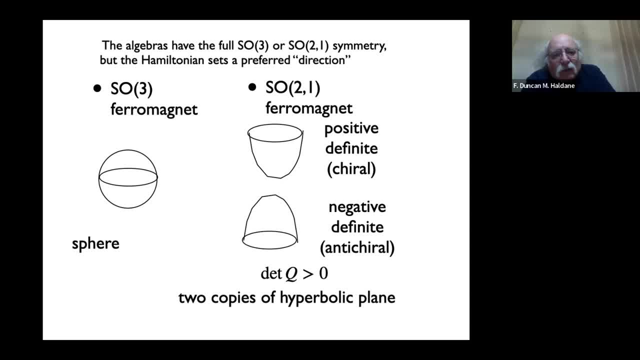 not at point. singularities doesn't occur in the quantum Hall effect. The quantum Hall effect is on flat lattice planes which are macroscopically flat. You can see that if you look at any ring right, The crystal is flat, And even graphene sheets. 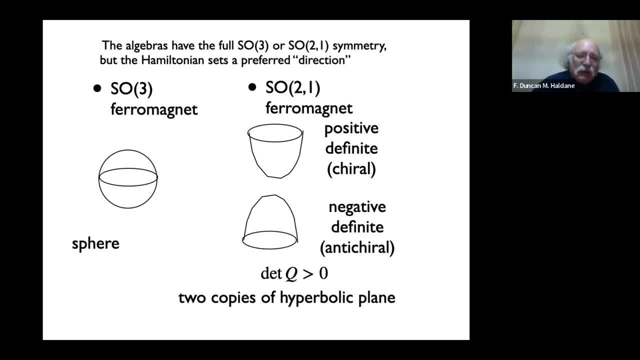 graphene sheets are like graphene sheets are like a piece of paper. They don't tolerate Gaussian curvature at all. They love, they can have. let's try this, They can. they can of course, be bent this way, right, But once you bend, 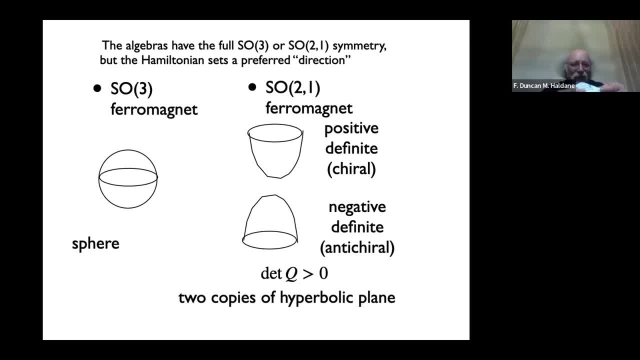 once you put extrinsic curvature on it, you can't, you can't, you can't bend them, You can't make them have curvature in the second direction. And in fact, the only way to get the Gaussian curvature in a graphene sheet, 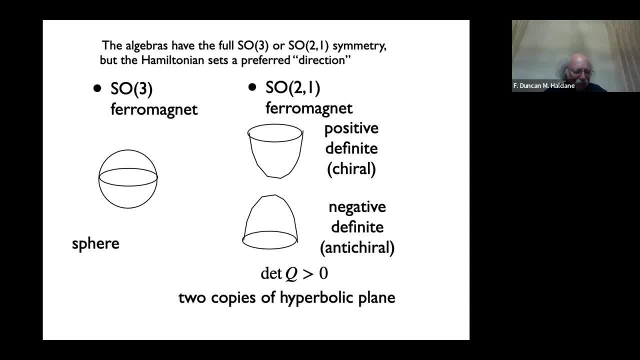 if it's not apart from having kind of disconnections and things. right If you, if you want to, yeah, if you do this, basically right. So of course, if you fold your piece of paper, of course you get a cone singularity at that point. 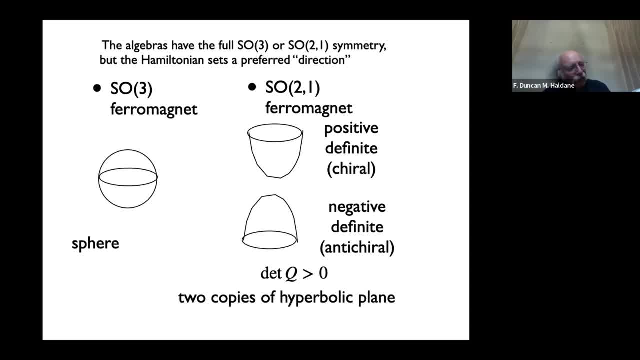 but the paper doesn't. there is some. if you force this to to wrap something, you force it to have Gaussian curvature. The Gaussian curvature is completely localized at cone singularities which are at the intersections of the folds you make. So I don't. 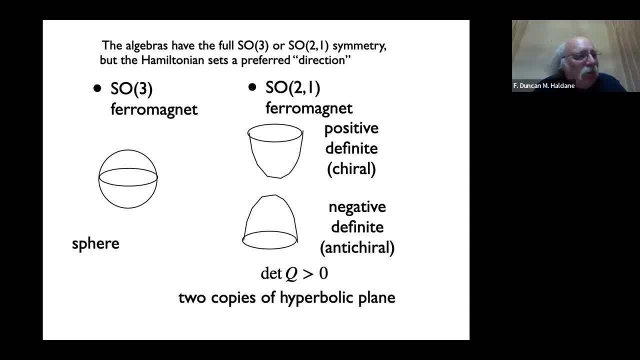 I believe the idea, while it's beautiful with conformal field theory and things, it's a property of the bulk conformal field theory, as in the Laughlin wave function. because it it is, it's matching this criticality on the edge. 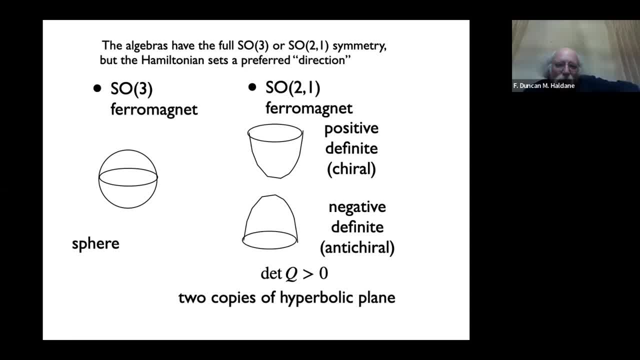 but the toy models extend it to the bulk. but there's no true conformal field theory in the quantum Hall effect bulk theory. It's a toy model aspect. And so, once you remove the rotational degree of freedom, which is clearly unphysical, 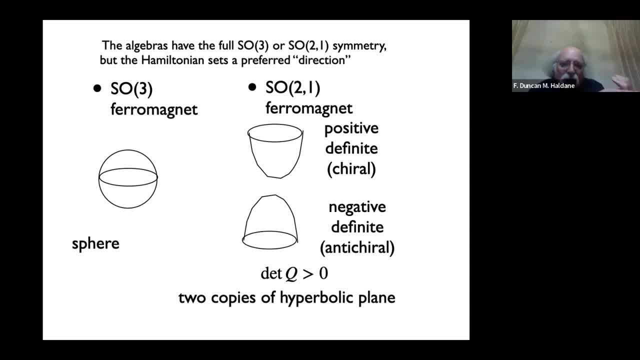 because it it there was. no, there's no rotational symmetry. in condensed matter, You actually start to find this thing. So the when Z term which is responsible, supposedly responsible, for this additional charge on the surface of the sphere, the? 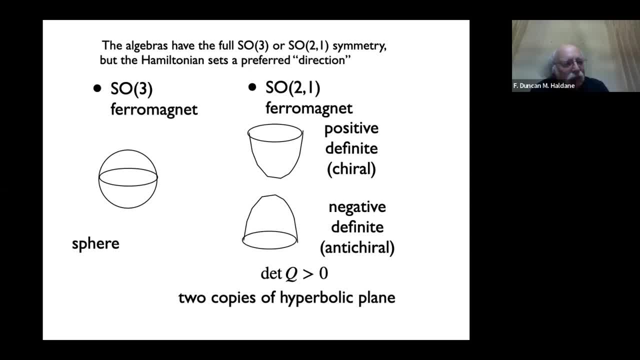 the X, the excess charge is actually just the, the double divergence of the of the quadrupole density. So if you actually adapt the isotropic formulas to the sphere, you actually find you can recover that formula- previous formulas- from Gaussian curvature as a special case. 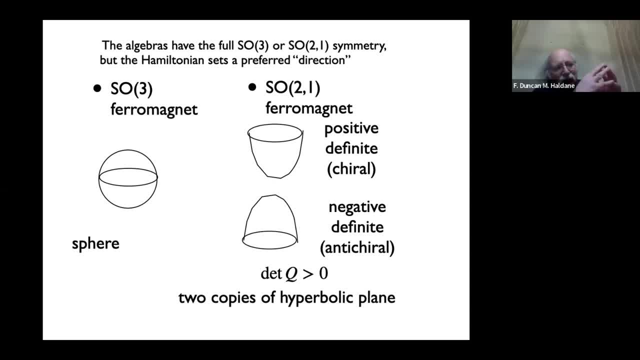 So of the you, if you identify the metric on the sphere with the quadrupole, now it has to be spatially varying because it's on a curved surface. The second derivative, the second divergence of the inverse metric gives you the Gaussian curvature. 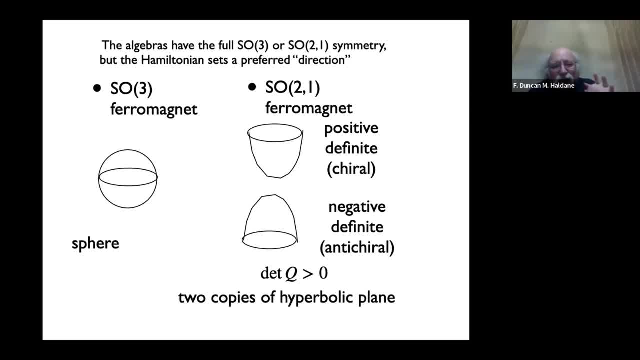 But that's exactly the same formula as the second day, as a second divergence, double divergence of the quadrupole thing which gives you the bound charge. So the. so the general formula which removes rotational symmetry from the from the model, actually removes the. 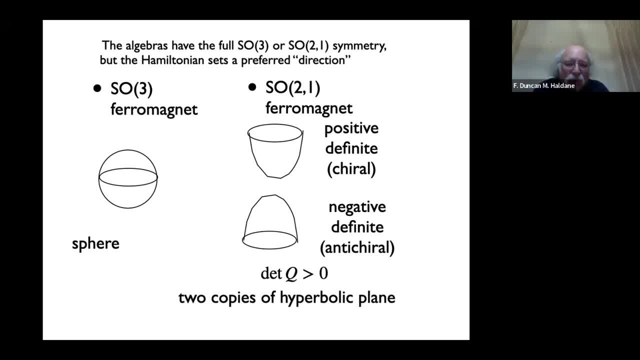 when Z term- So the Wednesday term- is only compatible with rotational symmetry. And there was a whole lot of stuff. There was a whole lot of stuff about the, the gravitational Chern-Simons term. I know people there know about it right. 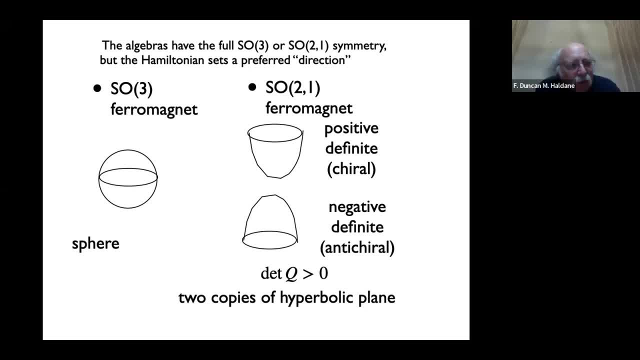 Or relate, in its relation to the, to the thermal Hall effect on the boundary, And I guess sometimes you know, some years ago Mike Stone finally showed that the the thermal Hall effect was, was like totally on the boundary Right. 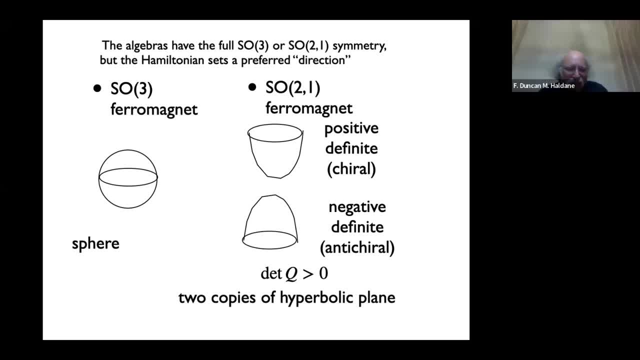 But if you have the Wednesday term in here, and and and in a row, relativistic field theory of a gravitational Chern-Simons term, which, but I think all that needs to be generalized to get rid of the rotational symmetry. but the Wednesday term gives rise to additional terms. 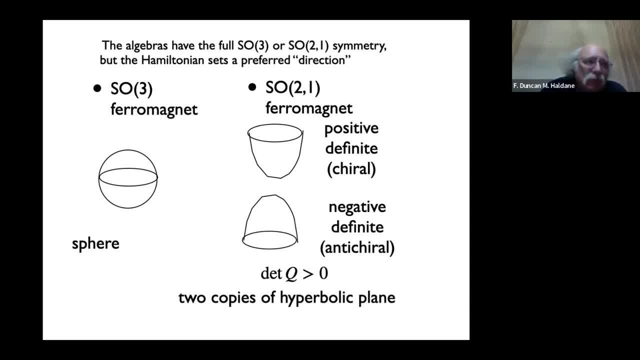 It's the spin connection. But once you realize that the, the, the, so two comma one, the, the quadrupole field is not a metric field, It's not used to measure things. The coordinate system is: the flat is the coordinate. 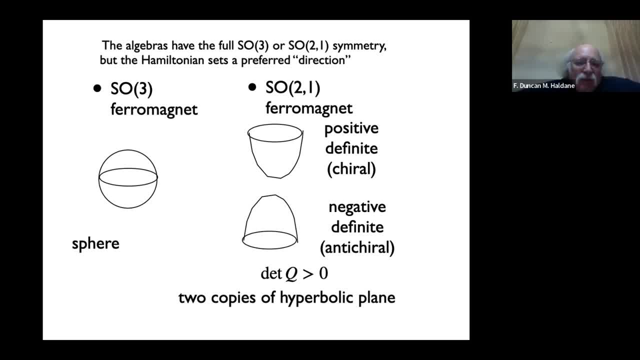 The coordinate system is the flat Cartesian coordinate system, The. the crystal plane inherits from the lab, inherits from this flat background. There's no integration over over fluctuating geometries. There's none of this, Yeah, Spin connection in it. So one of the things